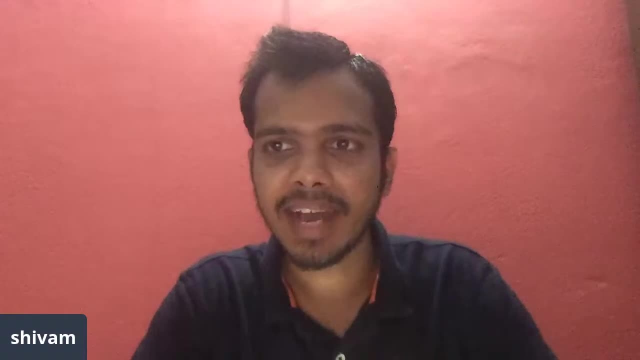 Yeah, Himals is there, as always. Yeah, hello Himals. How are you And how is your job going on? Yeah, I see that there are four people Live now. Yeah, hi, Harshith, Good to see you back again. So I didn't see you in the previous session. 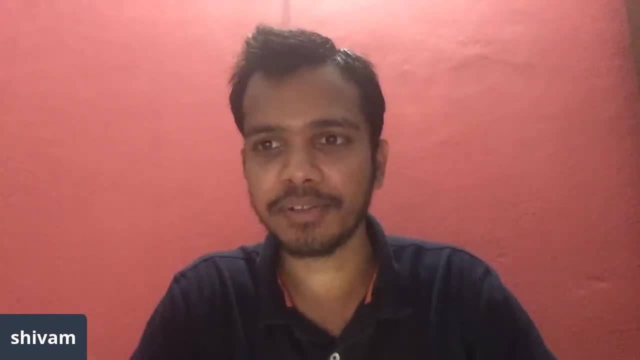 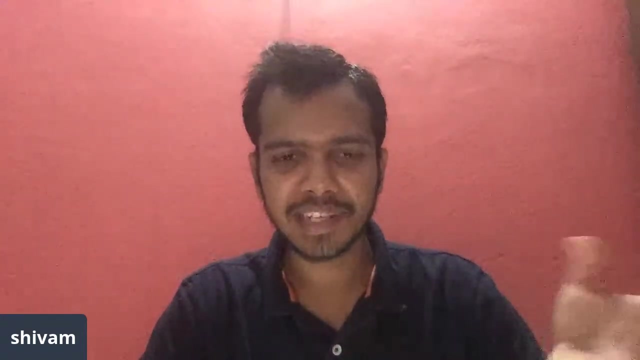 And, yeah, how are you doing, Adam, How is your work and how you're doing? Yeah, hi, Karthik, Yeah, Yeah, regardless. Pardon me, I am also good, Like I will be like working from home, mostly till till December, Mostly I will be working from my home itself. 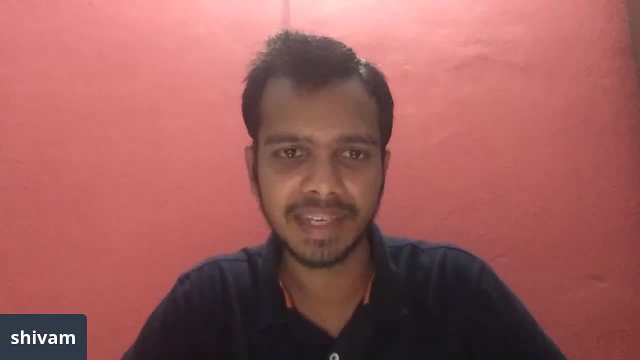 Because you see, a number of cases are increasing day by day And I'm not sure when the office is going to open again. And what about others Like? what about you? I mean when your office are going to open, Like? is there any communication on that? 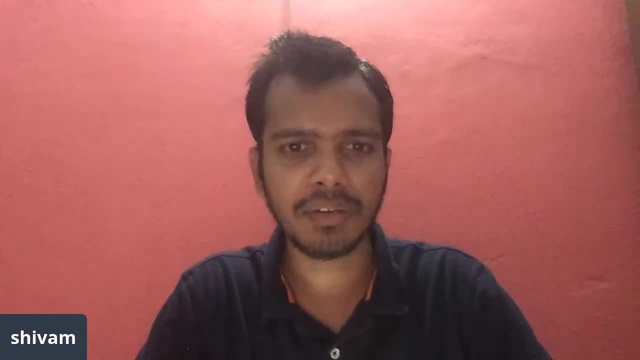 Yeah, I see around seven people have joined till now, So I'll wait for around one, two more minutes and we'll start the session. And this session is a very important one because I think process management and memory management are the two important parts of the operating system. So if you understand these two well and most of the operating system, then you will be able to understand. 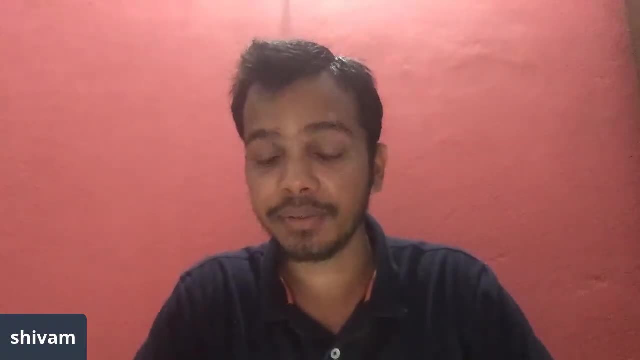 Yeah, okay, Harshith was not well, okay, Yeah, do take care of yourself during this time. Yeah, I saw your comment on my video on the process. Yeah, thank you for watching that And also giving a providing me the feedback on that. 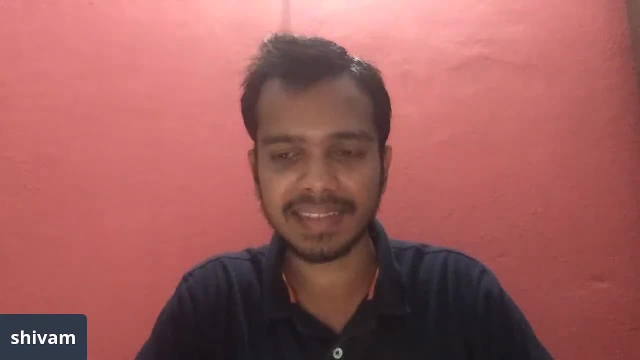 Yeah and Skarthik, I am certainly not this year. I'm also thinking like this year it's not going and offices are not going to open again, at least in the IT sector, And mostly I think it will be. Yeah, either number December or mostly next year, or the number of cases decreases. 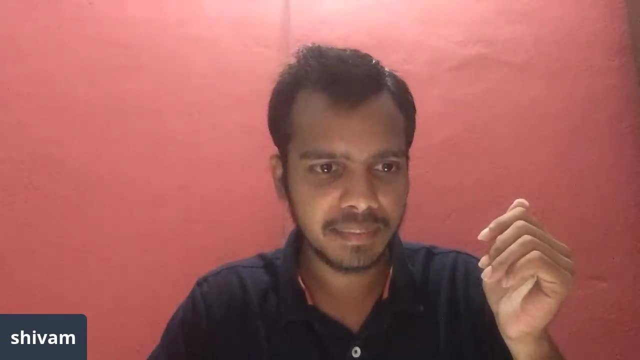 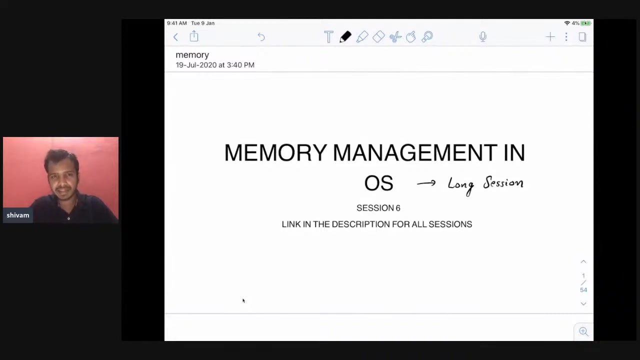 Okay, so let me- I think I think seven people are there- to let me just share my screen and start the session and I can take the questions in between from everyone. You know this session may be a bit long, So okay, just also comment: I mean, if you're able to see the memory management in OS and in this slide, if you are able to see, just do a confirmation in the chat box that you are able to see this. 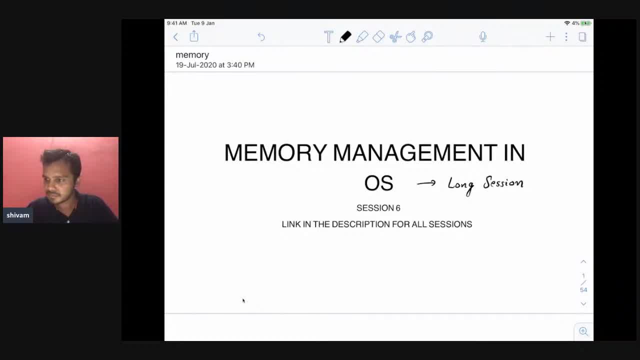 You can also do a comment preventionoks are sharing, and same one from Mr. Yeah, I think you will be able to see it. Yeah, so let me. I have not seen comments or anyone, so, okay, yes, She does say that and he is able to see, so I think all of you will be able to see my screen now. 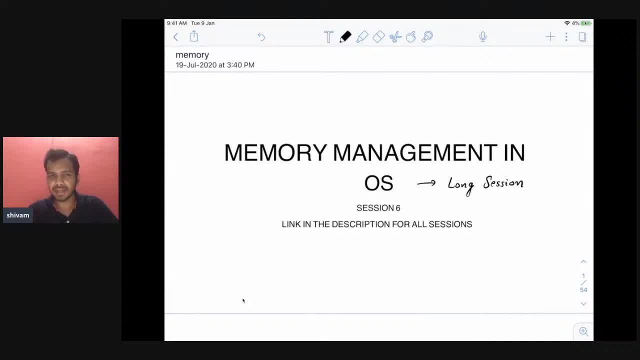 So in this, so this, this is mostly kind of second last session of Burke orbiting system. I'm training that I will take in the next session and the opt-in system course will be completed kind of. and in this section I will cover the memory management in OS like, which is very. 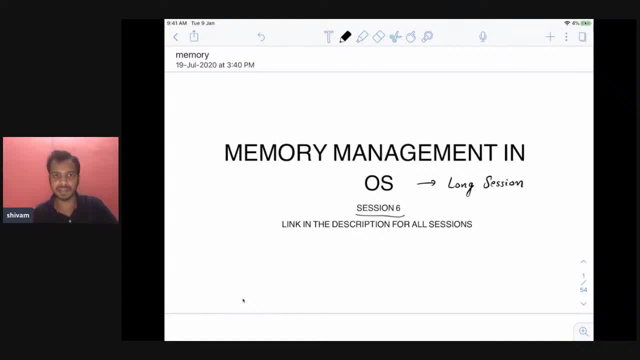 important and this is session six, so I have taken five sessions before this and if you have not watched those, of course the recordings are there and you can find the links in the description of those. all the videos and also this may be a bit long session because I will. 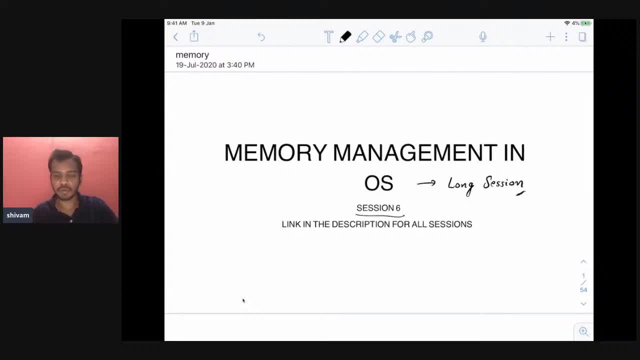 be covering the- I mean full memory management. that is normally. if you go to galvin book, there are two chapters for it. so I'll be covering in one session all of that. so it may take some long time and longer time, more than one hour maybe. so be there and you will. 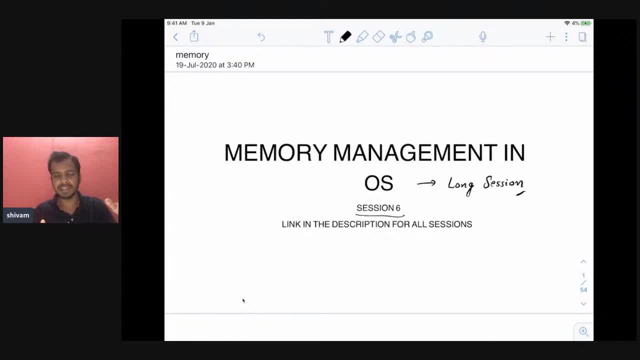 understand the whole concept better. yeah, I do not want to like break down this into two parts, because both the parts are connected. I mean virtual memory as well as paging. everything is connected to each other, so I didn't want to like break down that into two parts. so 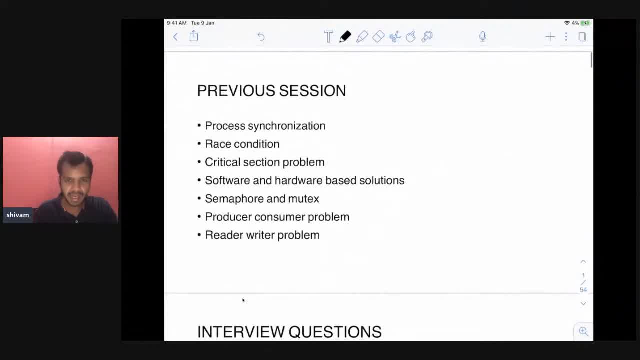 that's why I am taking that in one go itself. and also, if you have not subscribed to my channel, do subscribe to my channel and also like my video and let it go away- it will not wait video so that it motivates me more in. I mean sharing more type of this type of content. 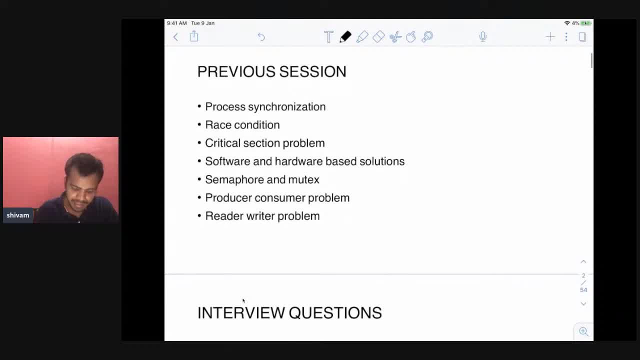 in future also. So in the previous session, if you see, I mean I covered like process synchronization part. what is race condition? what is critical section problem? what are the software and hardware based solution for critical section problem? What is the difference between Sema 4 and Mutex? 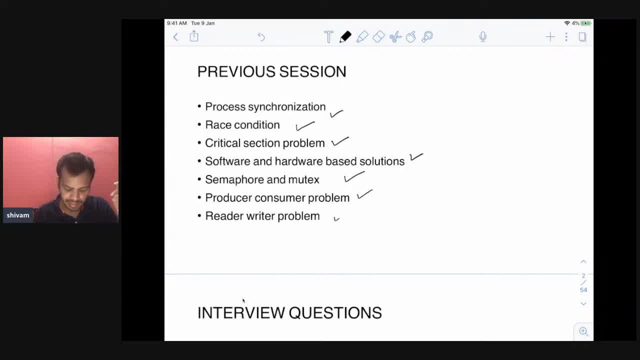 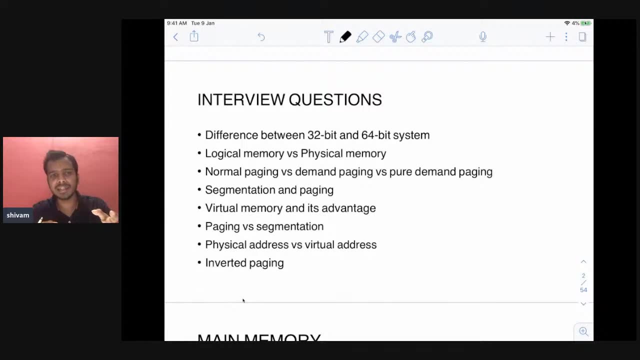 And I also gave the example here. then I discussed the applications of Sema 4 and Mutex in producer consumer problem and data writer problem. This all I covered in the last session. Now let's move on to like before every session. I cover that. what interview questions you? 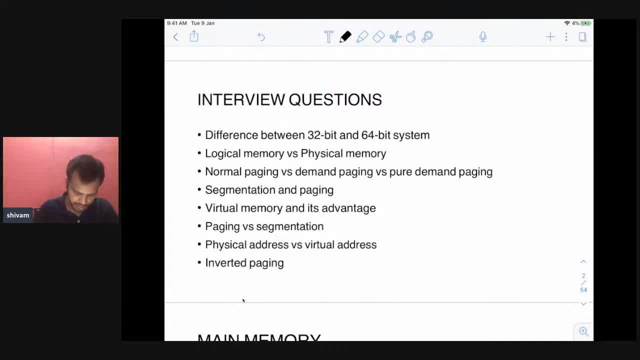 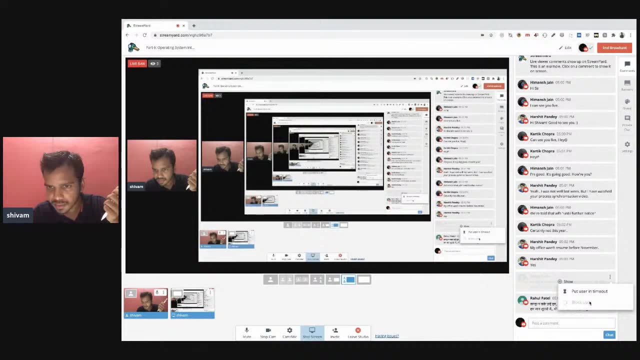 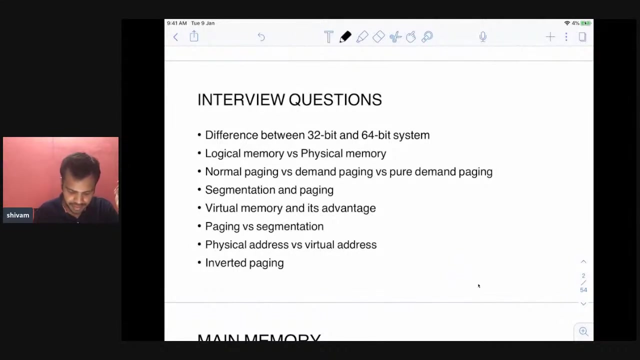 will be able to answer after watching this session. So some of the- if you see some of the interview questions here, let me one minute. let me block this user, Okay Okay. So the interview questions here are like difference between 32 bits system and 64 bit system. 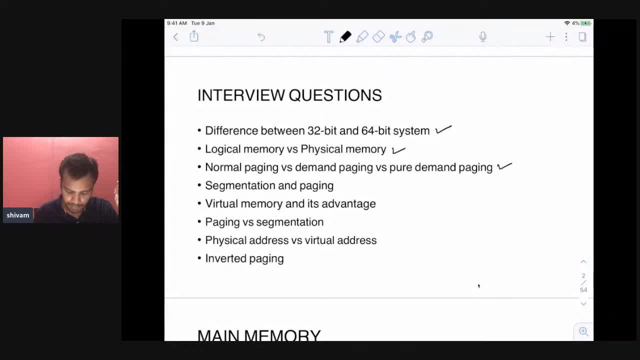 What is the difference between logical memory versus physical memory? What is normal paging, demand paging versus pure demand paging, the difference between all of this? And what is segmentation? difference between segmentation and paging? Then, what is virtual memory and its advantage, paging versus segmentation? physical address. 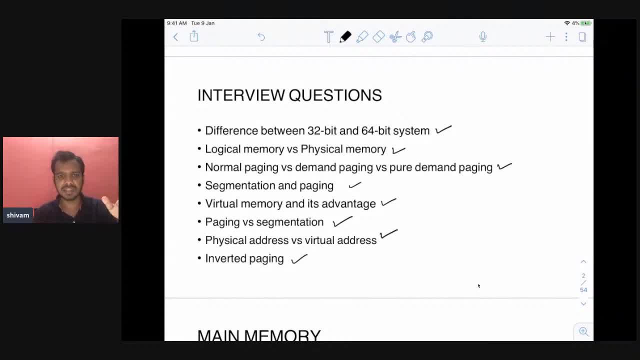 versus virtual address: inverted paging. Okay, So there are multiple questions that can be asked for memory management, because it is a very diverse topic. But I have included some of the questions here And as you go through the session you will be asking more questions, surely? 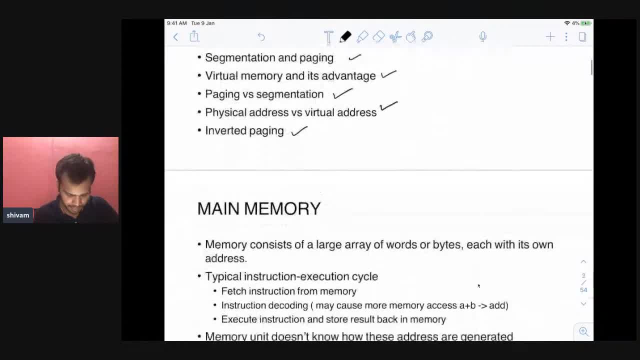 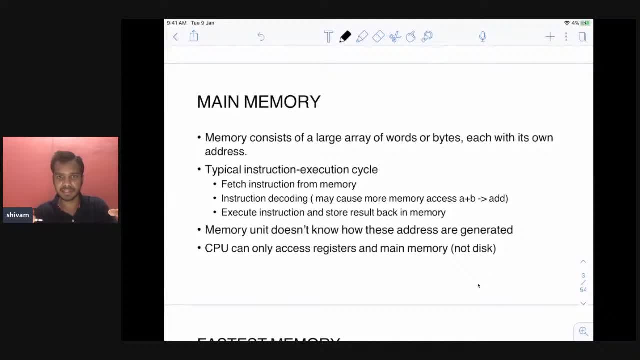 And you will see that there are more questions than this. So let's start with see, we are going to focus on main memory. So we are not going to mostly focus on the file system or a disk memory. We are going to focus on the RAM, main memory here. 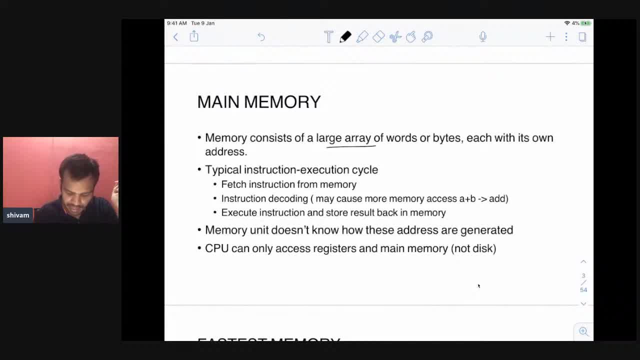 So if you see the main memory, main memory consists of large array of words or bytes, each with within its own address. Okay, So if you see the RAM, it's kind of an array of bytes. right, This is like an array of bytes. 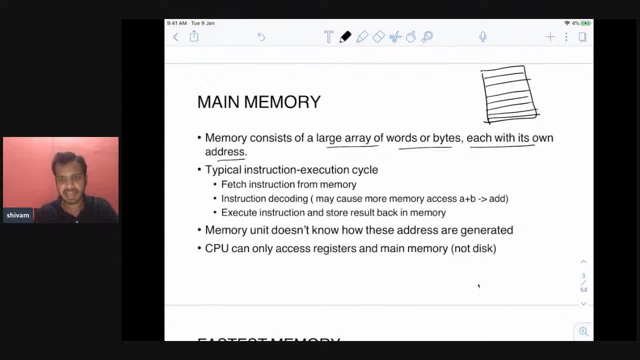 Now, in some system, what happens? This can be either like each address can be either byte addressable, So every byte is the address, And in some case it may be like you have a word addressable like maybe like like four byte is equal to one word. let's say then: basically you are considering four byte. 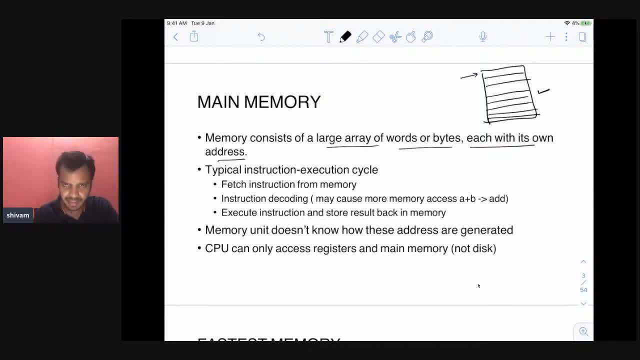 as one address. So it may also happen- It depends on system to system- But in all the examples I will take that Each byte you can address basically each byte. each byte is an address. Now let's understand the typical instruction execution cycle. 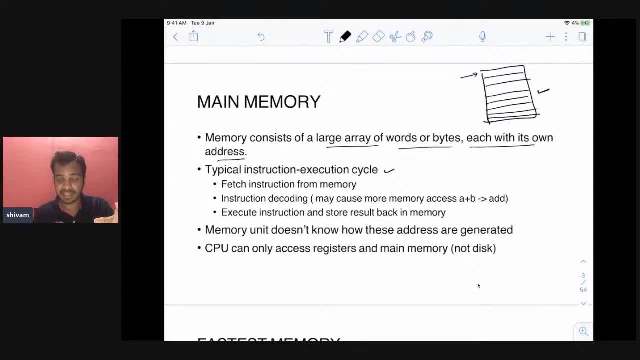 So what happens? I mean what happens when the instruction is is going to be executed by the CPU. So the first thing is the instruction will be stored in the RAM. From this RAM, the CPU will be there, the CPU will have registers. 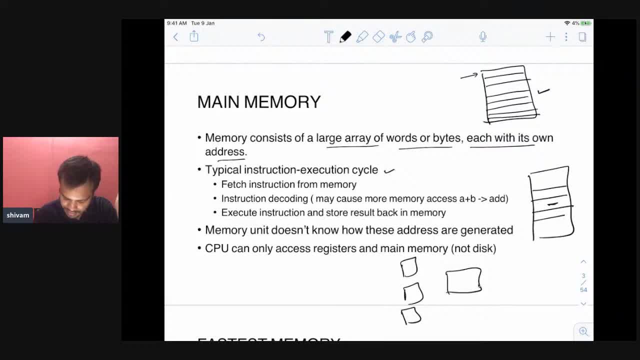 So, first, what will happen these instructions is, let's say, the instruction is add- right Now. these instructions need to be stored in the RAM. Okay, So the instruction needs to be phased to one of the registers near the CPU, right. Once this is done, instruction decoding. so instruction is add now. decoding of this instruction. 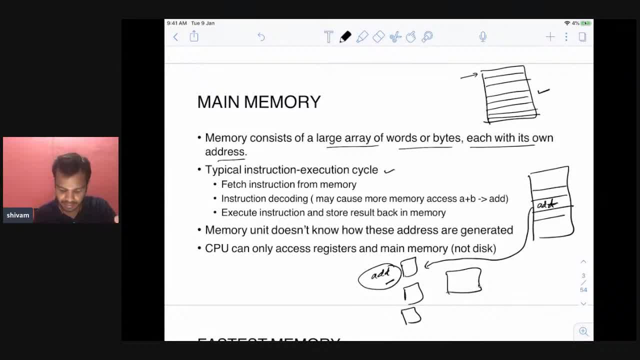 will happen like: this is add instruction. now CPU will understand this is add. Now there may be some more memory access. why, let's say, there is add A plus B, right? Then you also need to fetch A and B from different memory addresses, right? 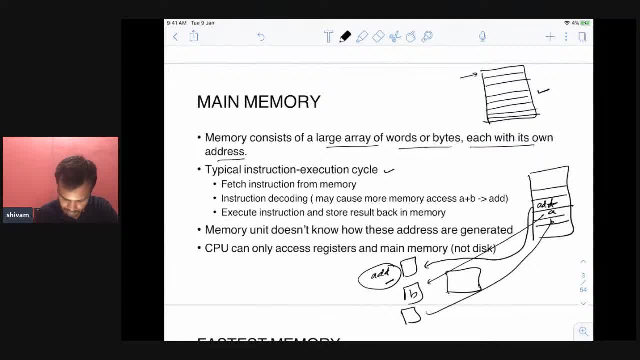 So let's, A, B and C will also be phased here. Now, once all these values are phased. now, add is phased and B and C are also phased. Now what we, what what CPU will do, is so it has ALU and an arithmetic logical units. 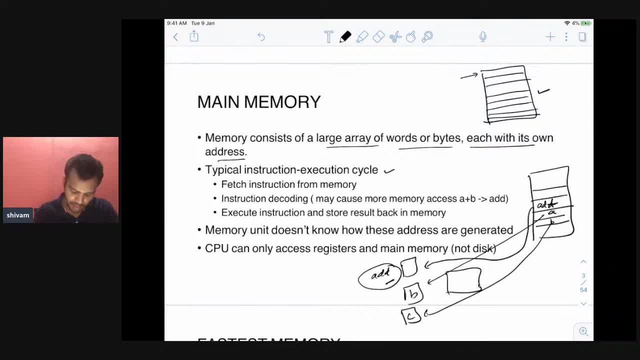 like to do the computation like here. addition is the computation computation. So it will add the values of A plus B and later there is a fourth register. it will store this value, A plus B- let's say it's A plus B- in this register. 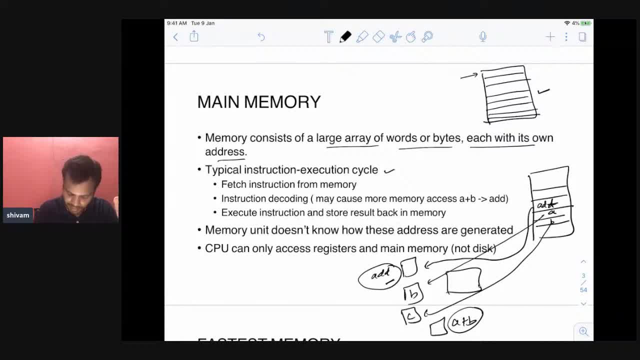 And once this calculation is done, execution is done, this value will be again written back to somewhere in the memory. So this is the typical instruction execution cycle. that happens is it performed by the CPU And always understand that memory unit does not know how these addresses are generated. 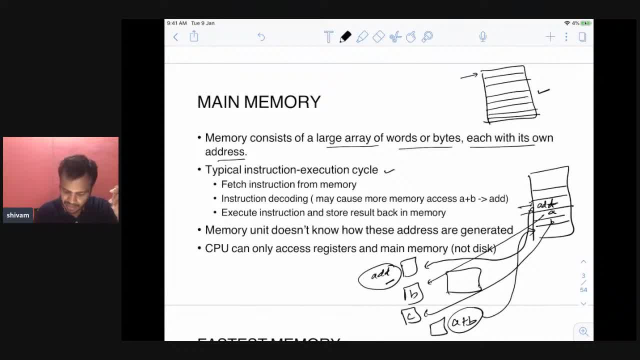 So, like every like, every value will have an address here. but a memory management unit does not know the method, how this address was generated. It will only know: this is the address, that's, that's all I mean. it does not know how it. 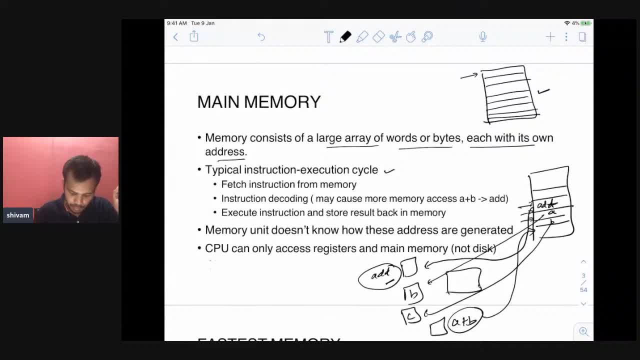 is calculated and everything. Now also, you CPU can only access registers and main memory. I mean this is very important. CPU cannot go and access the disk directly, first the, I mean first the container. The content has to be bought from the disk to the main memory, then from the main memory. 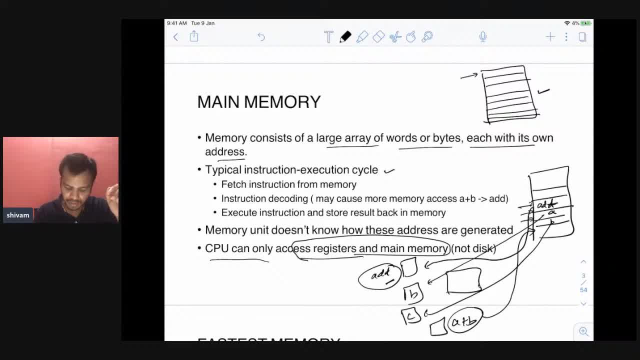 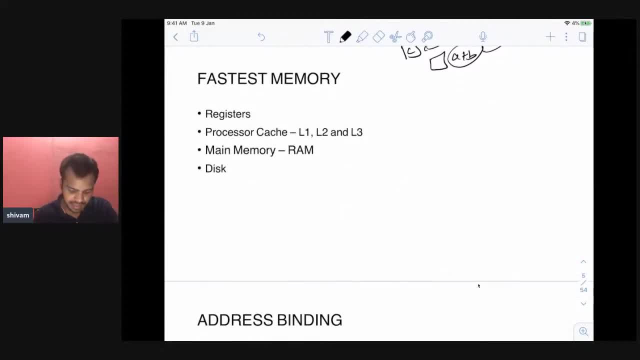 to the register, then only CPU can work on that. This is very important to understand. So, these basics of operating system, I will say, and let's go on to like the which are the fastest memory, if you see. so registers are of course the fastest ones. 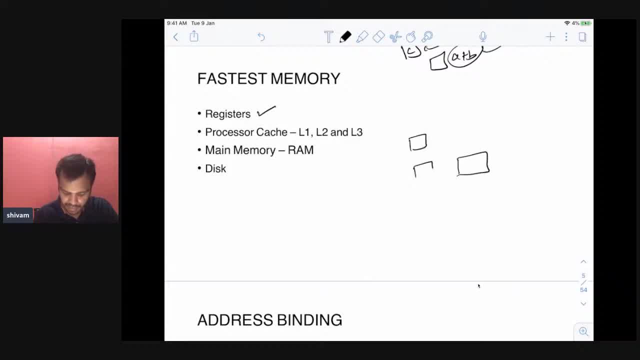 So if you have CPU, the closest one, the closest memory to CPU are the registers. these are the closest to the CPU. Then you have processor cache also. like they are a bit far away, let's say this is the RAM here. 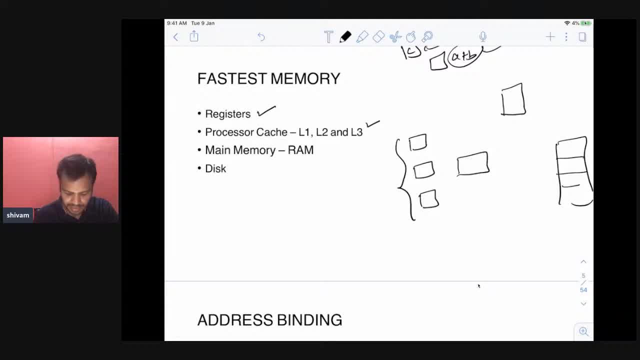 So then you have, you will have processor cache will be, which will be a bit far away than the registers, But we have the second, fastest, I will say- memory for the CPU and the last one will be main memory. So main memory will be the last one. 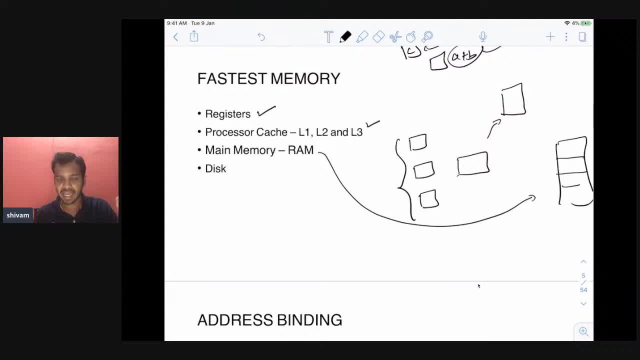 I mean it's not very fast. I mean you will think that, okay, RAM is the fastest one, but no, the registers and processor cache, these are the fastest one. And at last, it is the disk. I mean. disk is the slowest one, I mean, and also the CPU. 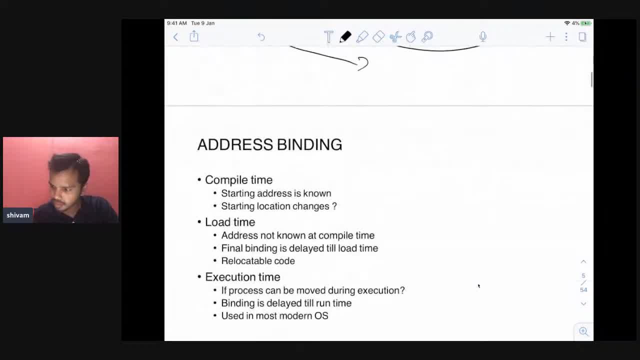 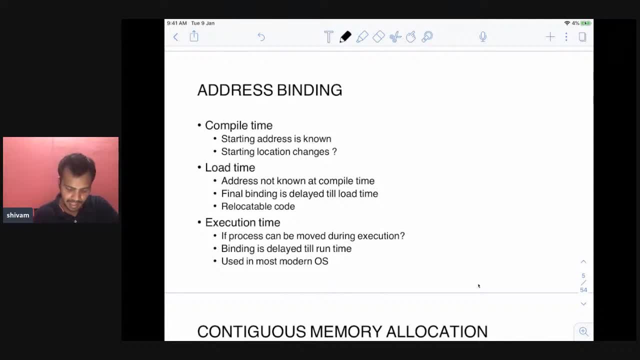 cannot directly access the disk And if you have any questions in between, do ask the questions I can answer here when I'm going through the slides And let's understand like what are the different types, how address binding can happen. So once you have created a process or a program, then address bindings will also happen. for 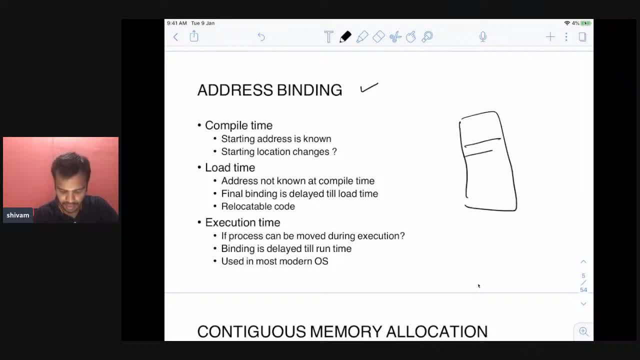 that right, Like I mean, if you have this program right, if you have this program is there, which will have multiple instructions, these instructions need to be given some address. Now this address binding can happen in three ways. 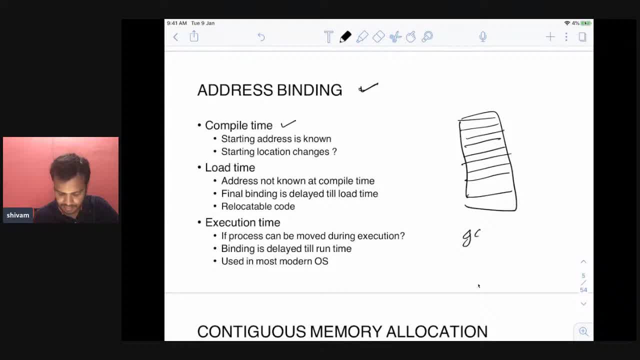 So one is compile time. So when you use compile time, So when you use GCC or G++ and compile the code itself, at that time only all the instruction can get the address also right. In this case, what is happening? 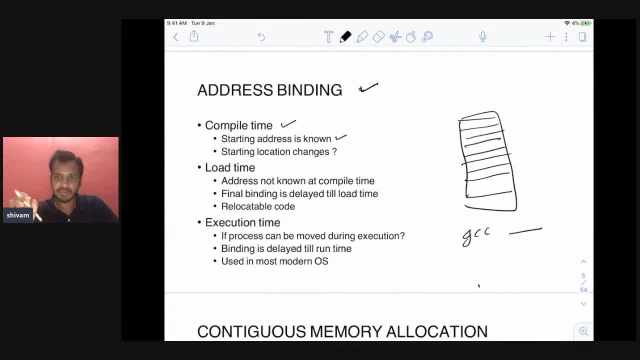 So see, compile time. you can only do compile time binding when you know that okay, at which position in the RAM this program is going to be placed. If you know that beforehand, then only you can use compile time and then you can hard. 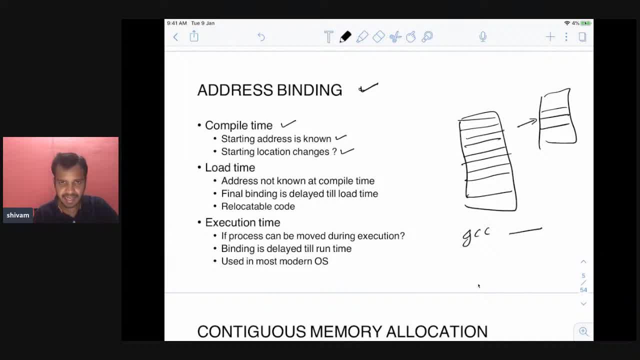 code, the address. But the issue in this is that, let's say, if the starting address changes right, you have compiled with some address, let's say 2000.. This was the base address. Now, when you are going to run the program, this address is occupied by some other process. 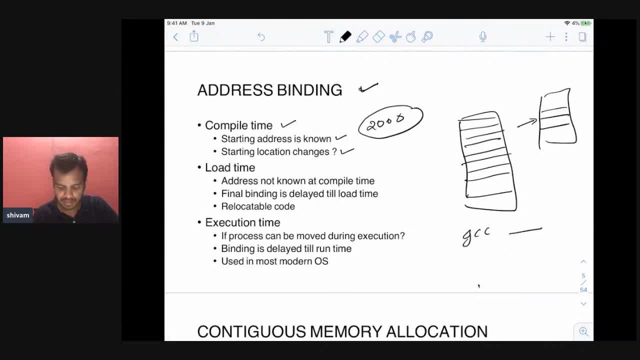 Now what you do? Now you again need to recompile the process and again basically change all the address right. There are some questions like: why was the need to divide memory all this? Why can't we have a single type of memory? 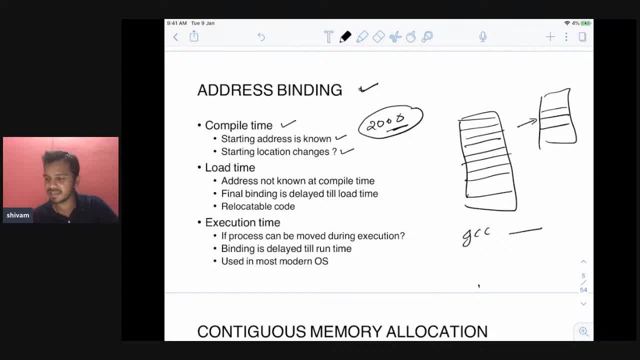 See, I mean, all the memory has some limitations. See, this is the. I will say the cheapest and the cheapest one right. This is the cheapest one right, cheapest one right. i mean this: if you want one tb of this, you have to pay very less amount and you 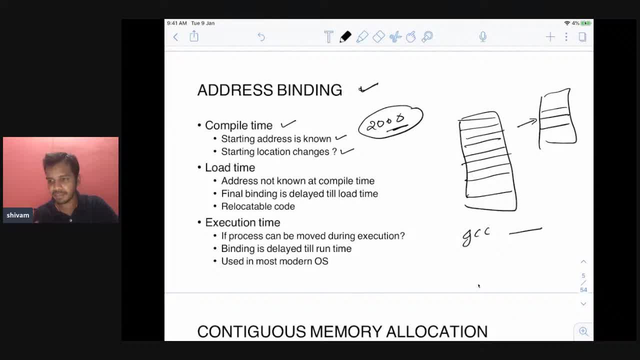 will get that. but if you want one tb of ram, right, i mean the cost is higher, right, and also you do not want to store all of the things in ram. only, ram is like it is like, i mean, you are basically, uh, it is in the memory, right, so it was able to access it, but you do not want all your programs. 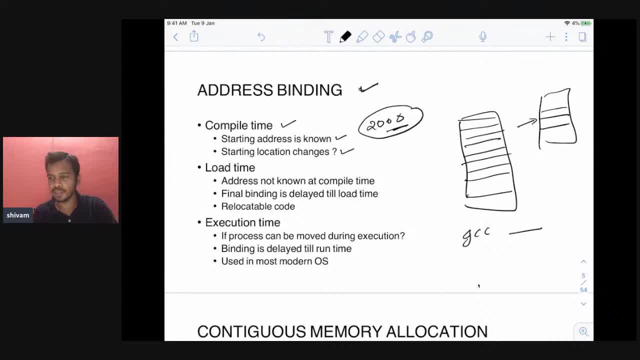 everything to be in the ram right, like, let's say, if you have like videos and music and everything, you want it to be on the disk. but let's say when you are playing it, then only you want it to be in the ram right and also understand the cost of everything, like the cost of registers is very high. 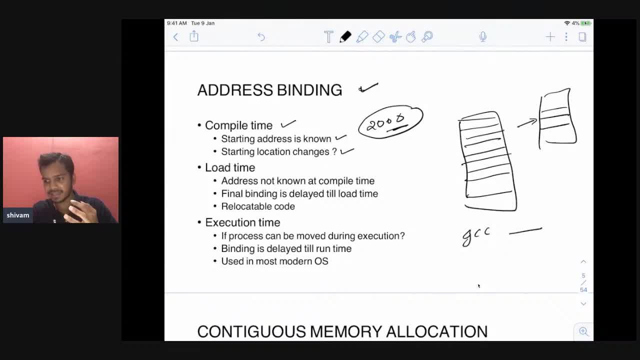 then the processor cache cost comes, then the ram and at last is the disk. so cost also matters here. so rom is not uh okay, rom is not uh, okay, i have not discussed about rom here, but yeah, rom is not same as the disk. i mean, uh, rom is again. 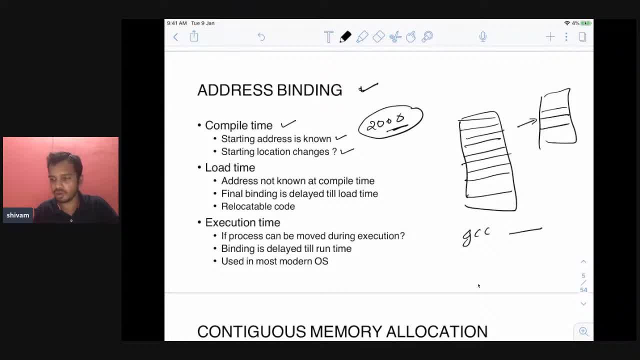 i mean you can compare it to kind of ram. i mean it is also costly, it is not very, i will say, cheap, i mean like this. but i am not covered that. i have not read much, much about rom, so i have not covered it here, because most of the important- if you see, these are the most important ones- uh, the memory. 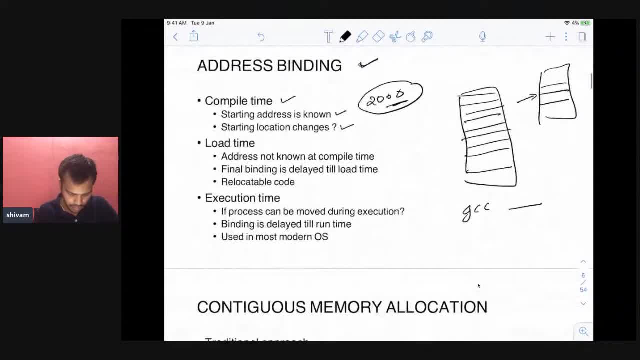 that are that are used mostly in os. okay, i discussed about the compile time. now let me go to the load time. so, load time in load time, what happens once you have compiled the code and the ruler is loading your code in the main memory right at that time, let's say you can also fix. 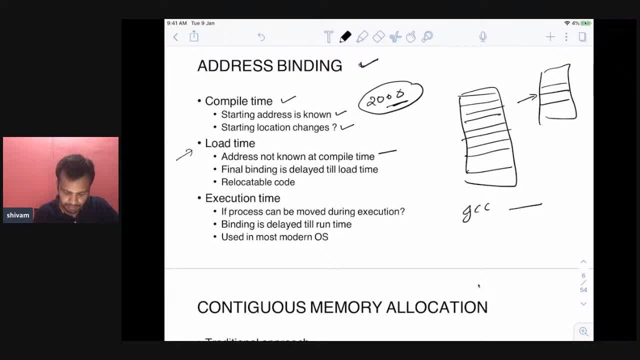 the address. in this case what happens? address is not known at the compile time. right in this, what happens? the final binding is delayed till the load time. only when the program is loaded into the main memory, then the addresses are calculated for each instruction and basically this is reload. sorry, 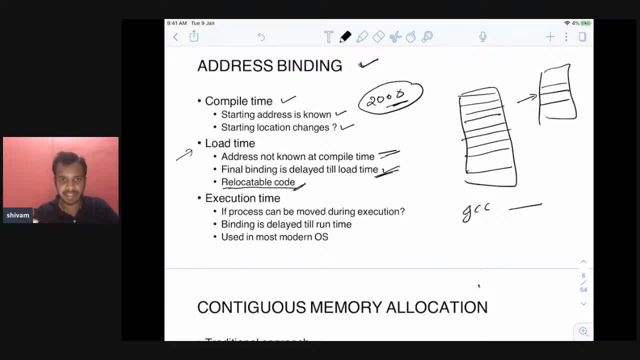 relocatable code. that means this code can be relocated easily, let's say at the load time, let's say it is loaded into the main memory and all the computations are done based on this base address. but whatever this is right, now let's say this address changes to 4000, then easily, every 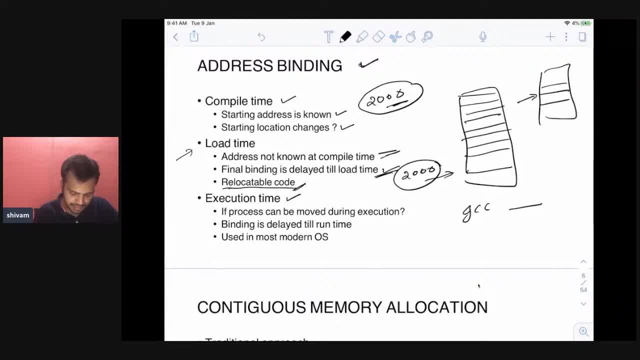 instruction will adjust to this changed address and the last one is execution time. so after loading also, program is not running. it's just been loaded, now it has to run also right now. in some cases what will happen? and if i just say in today, modern operating system, the address binding happens at: 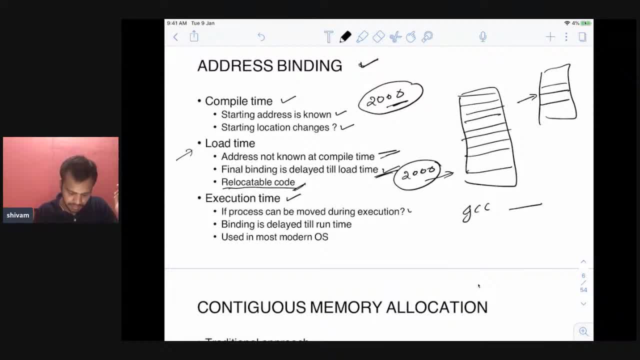 the execution time when the program actually runs. you are binding at the execution time, right now. what happens if the process itself is moved during the execution? right, if the process was somewhere here, right, it was here, let's say in the ram. now after some time it is moved to here, right? what happens? 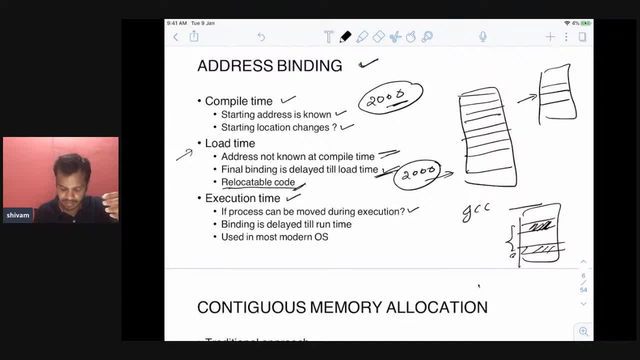 then we will discuss the challenges, how we can address the challenges. we will discuss that in this one and in this, binding is delayed till the run time, until the program runs and- and this is the actually the- using the most of modern operating system, and this we are going to discuss here. 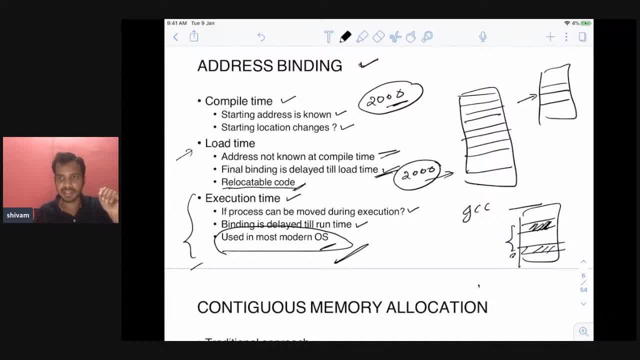 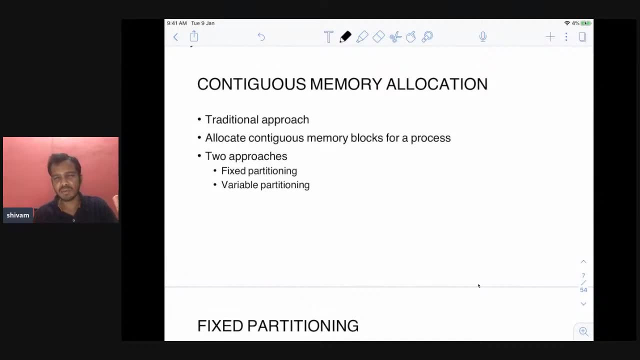 like whatever we are going to discuss here, we are going to discuss about the execution time, i mean the address binding at the execution time. these two, compile time and node time, are not much much used. i mean in today's modern of the system not much used. okay, now let's look at different memory management techniques. so first i will 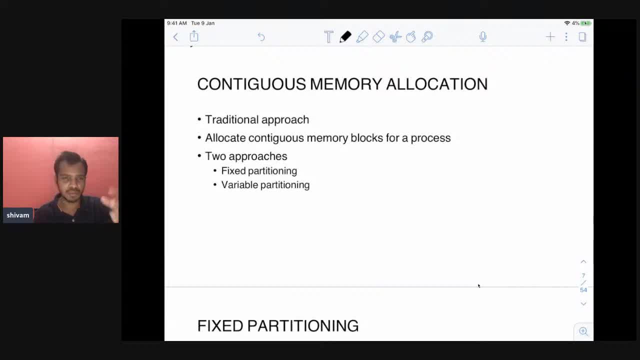 go towards the legacy. uh, i will say techniques like that was used in the old times, but let's also understand, like how the memory was used to manage in the very old time, how this was was managed. so, of course, this is a traditional approach to memory management and in this, what? 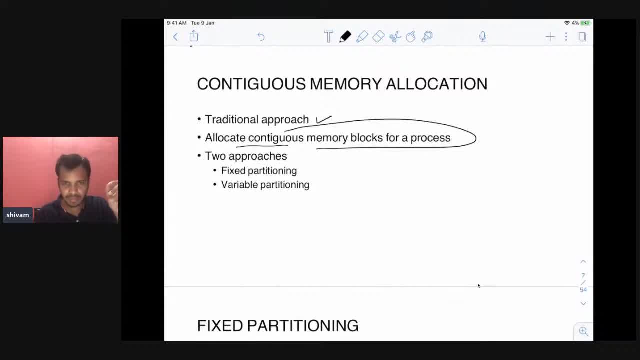 you allocate contiguous memory blocks for a process, So the memory is contiguous. There are two approaches to this. One is fixed, so what is contiguous means This is a RAM right And if you have process P right of, let's say, two KB. 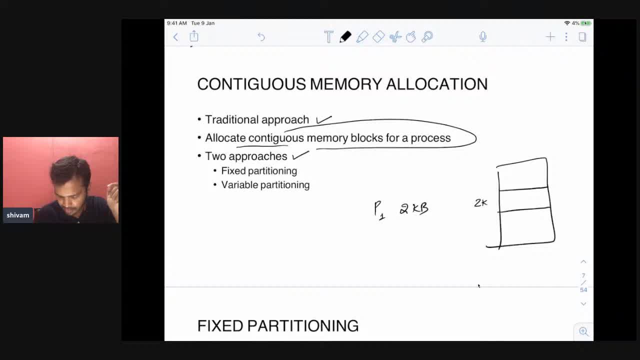 then this will be like contiguous from here to here. two KB it will be. It will not be like: okay, one KB you have allocated here and one KB you have allocated here. It cannot be something like this. It will be continuous always. 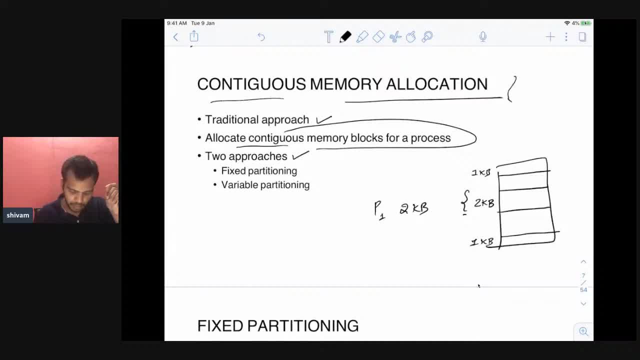 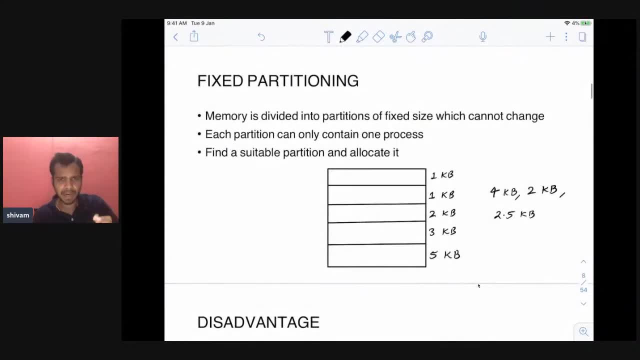 in this contiguous memory allocation. Now there are two approaches: fixed partitioning and variable partitioning. You look at both of these now. So fixed partitioning is quite simple. So memory is divided into partitions of fixed size which cannot change. So this is important. 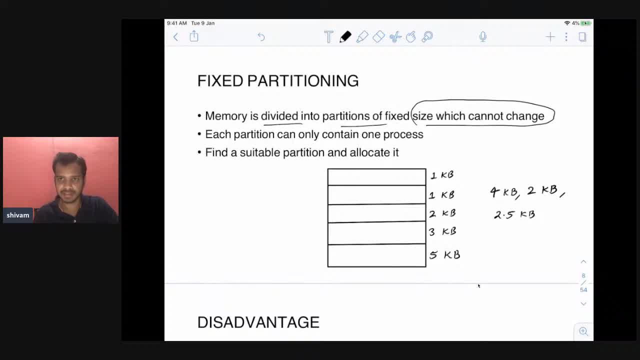 So memory is already divided into partitions. Good size cannot change. The size is all fixed from beforehand itself, Like when the system started then before that it was maybe hard-coded in the kernel code itself that this all partitions will be there And also each partition can only contain only one process. 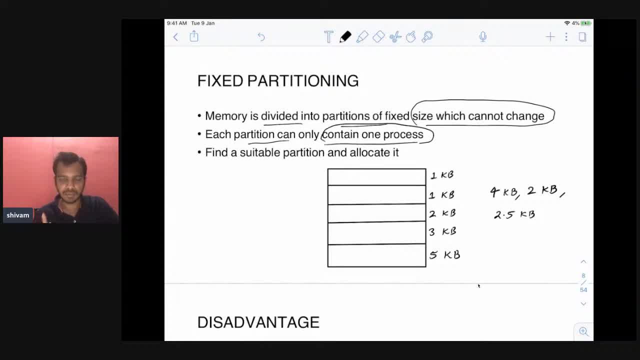 This is very important. Each partition cannot contain two process. It can only one process, And algorithm is quite simple: Find a suitable partition and allocate it You can use like a simple example. take this one I have, like let's say, this is the RAM, our RAM. 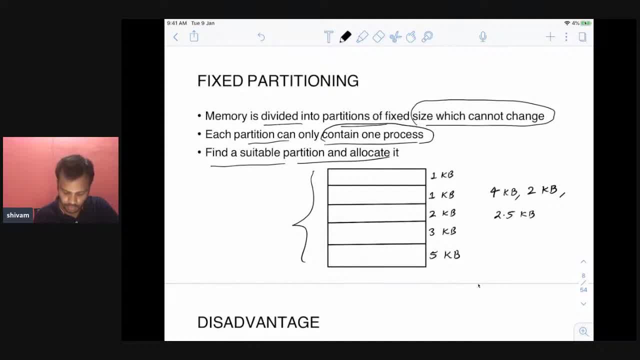 and I have like five partitions. let's say Of, one is for one, two of is one KB, one is of two KB, one is of three KB, one is of five KB. Now, this is four KB, two KB, 2.5 KB. let's say: 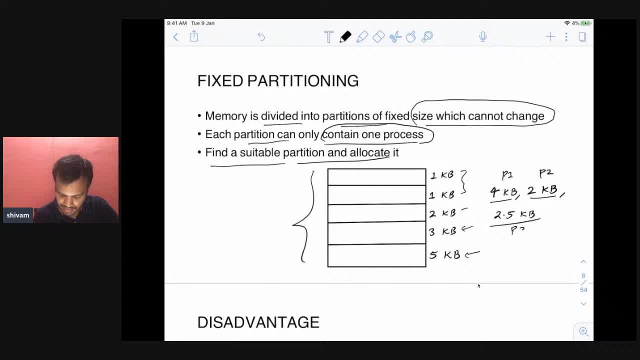 This is the process. This is P1,, this is P2, and P3.. This is the size of the memory required for all these process. Now, when four KB come, I will go from like starting to end: Okay, this is one KB. four KB cannot come here. 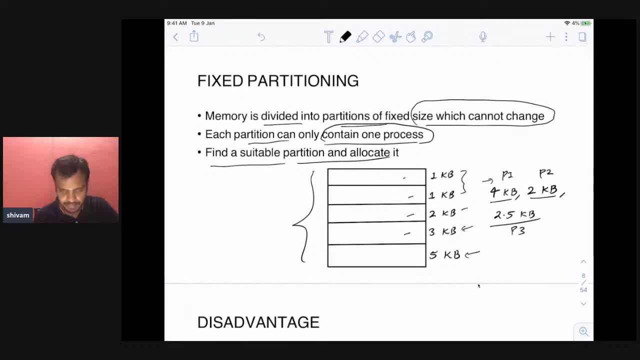 This also cannot come Here. also, it cannot come Here. no, In the five KB the four KB can fit, So I will allocate it here, This P1 to here, And one KB will be still free here Now. next one is: process is two KB, right? 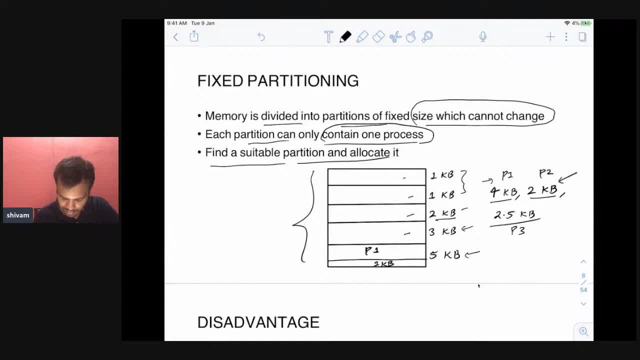 Again, I will go through from the starting and I will see that this two KB, this two KB it can fix right. So I will allocate this P2 to this two KB total. Last one is 2.5 KB. 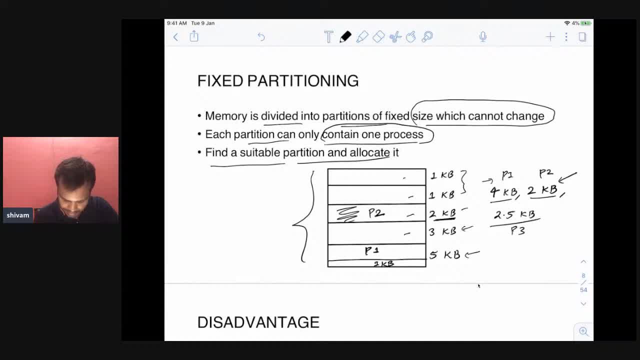 Now see 2.5 KB. if you see, I will again iterate and this one is the one, And here I will put P3, right. So this is the technique here, But the issue. if you see, here there is one issue here. 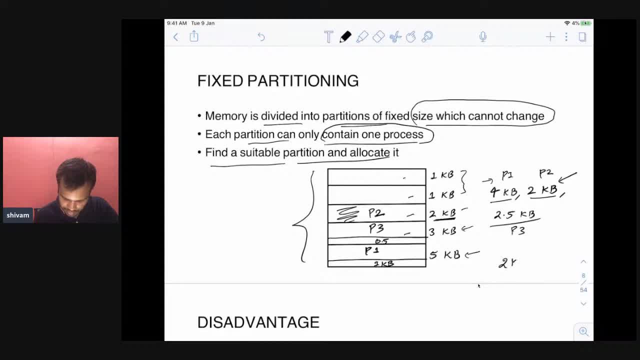 Let's say, if you have a process of, let's say, two KB coming again right Now, can you allocate this two KB? I mean You cannot right, Because, see, you have two KB, because there is one KB here, one KB here. 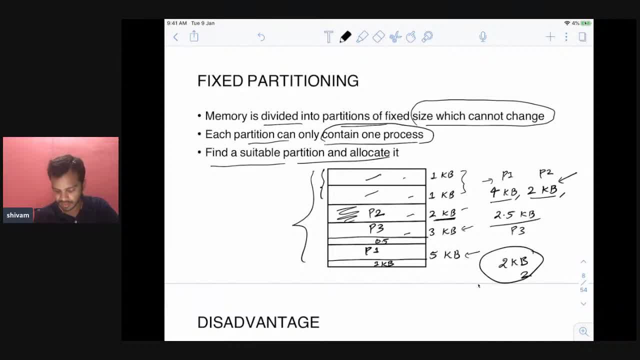 So, if you sum these up, you have two KB, But you cannot, even if you have two KB free in this RAM, you cannot allocate this two KB process because I mean, as I told you, each partition can contain only one process. 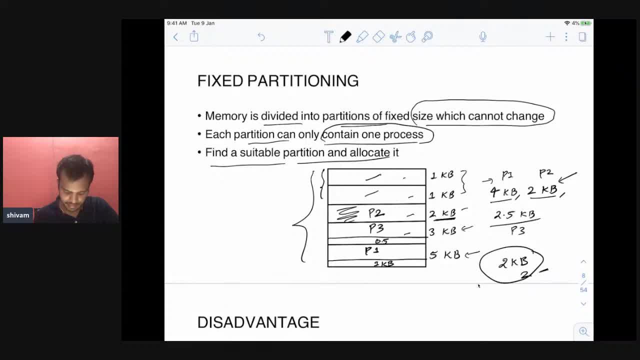 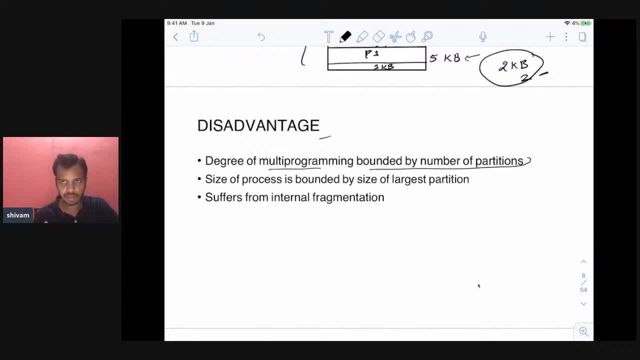 So you cannot do this. So that's the disadvantage of this fixed partitioning. So if you see, the disadvantage degree of multi-programming is bounded by the number of partitions, So basically the maximum number of process that you can have in this. 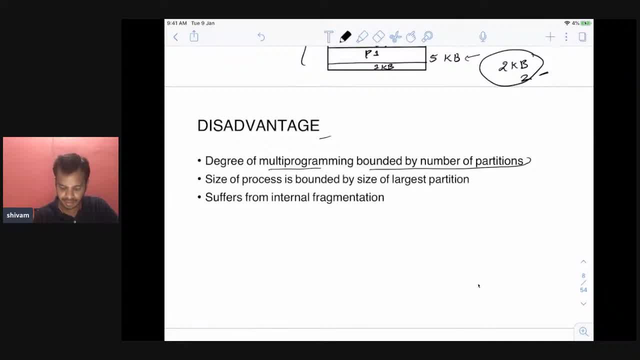 using this technique is equal to the number of partitions. you have right. Let's say, if you have five partition, but if you want to run six process, you cannot run it here. Also, size of the process is bounded by the size of the largest partition. 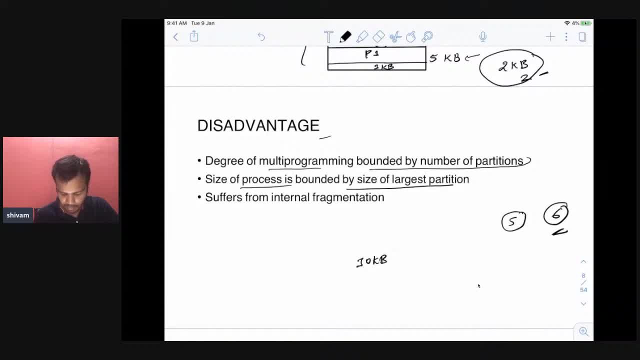 That means, let's say, if your process size is 10 KB, but the largest partition size here is only five KB, then you cannot run this process. You cannot run this process. Also, this suffers from internal fragmentation. So this is very important here. 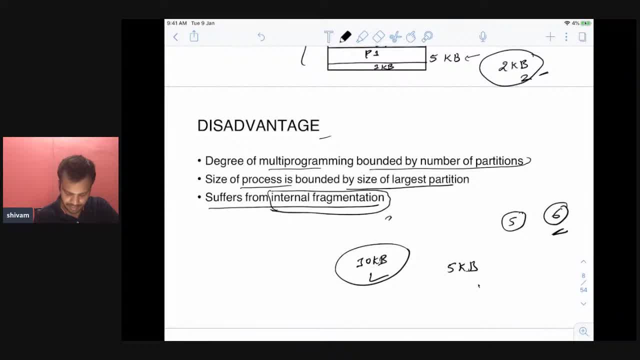 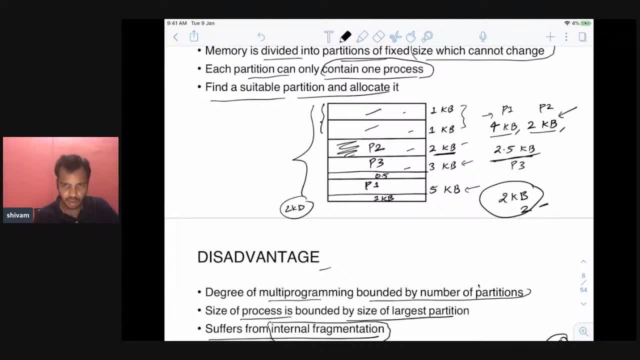 The fixed partition method suffers from internal fragmentation. I told you right, For example, two points, for example two KB. you did have I mean two KB, but you were not able to allocate it. So this is called internal fragmentation, right. 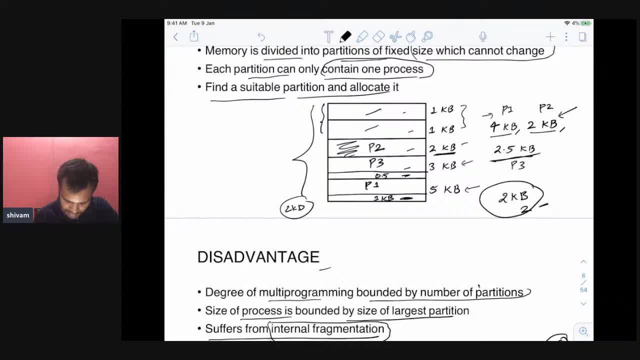 Also, if you see, there are some internal fragmentation created here, also right of 0.5 KB, of one KB, And you cannot use this fragmentation because, as I told you, one partition can only include one process, So this one KB is wasted. 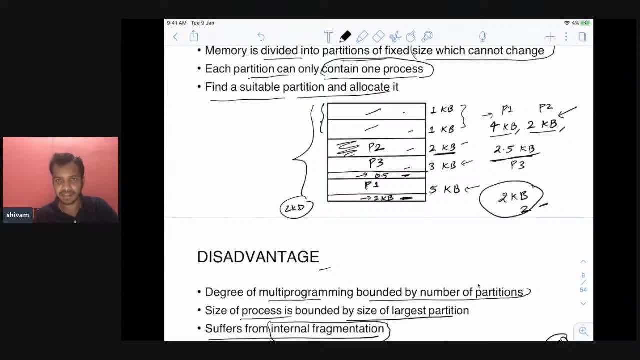 This 0.5 KB is also wasted, And this is called internal fragmentation, because each and this fragmentation are internal and this is related to the partition itself. That's why it's called internal fragmentation. So I hope you would have understood this. 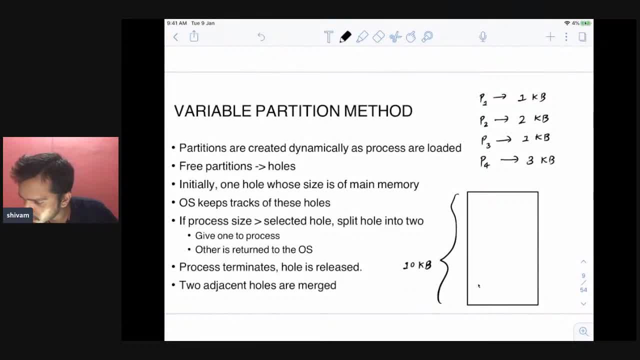 There are some questions. Yeah, so Harshith has asked what is mean by term binding? Yeah, it means the same. Yeah, you have to assign: like, for each instruction you have to assign an address. That is called address binding. 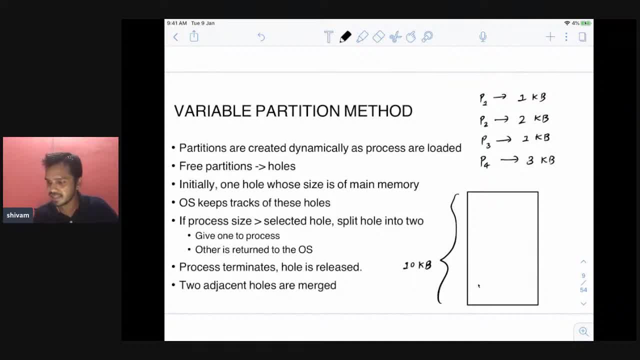 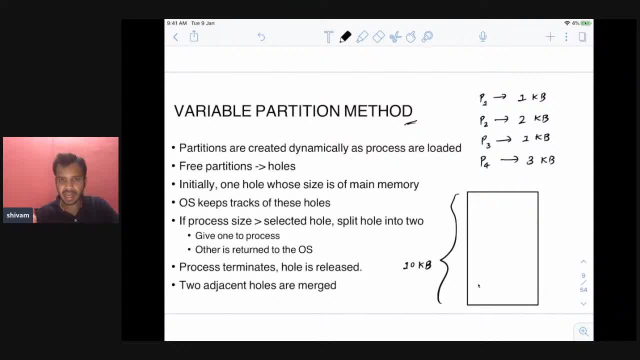 Okay, next one is I will cover is variable partitioning method. So this: I already gave the example of fix partition. let's look into variable partition Here. what happens? partitions are created dynamically as process are loaded. So there is nothing like okay. 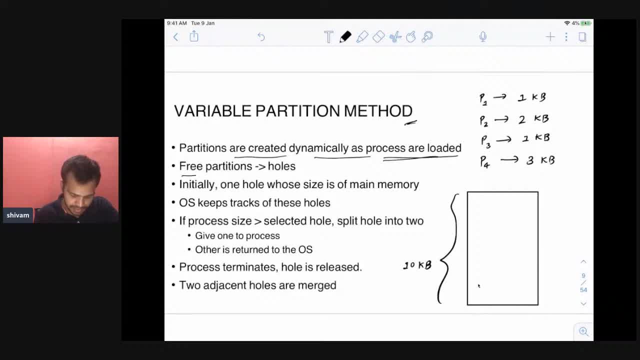 there is fixed partition, There is nothing like that here, And free partitions are called holes, right? Okay, I'll give an example, you understand, And initially there is only one whole whose sizes are the main memory. See, initially there is one main memory. 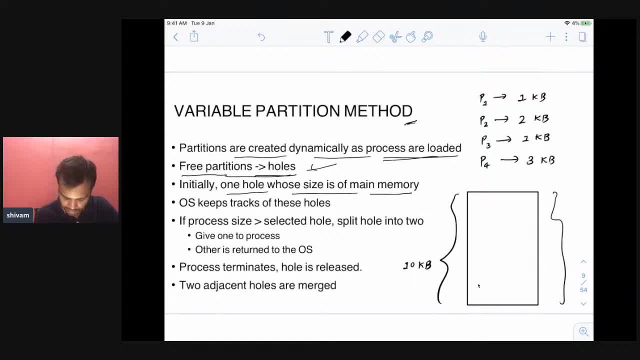 only one hole, right, this total is a hole of size 10 kb. so initially you have only one hole of size 10 kb. so hole means whatever the free partition. so this total is a free partition. now, right, this is the whole here. and also os will keep drop. the kernel will keep track of all the free holes that. 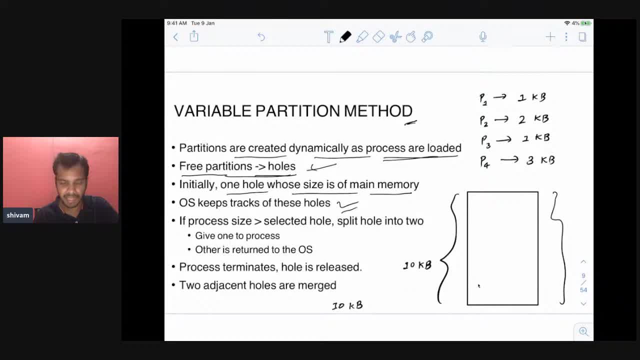 are available and it will then basically assign that to the process. now they see the condition can happen. if process size greater than selected hole, then what will happen? you will split the hole into two right because the process size is greater right than the whole size. then one hole. 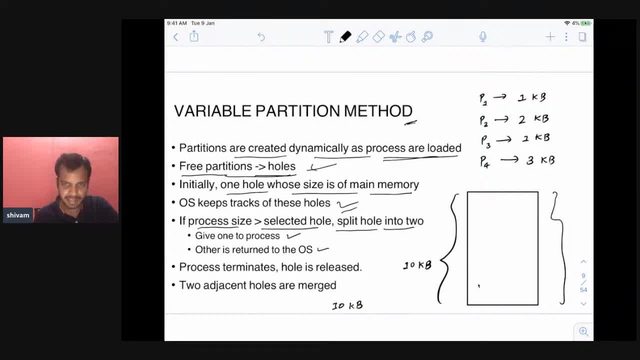 you will give it to the process itself and the remaining hole will be returned back to the os and when the process terminates, hole is released and two adjacent holes will be merged. okay, let me give the example. this is all theory, but let's see this. so initially you have one. this is a list of 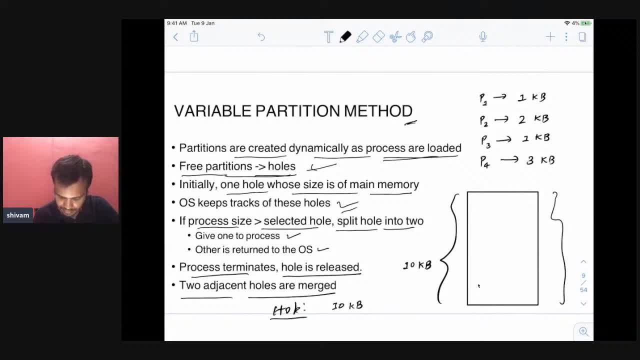 hole that os is keeping track of. initially you have hole of 10 kb. now, when the p1 arrives, you put it here even and one kb is there now. you see, now you have the os will have only one hole of nine size, nine kb. right, because this is the hole now that is the size of nine kb. right now, when p2 comes, p2 goes. 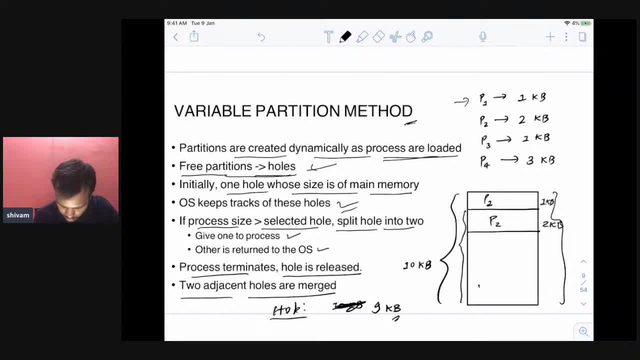 here. this is two kb now. you os will only have one hole of size seven kb. after that, one kb again. p3 comes, then the uh, there is only one hole. this is the hole of size six kb and at last there is three kb process. before, three kb. now, at last you will have one hole. 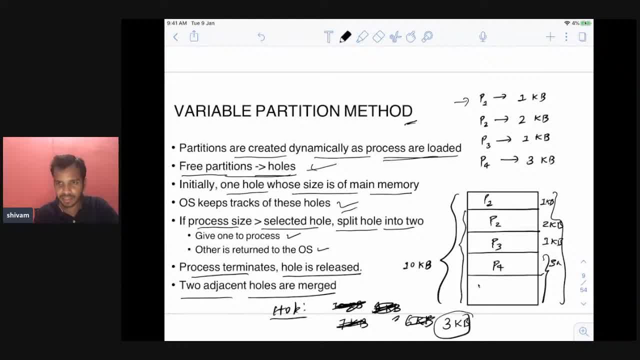 remaining of three kb, right. so this is how this happens dynamically. you are creating right now what can happen is see, some process can also terminate right now. let's say, p2 terminates- right. when p2 terminates, this uh hole of size 2kb. now see, after p2 terminates, one new hole will be. 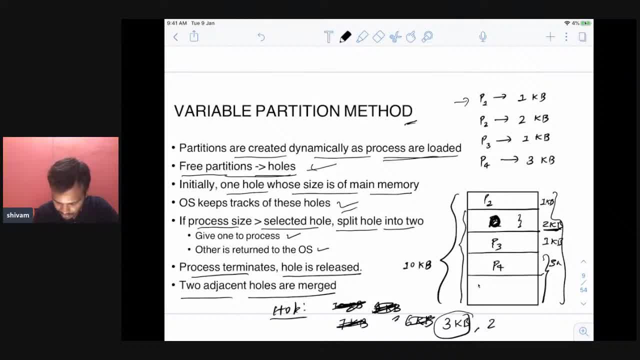 created, right? so this 2kb hole will return back to the kernel. now you will have two holes of size 3kb, right, and let's say, p4 also terminates after some time. then you will have, uh, this, this is also a hole that will be returned- and 3kb, but actually these two will be merged, right, as i told you this. 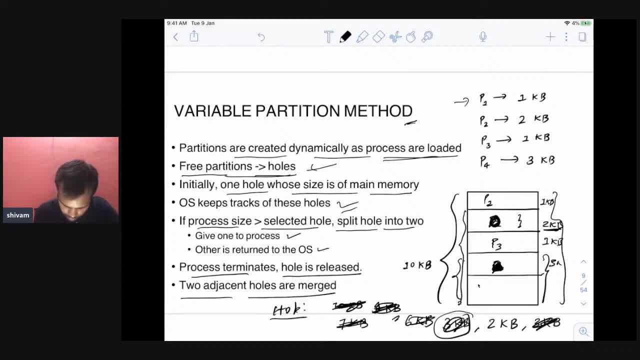 truly must, and this will become so. these two will be merged and you will have again. let me write: you will have two holes, one of size 2kb, one of size 6kb. so this is how it happens, right. but there is one issue here. the issue here is that, see, let's say, if you have seven kb, process right. let's say: 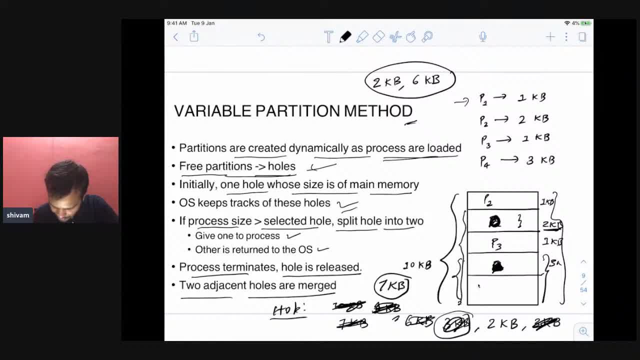 if you have seven kb process, right, but total uh free memory you have is. or if you see total free memory you have is totally 8 kb is free and now you have a process of 7 kb, but again you cannot allocate this because these two holes, if you see this hole and this hole is not continuous and we 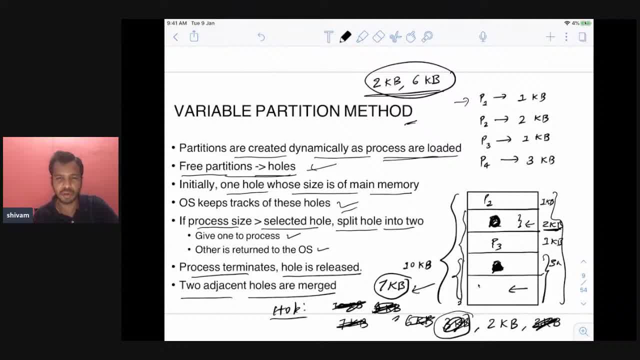 are in the continuous memory approach. that's why you cannot assign it and this is called external fragmentation, because you have that memory right, you have 7 kb of memory in the ram but those are not continuous and this is because, see in variable partitioning you will have 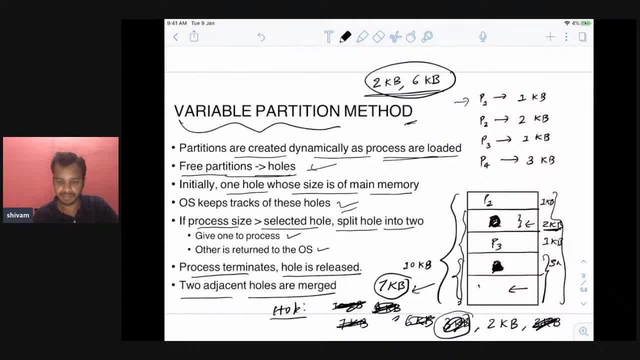 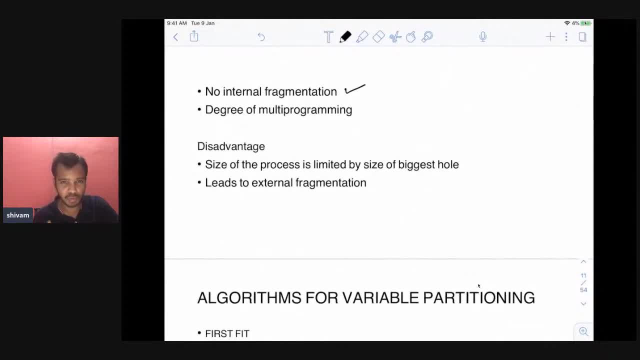 this external fragmentation and in fixed partitioning you will have, uh, internal fragmentation. that's important to remember. so, of course, in this there is no internal fragmentation because there is no partition here. right, the partition is not fixed here. also, degree of multi programming: you can run as many programs as you want, right? there is nothing like it's fixed, right. 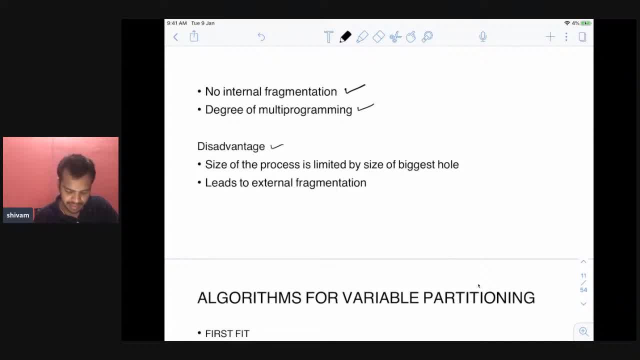 initially. but the disadvantage also is advantage here- is that size of the process is limited by the size of the biggest hole, right. that limitation is here also right because this is continuous memory and this leads to external fragmentation. so this is the main disadvantage, i will say, of this. 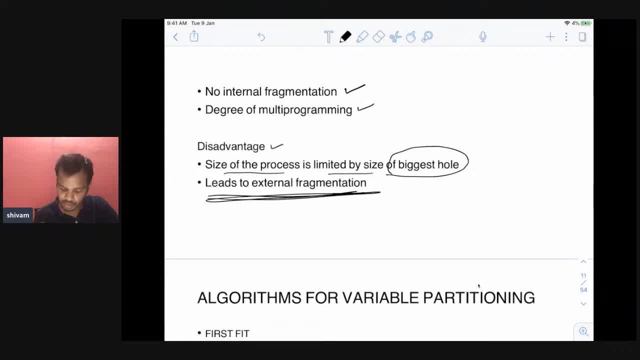 because, see, external fragmentation is very bad. i mean, you have you in. in that case you had eight kb of memory free and you wanted to allocate a process of seven kb. but you cannot allocate it because these are not. one one was of six kb and one hole was of two kb, and these are not. 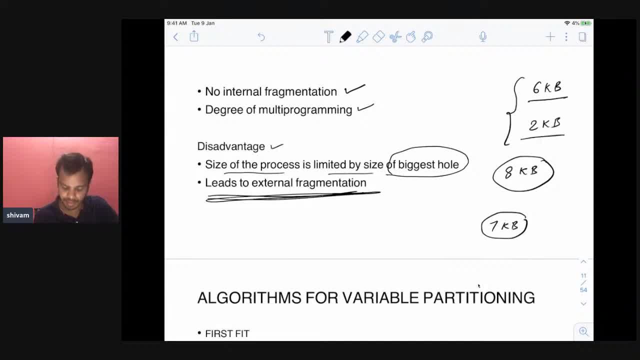 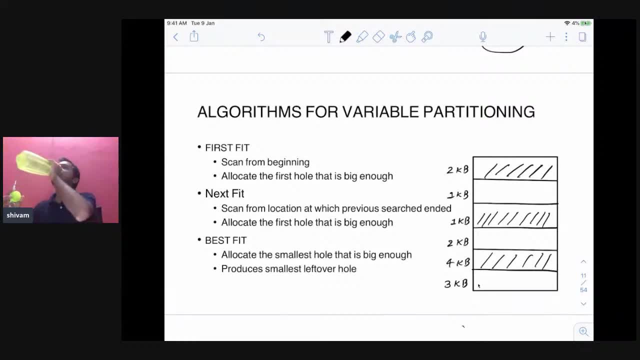 continuous. that's why you cannot allocate it. that's very dangerous. i mean, okay, let me, just because this session may be a bit long, so okay. so next is the. there are some algorithms for the variable partitioning, right. so these algorithms are: uh, first fit, next fit, best fit, and last one is worst fit, right. these algorithms are: 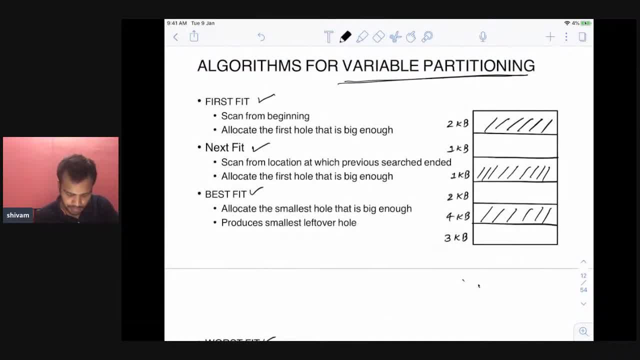 quite simple. see in first fit what you do. you scan from the beginning. let's say example: if you have, let's say, two kb of new process and let's say this is the, i mean, this is the state of ram after some process has come and, uh, left out, right, this is a state, let's say final state, at this moment. now, if one. 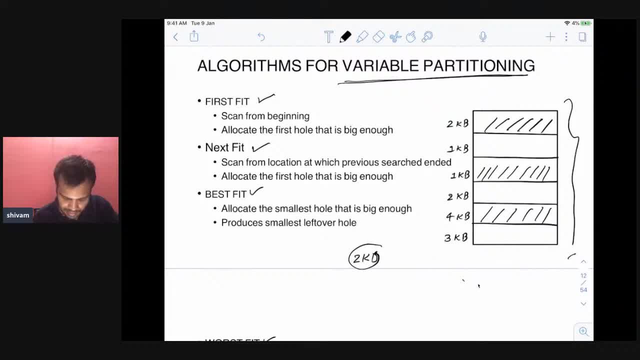 two, three process comes, you start from the first. uh, i mean you start scanning from the beginning, right? so this is the first hole you scan, but this size is one kb, so this cannot fix here. when you go to the next hole, that decides two kb, here it can fix. so you allocate this hole to the 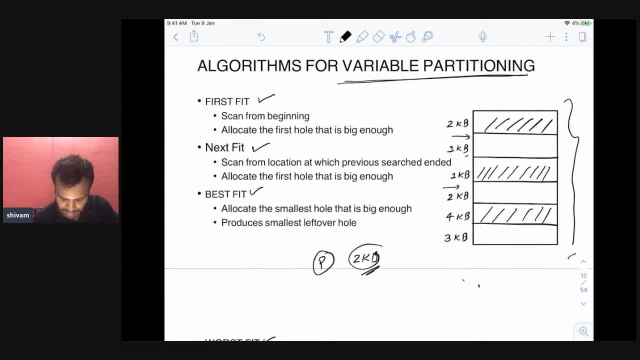 uh, process, this one, this process peak, let's say, this process was p. you allocate this hole to this process here, right, this is quite simple. this is first fit right. so you start, you scan from the beginning of this, right, you have to only scan the holes. right, because this is occupied, why you need. 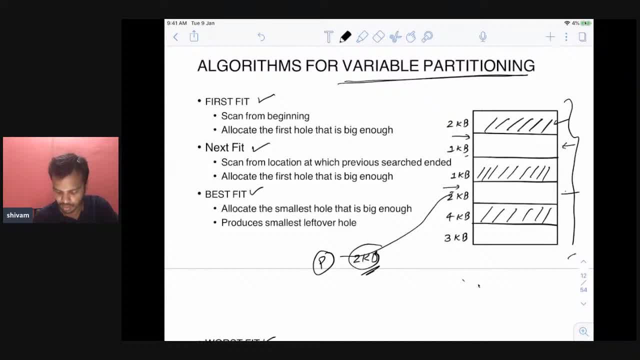 to scan this only one. this is the whole. this is the whole. this is the whole. only scan these three holes and whichever first is bigger than this one or equal to side whose size is greater than or equal to this one, put it there now. next fit is quite simple to and similar to first fit right. 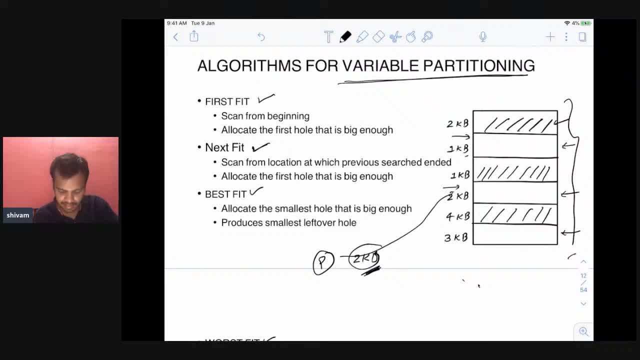 this is what happened. scan from the location at which previous search ended. let's say after this: another process comes right after, of size uh, one kb. let's say right. so let's say this is p1. so now you have assigned this process p to this two kb. let's say after this: 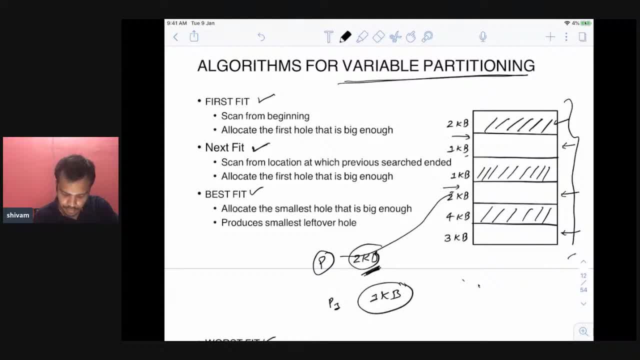 process. one kb comes now. see in first fit what you will do. you will start scanning again from the beginning, but in next fit you will start scanning from here, because your last last search ended here right at this two kb hole, right. so you will start from here. now you'll go to the 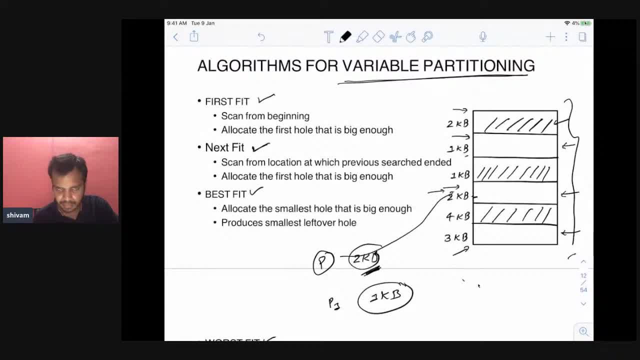 next hole, that is three kb right, and this one kb is a. three kb is greater than one kb, so this is will be put here. this is next fit. now, what is best fit? allocate the smallest hole that is big enough. that means see there are. let's say: let me remove this two, let's say: these are gone here and these. 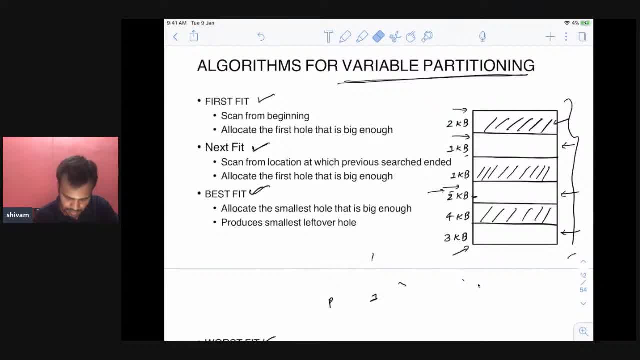 are not there and again, this is the initial state. let's say, and you have, let's say, a hole of size 2kb right now, see, you have, let's say, this is the process- you want to allocate right of 2kb. now you have three holes here: one is of one kb, one is of two kb, one is of three kb right now, see, 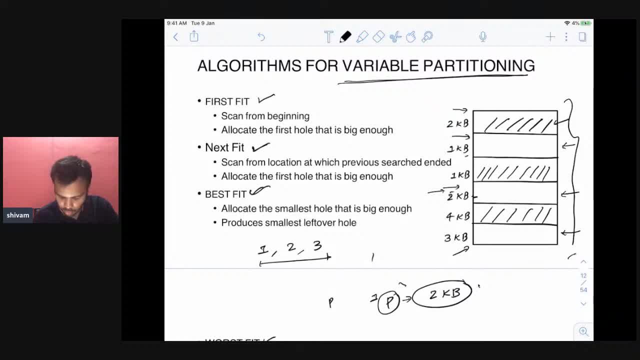 you have to find, allocate the smallest hole that is big enough, so the hole should be at least greater or equal to 2kb. which are those? these are the holes that are greater than or equal to 2kb. now, among this, you have to find the smallest one that is two right, that's. that is the uh process. 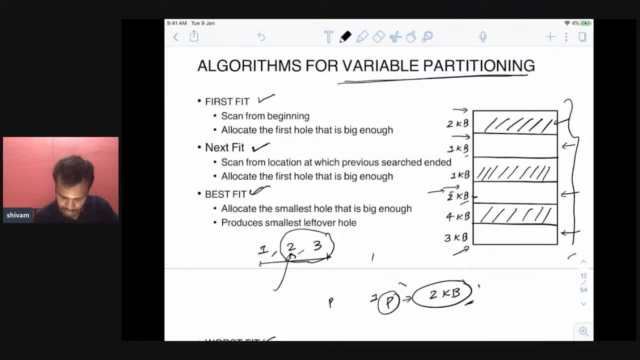 here. that means you will allocate this to the this hole, this two kb hole here. so basically allocate the smallest hole that is big enough and this will produce the smallest left over hole, because since you are picking the smallest one right, the left over part will be very small. now the last one is: 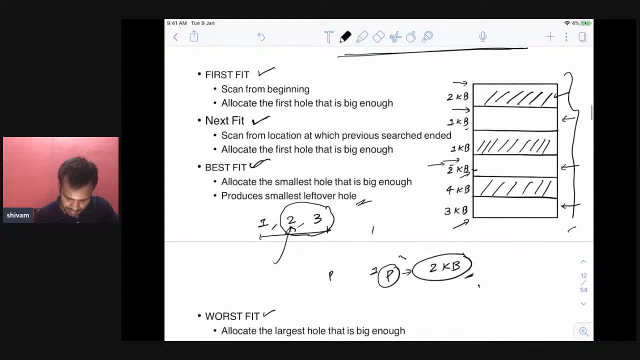 the smallest hole, that is big enough. so in the worst fit, okay, in worst fit also. you can take the example, see same, take same example. you have uh, this process, uh p is there and again it is coming off size 2kb right now. you have to find which uh holes can actually fit in this, in which holes. 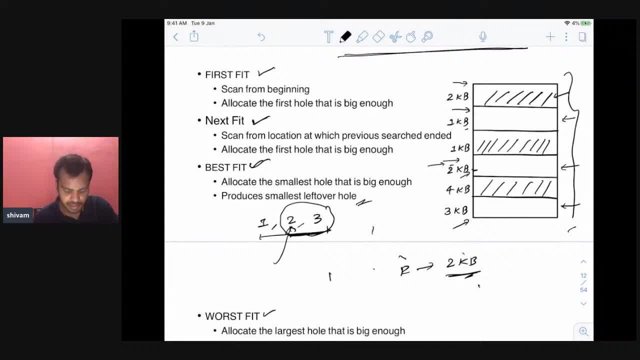 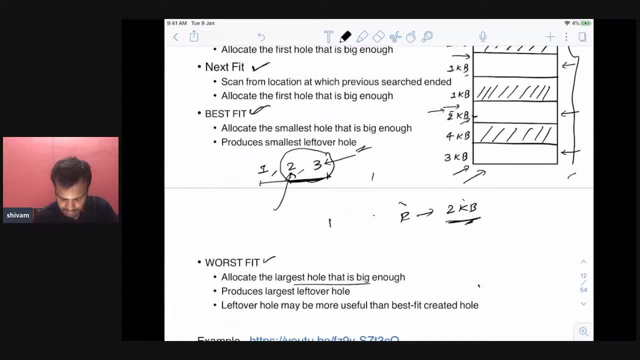 this process can fit. this can fit into two and three, these two holes, right, but among the which one is the largest one, this 3kb, right. so in the worst fit, you will assign it to the 3kb hole, so basically allocate the largest hole. that is big enough. 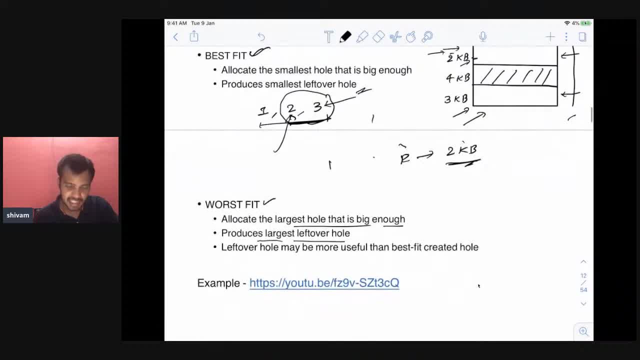 which is the largest left over hole. but don't always think that best fit is better than worst fit. why? because some cases left over hole may be more useful than the best fit created hole. see in best fit the hole can the hole which is created right can be of, let's say, 1kb. 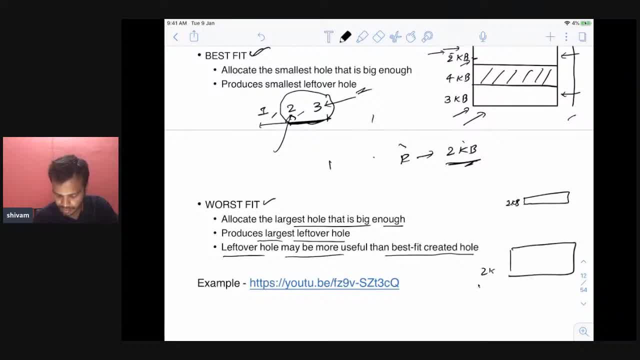 and in worst fit, the hole that is created can be of size 2kb. now, which is more useful, right? because if a process of 2kb comes, this can again be allocated to that. so don't think that best fit is better than the most popular hole. so i just want to clarify that. okay, so this is the 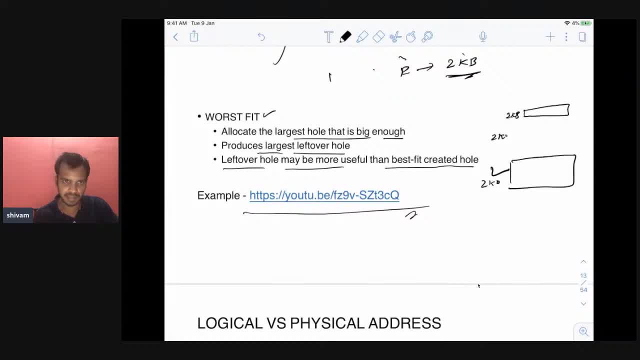 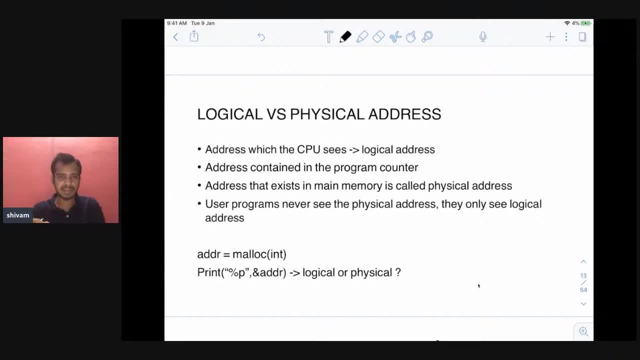 the, the. this is the, the way you can use this, uh, with different kind of situations and also, if you want a good example of this. so there is a video. i mean i've explained, with very good example there, of all these three algorithms. uh, you can also watch that. okay, so this was all about. i will. 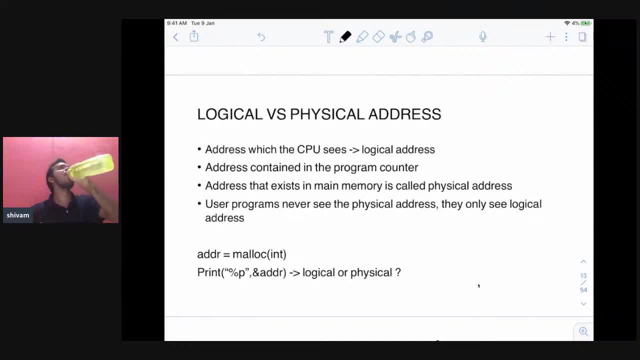 say, the traditional methods of memory management. we do not use this method now, but i just wanted to. you should know that, okay, how it was used in the old times. that's why i completed all of this, So now I will move on to the main part. 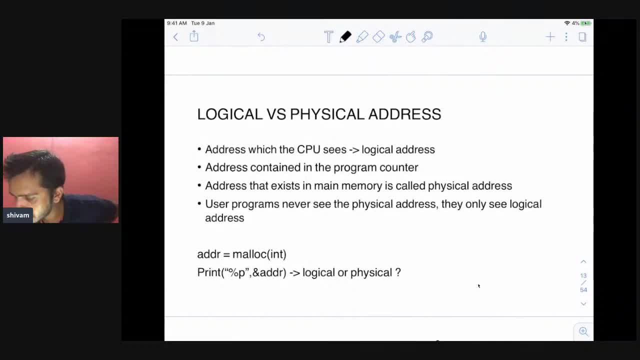 OK, there are some questions. When do deep fragmentation of disk? then what exactly happens? OK, about disk, I will cover in the next session when I will cover all the file system management. Then I will cover about deep fragmentation in disk. 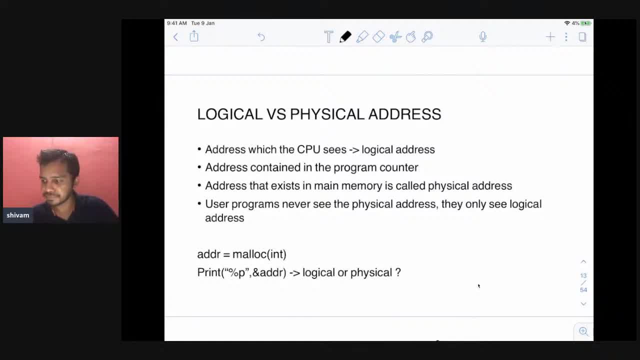 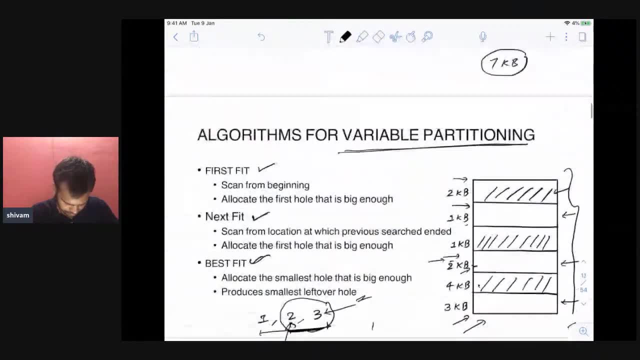 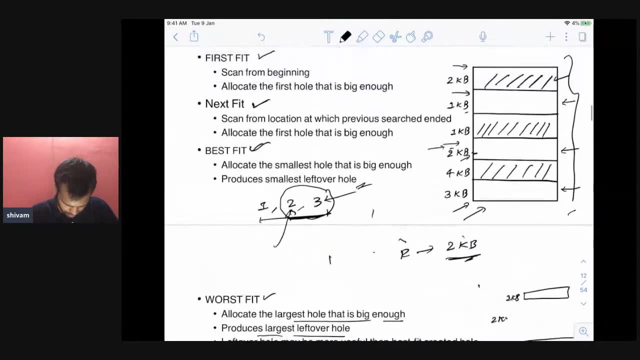 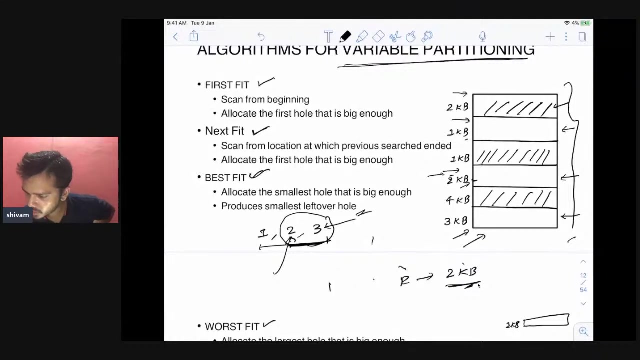 Here I am covering only about fragmentation that happens in the RAM. So now it will be process size lesser than selected hold. I am not sure which part you are commenting about. like should I do: process size lesser than? Yeah, always process size. 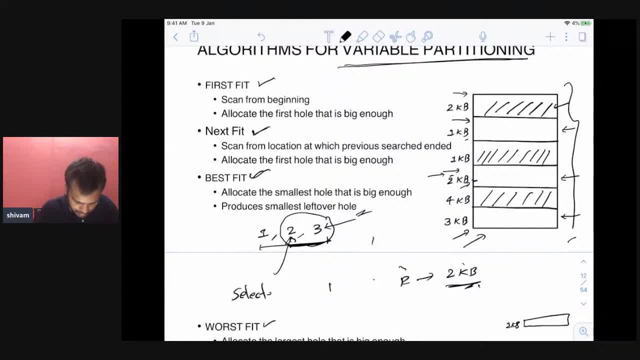 See: always the selected hold. whichever you are selecting, this will be always greater than equal to the process size. always, Always. We want to apply, We want to apply any algorithms. In any case, you have to fulfill this requirement first. 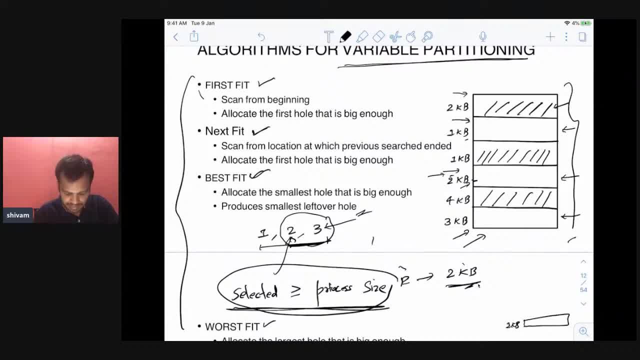 that the selected- whatever you are selecting, whichever hold, that size would be at least greater than equal to process size. This should always satisfy. Then only you can apply any of these algorithms. And if the hold itself is smaller than the process, then there is no. I mean you cannot allocate it itself. 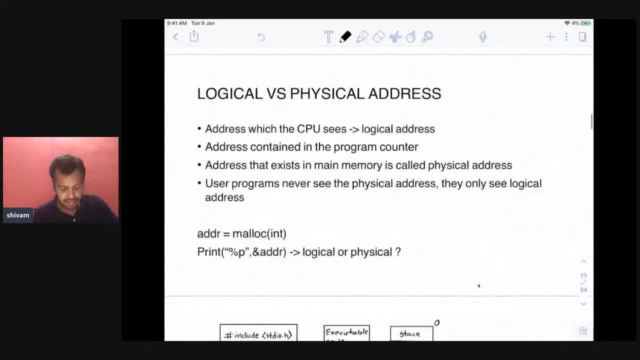 You cannot use any algorithm. OK, now let's move on to the main part, that is, logical address versus physical address. See what happens, If you remember, in the program counter sorry, PCB process control block. I told there is a register, not a register. 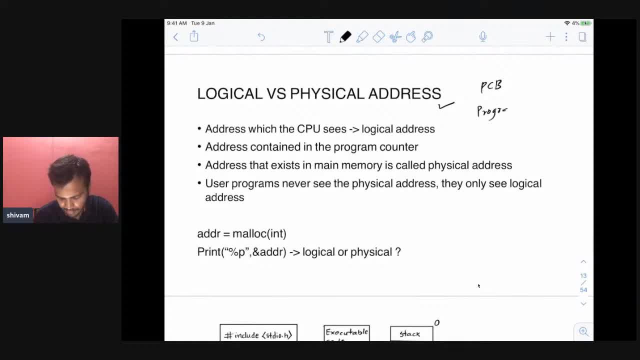 but there is an attribute called program counter, right, if you remember. Now, this program counter- what it actually does is this- stores the logical address of the process, And there is a difference between logical address versus physical address, right? So see, logical address is simply like I mean. 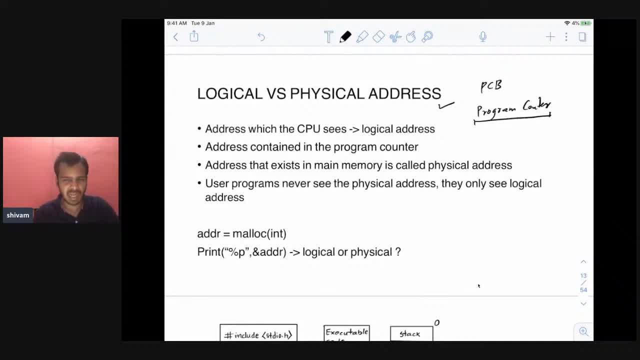 the kernel will basically see the program, like what is the size of this program and everything, and it will do some pre-calculation. Let's say, this is the logical address, right, And what the kernel will do is it will allocate, let's say, from here to here. 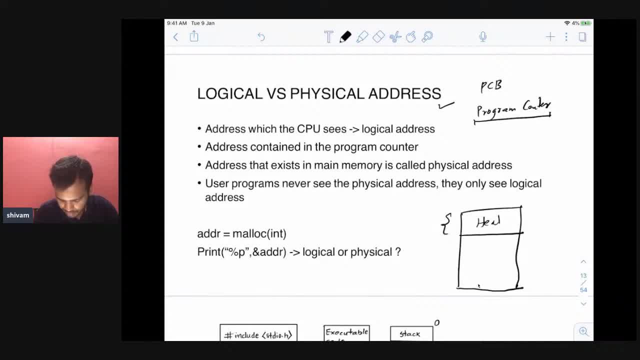 So let's say- I'm just taking example- let's say here From. let's say here to here, it will allocate to stack. let's say Then somewhere here data right, Because there are four memory segments. right, heap, stack data and code right. 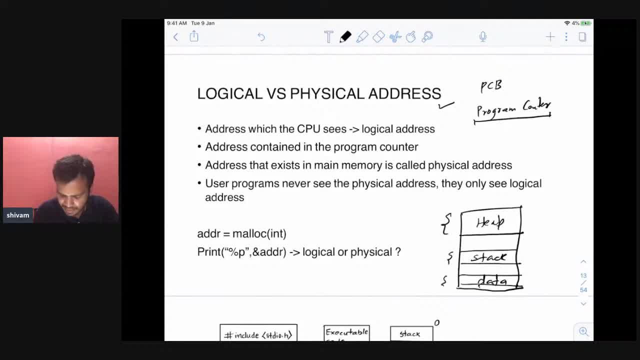 So this it will be done by the kernel itself, And here the address can be something from zero to, let's say, something max. This is called logical address, right? And I will tell you what is physical address. So physical address is see address, actually that is present in the RAM. 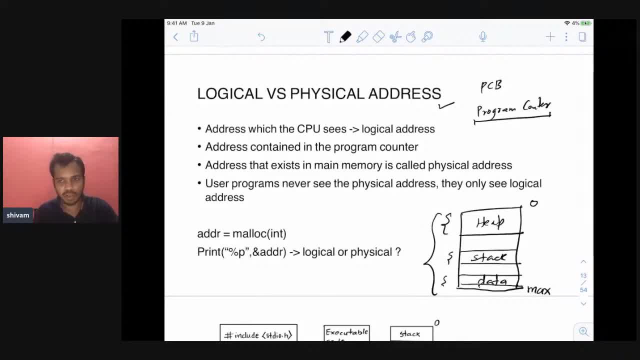 So this is logical. I mean, this is not present anywhere. These addresses are not present anywhere. These are logical. These are just stored in the your process control block. That's it, Nothing else. There is nothing, no other significance of this logical address. 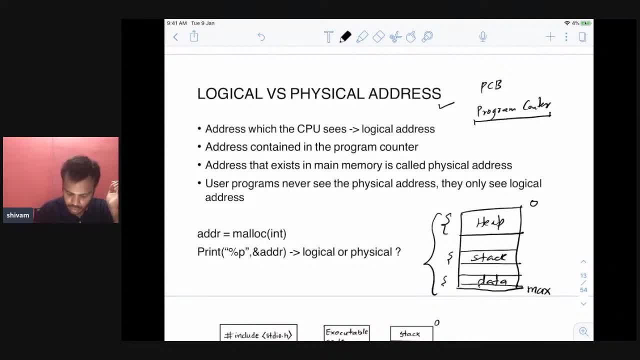 There are some addresses that are computed by your kernel and that are stored in the PCB, And the physical address are the actual address. So when you have RAM in RAM, I told you it's byte, It's addressable, right. 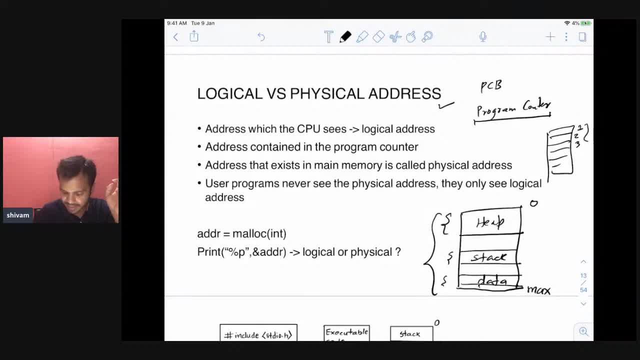 So here you will have first byte, second byte, third byte. So these address of these bytes are the physical address, actual address. So address that exists in the main memory is physical address. Now, always remember, CPU will always see the logical address. 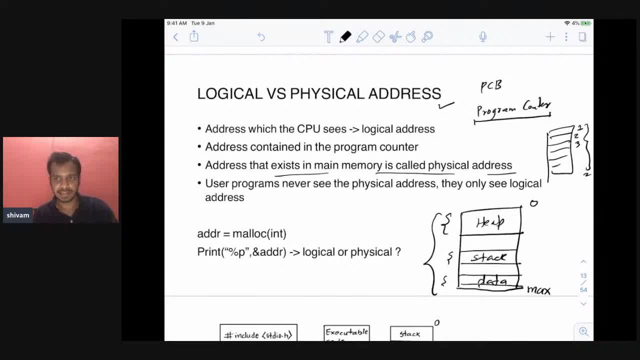 Why? Because see, CPU will always check the program counter register And in program counter register always logical address is present, right? So CPU will only see the logical address always, And also user programs never see the physical address. 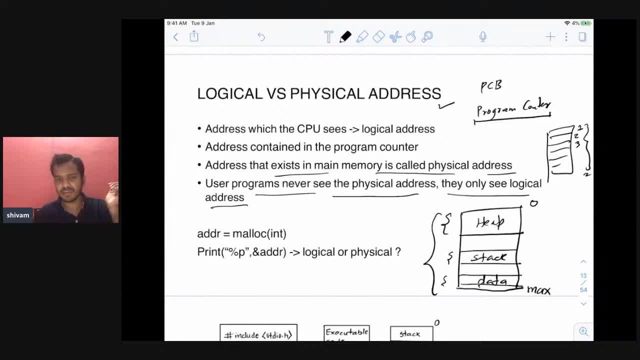 They only see the logical address. I will just tell you: try to find out for any program the physical address. You will never find it out, You will only see the logical address. So whatever address you are seeing, right anytime, you are seeing only the logical address. 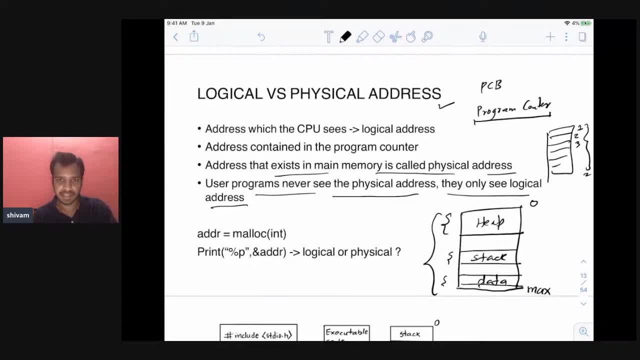 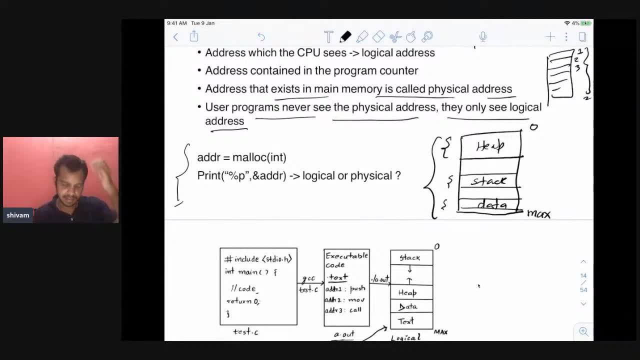 not the physical address. Physical address mapping happens differently that I will go after some time And see this, this example. I'm sure you'd have done this right. You'd have used malloc in your code, right? Let's say, you know what malloc returns, right? 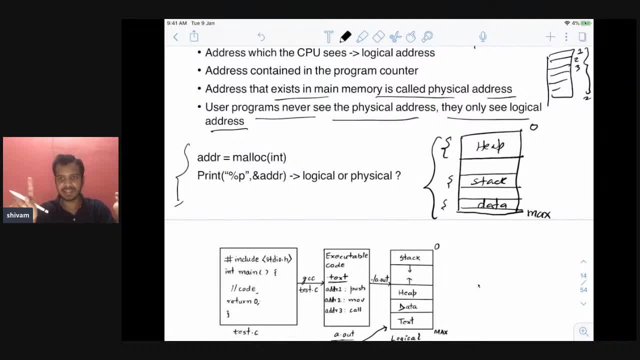 malloc returns an address to the starting. whatever the allocation is done, the starting address of that, that address is returned by malloc right Now. if you try to print the address of this ADDR, this pointer now, I will just guess. 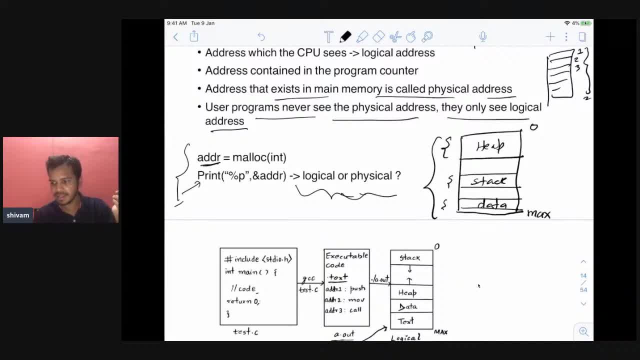 this. I mean which address you will get- logical or physical right? This is very important. I mean you will think that it is the physical address that you are getting, but no, the program will never see the physical address, never. 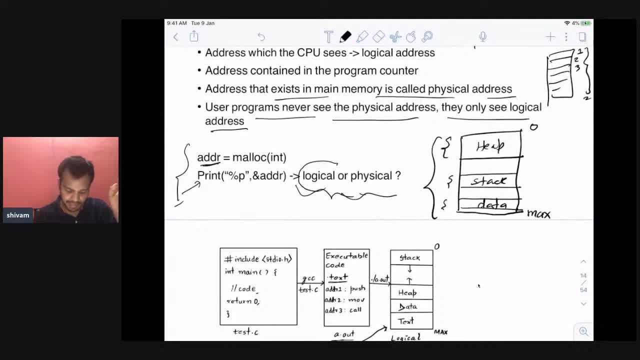 It will only see the logical address. So whatever address you are seeing by printing this address, so whenever you are trying to print the address of a pointer, you are always seeing the logical address, not physical address. And if you go to Linux, use any command line, anything, you will always see the logical. 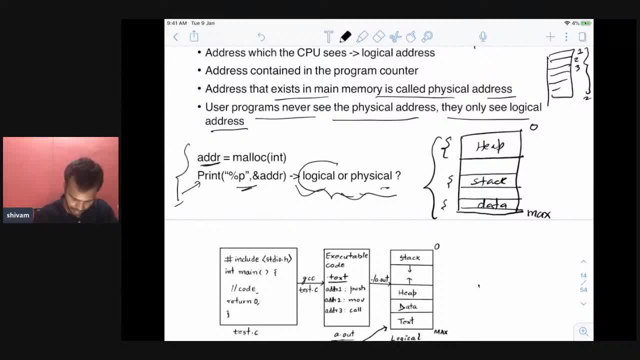 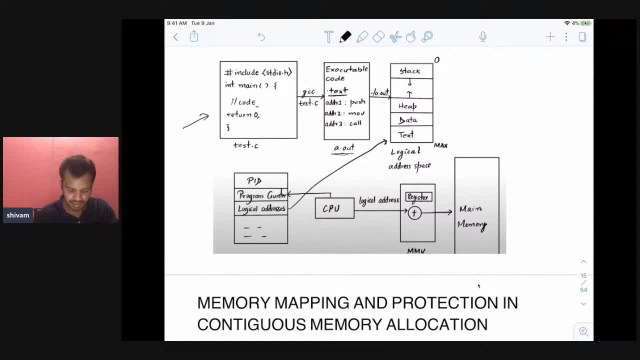 address, not the physical address. Okay, This is a diagram example I have given like: you have the program. right, You have the program. let's say simple program is there Now, once you compile this, this is broken down into executable code, right? 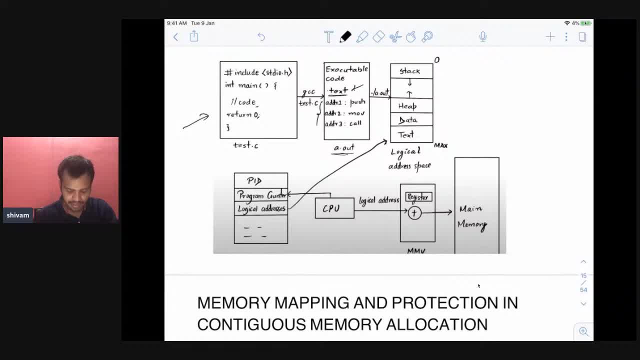 You have the text section and there will be instructions like at address one, address two, address three, right, And this is the executable file aout that is produced right Now. this will be divided into by the kernel itself. It will be divided into stack. 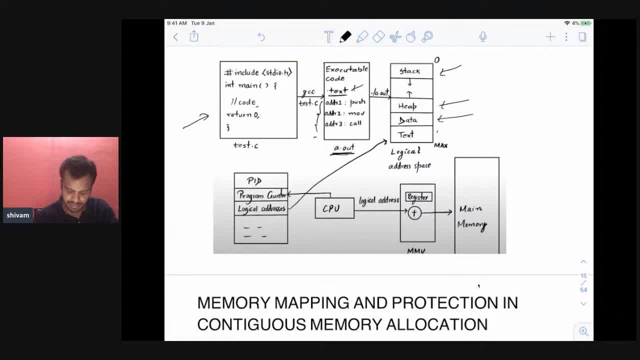 It will be divided into stack segment, heap segment, data segment, text segment, right, And this will be mostly from zero to max. This is mostly from. it can be any address like starting from, let's say, four to max or anything like that. 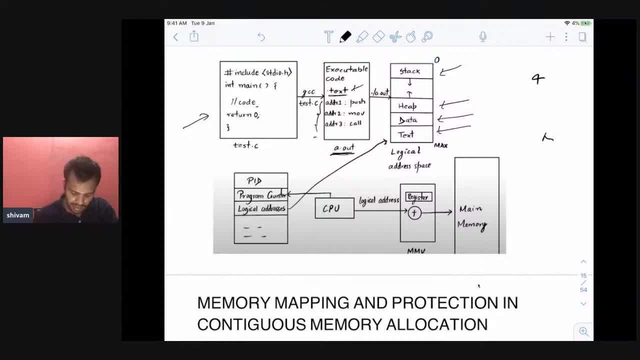 Most of the address will be in hexadecimal, not in decimal exactly, And this is and this is. these all are the logical address, right? And if you see this logical address, if you see your, I told you process control block, in that the logical address, this logical address will be stored like the mapping of 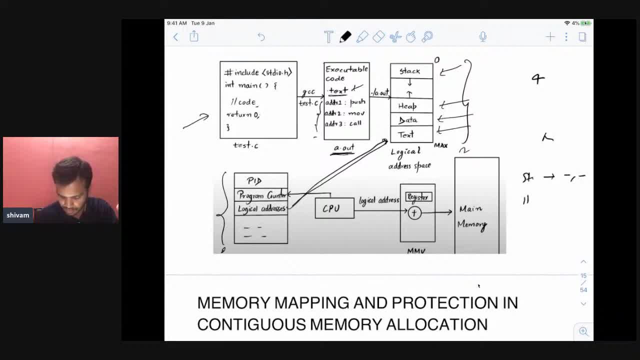 stack is from this to this, right Heap is from this to this. This all will be stored in the logical address. There is an attribute there that will be stored in that. Now, once they start running, once this program starts running, the CPU will see the value. 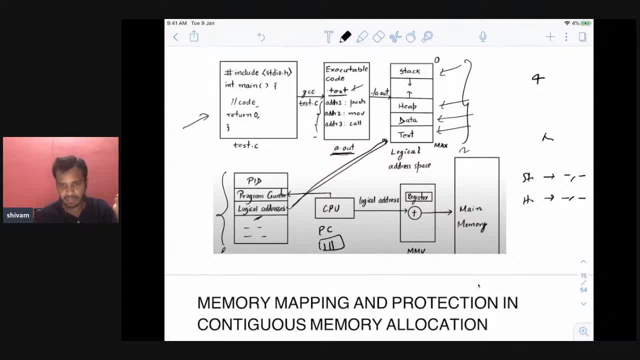 from program counter. what is the address here? And then there is a memory management unit which will convert this logical address into physical address, And then the instruction will be phased from the main memory. That's how it happens. This is a good example of that. 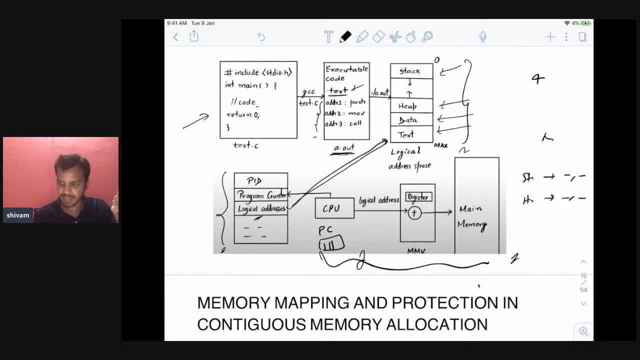 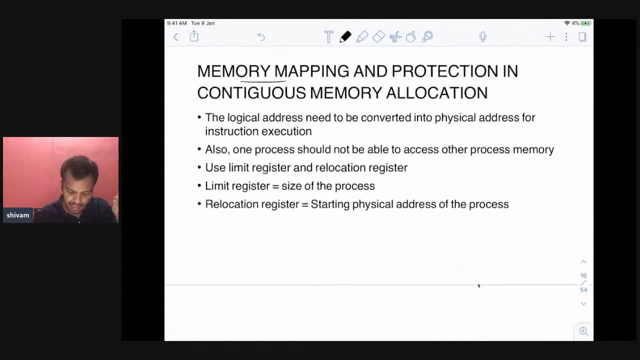 And I will explain more about this, like how this translation happens. Okay, now let's look at how you are going to do memory mapping and protection in continuous memory allocation. So we have already looked at the continuous memory allocation. Now how will you provide protection and mapping in that? 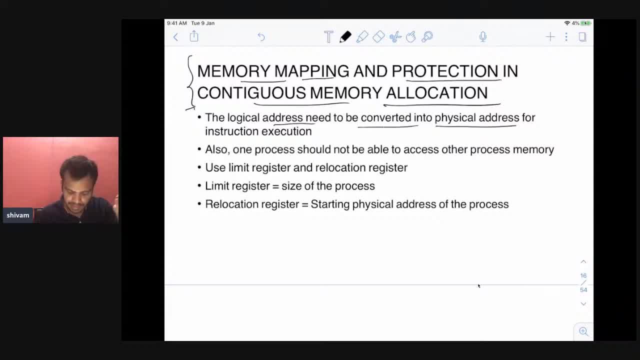 Now see, the logical address need to be converted into physical address for instruction execution, because in the physical address itself all the instructions are there, right? So you need to convert the logical to physical. Also, one process should not be able to access the other process memory. 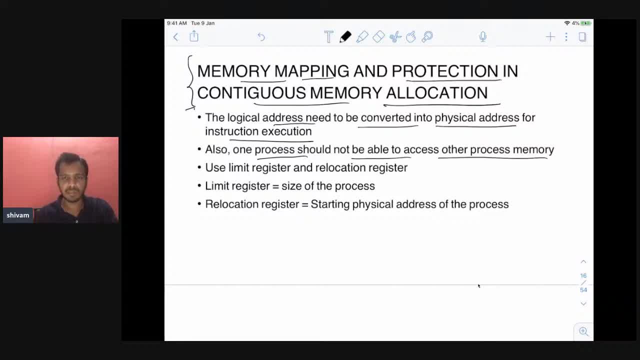 And it's bad right If one process is able to access another. normally we get segmentation fault in that right. So how will you do the memory mapping and protection in continuous memory? We will use two registers: one is limit register and one is relocation register. 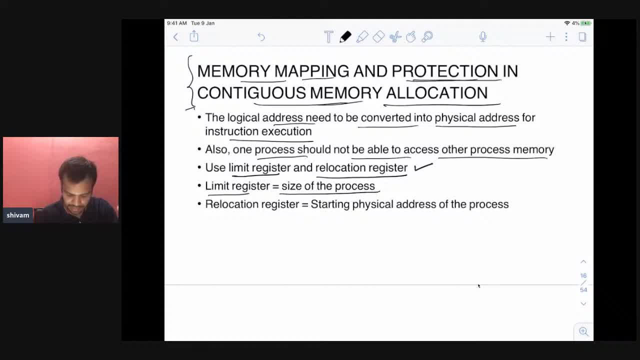 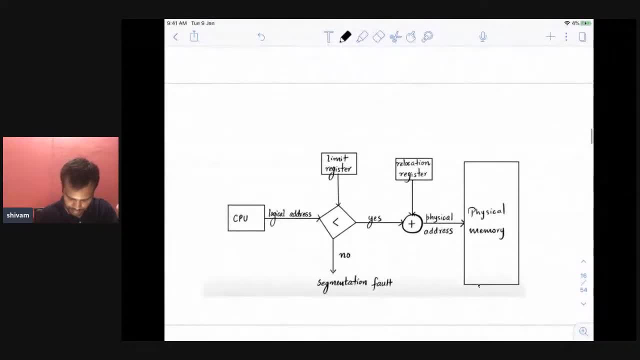 In the limit register we will basically store the size of the process- what is the size of the process- And in relocation register we will store the starting physical address of the process. Let's see this example. You will understand clearly, Okay. 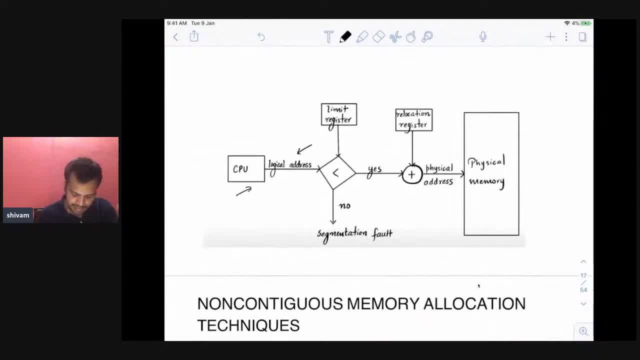 So CPU will see the logical address right. First it will check that this logical address is lesser than limit register or not. If it is not, that means this process is trying to maybe take the memory of some other process. right? In that case, do segmentation fault? 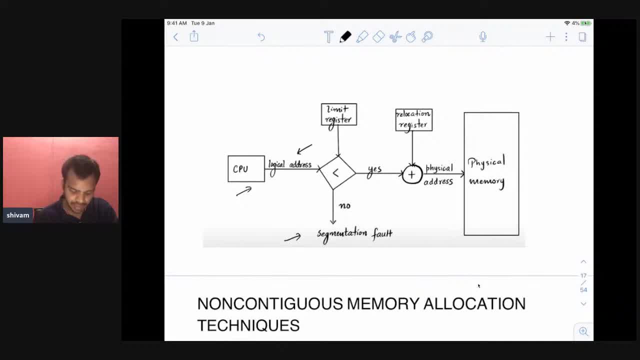 But let's say the logical address is lesser than limit register. What is limit register? It is the process size, right. So of course, logical address would always be lesser than this one, right Than the limit register. So if it is lesser than this, then proceed again. 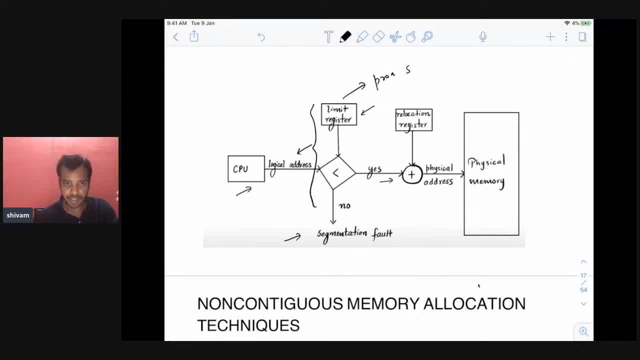 And so this is for protection part right Now, you're protecting this process from not accessing other process memory. After once this is done, you also need to do the mapping part right. So what you do? you take the base address of this process. 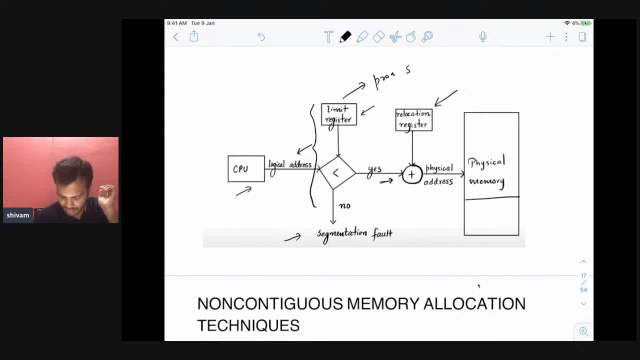 So there will be some base address. Let's say this is the base address, right? So let's say this is contiguous, right? Let's say this is 1000.. And this is a base address or relocation address. right From this, what you do, you will basically sum up this. I mean: add the relocation register. 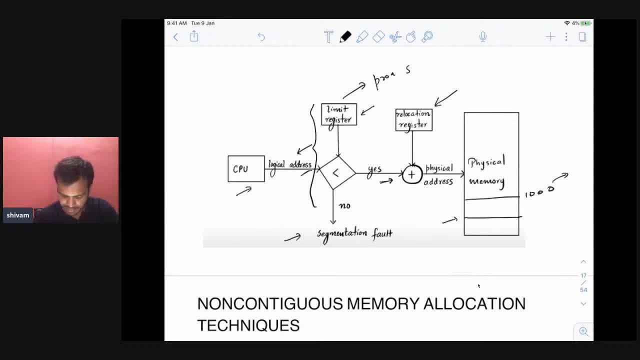 plus this one logical address. and you will go here And let's say this logical address is 5, right, And basically you want to fetch the fifth instruction for this process. So you will do 1000 plus 5.. And somewhere here the instruction will be there and you will fetch it. 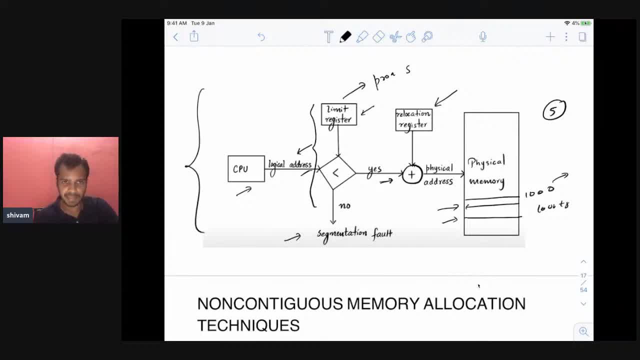 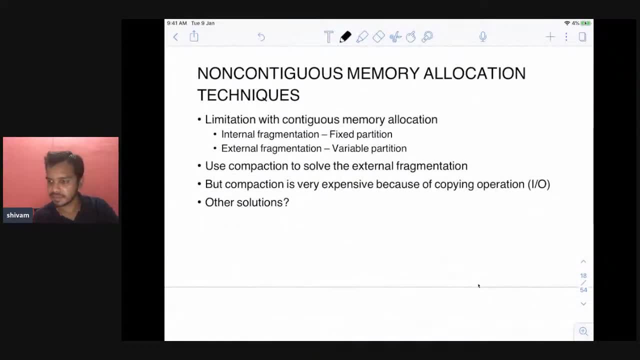 So this is for contiguous memory allocation, memory mapping and memory protection. Okay, contiguous is done. Now let's move on to non-contiguous memory allocation techniques. Okay, I will take some of the questions at the end, because this session can go for long. 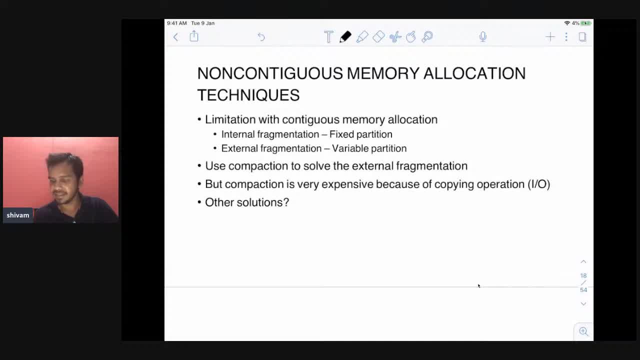 So let me just complete the session first and I will take all the questions at the end itself. Let's now look at non-contiguous memory allocation techniques. right, So there is a limitation with contiguous memory allocation. If you have seen right, you have two limitations. 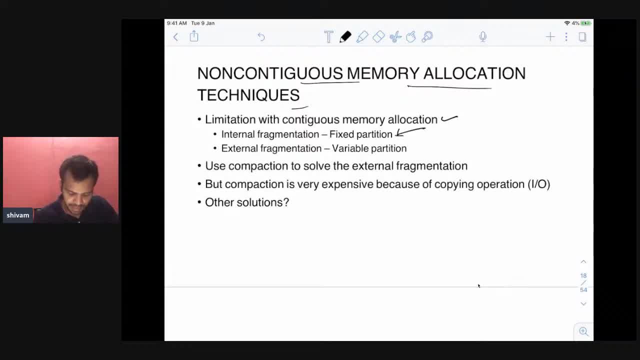 Let's say, if you are going for a fixed partition, you are suffering from the internal fragmentation. If you are trying to go for the variable partition, you are going to suffer from the external fragmentation. So there are some disadvantages, always with contiguous memory, right? 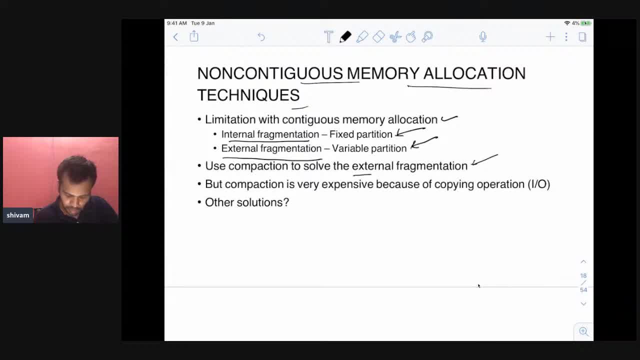 But there is one solution: You can use compaction right to solve the problem of external fragmentation. So what you do in compaction is, let's say- I'm just giving an example here- Let's say this is. let's say this: all is done right. 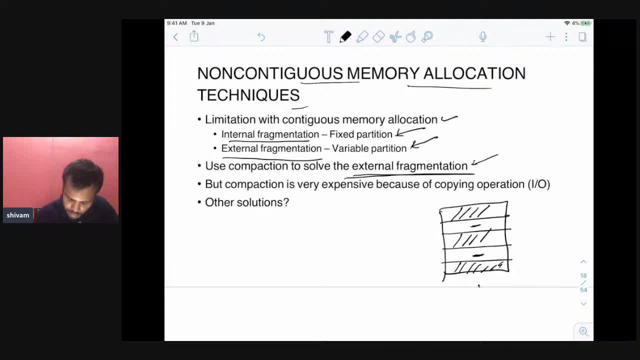 In compaction, what we'll do? this hole and this hole is free, right? You may try to compact this too, right? So what you will do is you will try to bring all these areas that are filled at the top and whichever the hole is there, you will try to bring it at the bottom. 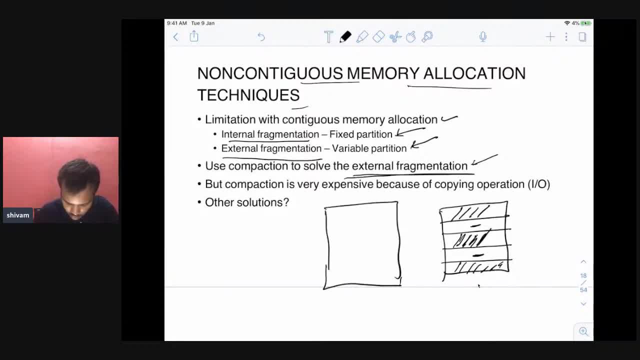 So the final right- Let's say the final rank will be after compaction- will be something like this: You will have these three occupied here And at last, these two holes will be free, right, Because basically, what you have done, you have moved this here. you have moved this. 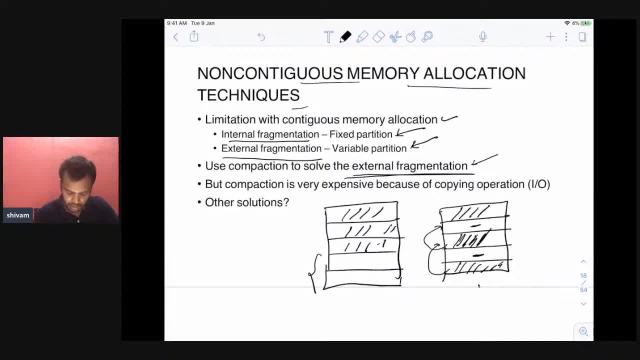 here kind of something, something like this: and these two are free here. Now you can add: now you do not have external fragmentation because you have done the. I mean, you have basically summed up this hole, whatever hole you have. 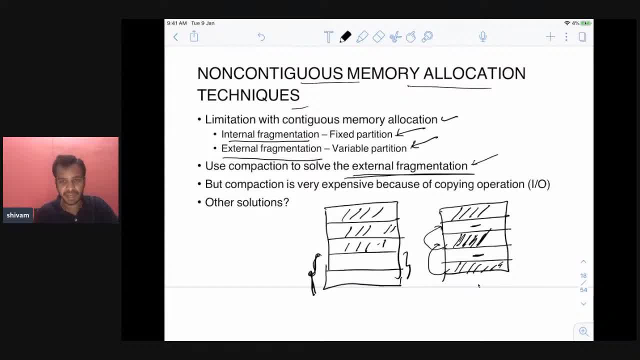 Now, you have contiguous memory here, right? But the issue with this is compaction. is that? see, you have to copy a lot here, right? This has to be copied here. This has to be copied here, And you know, copying is the IO operation, right? 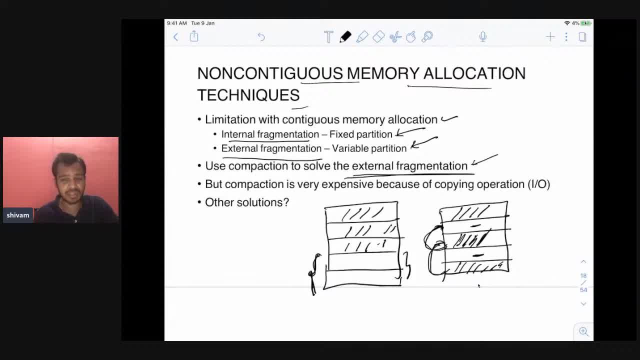 And you know how much expensive IO is. So this solution is not. I mean it is possible, but it's very difficult to implement And it's also very expensive if you want to do compaction to solve the problem of external fragmentation. 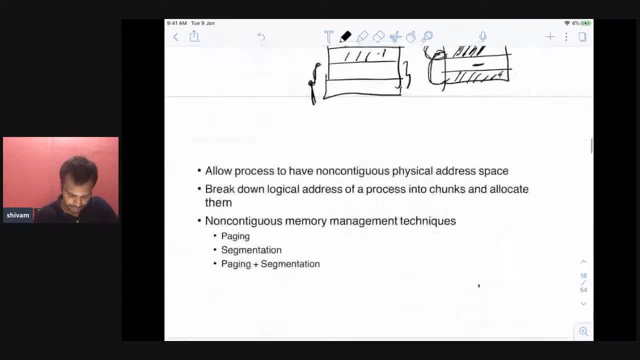 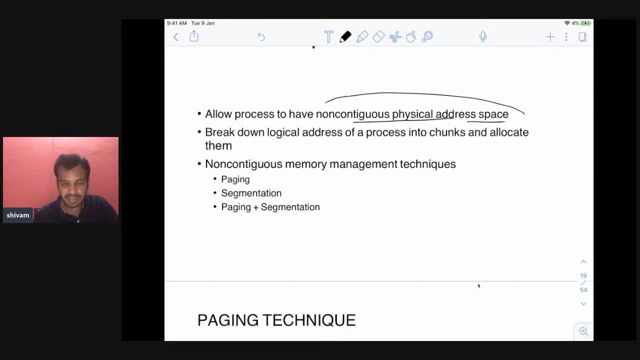 Now what other solutions do we have? Let's look at those. See now what? what if we allow the process to have a non-contiguous physical address space? So what if we allow this right? So initially we were thinking that 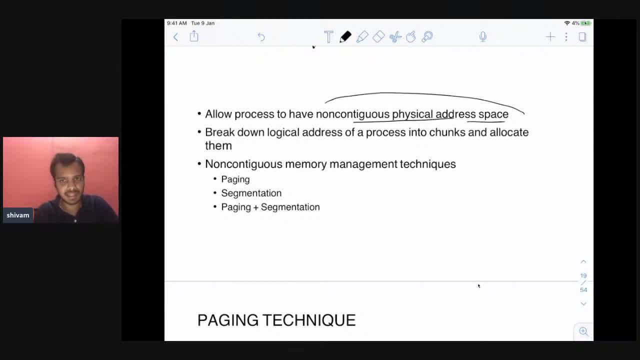 Also, all the process would be in contiguous memory block in the RAM. But what if we think different and think that, okay, process would like be like it can be like non-contiguous. right, This is what you can do. 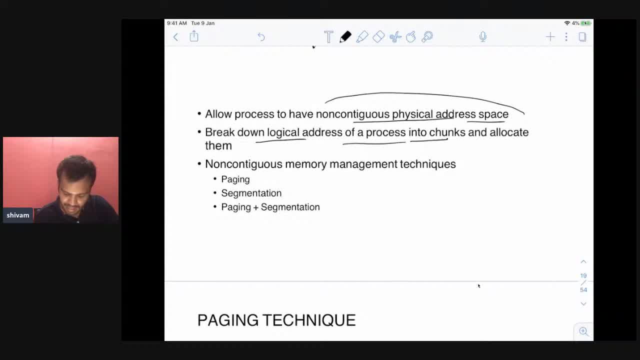 Break down logical address of the process into partitions and allocate them right. We will look at this, We'll understand more And like there are three important techniques here for non-contiguous memory management technique For contiguous, you know right Which one are: the fixed and the variable one, right? 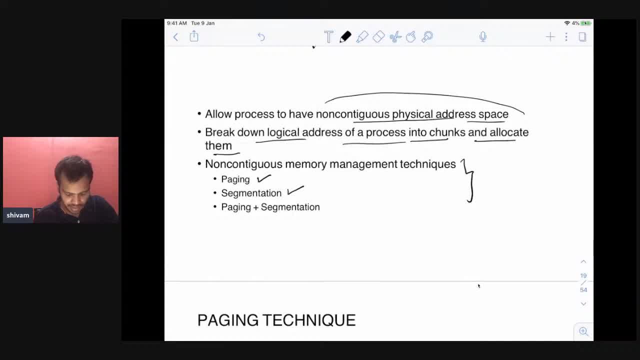 For non-contiguous like. one is the paging segmentation and one is the combination of paging and segmentation. Both are there, but I will only cover paging and segmentation in this video And if you want to like study paging and segmentation, combination of both of this, you can study. 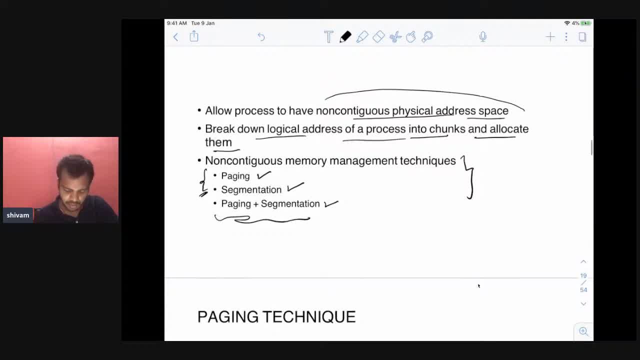 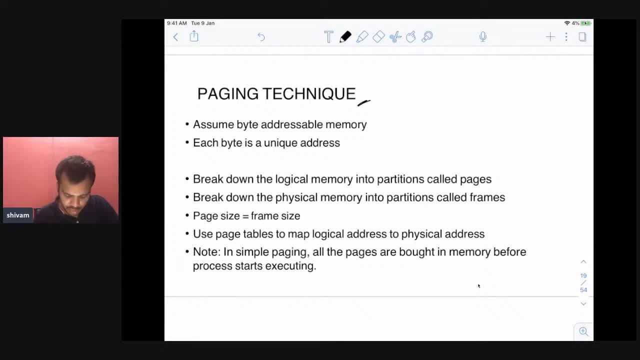 by yourself. but that is not in the book also And I am also not covering it here. Okay, Let's now move on to the paging technique. Now I told you right. We will assume that all the- I mean all the address are byte addressable in the RAM. 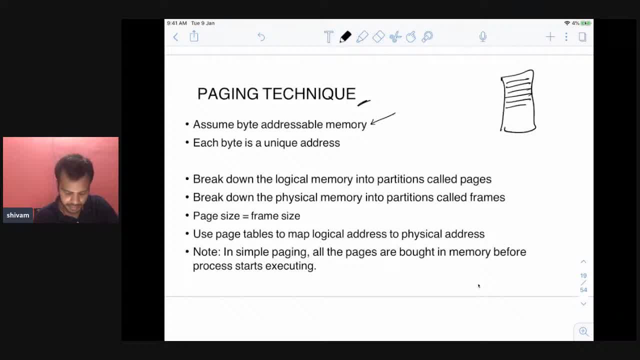 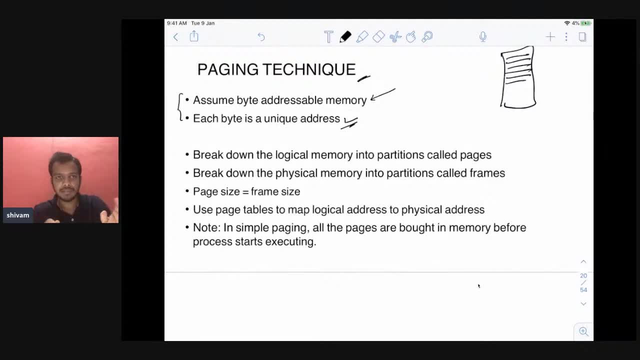 So every address is of one byte in the RAM And each byte is a unique address We will assume for all our examples. So the paging technique is very important. If you understand the paging technique, you will understand everything. You will understand virtual memory. 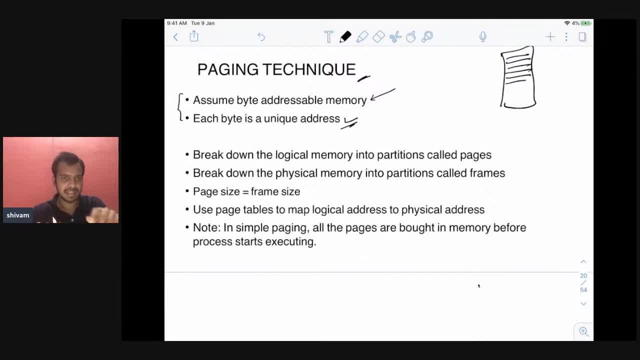 You will understand demand paging. You will understand everything If you understand the paging technique. this is the base of everything. But if you do not understand paging technique itself, you will not understand anything. So please focus on this part. This is very important. 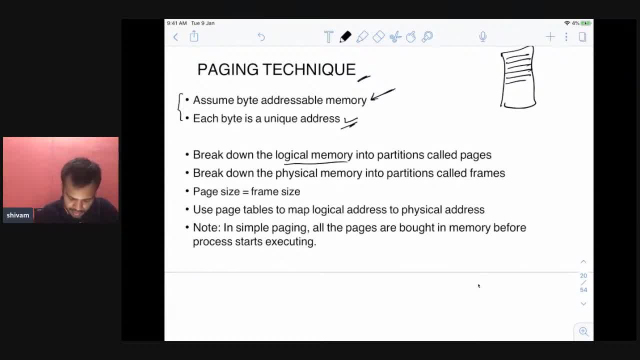 So in this what happens? you break down the logical memory units into partitions called pages- Very important to remember down the logical memory into partitions called pages and you have to break down the physical memory also into partitions called frames. this is also again important, see logical memory. 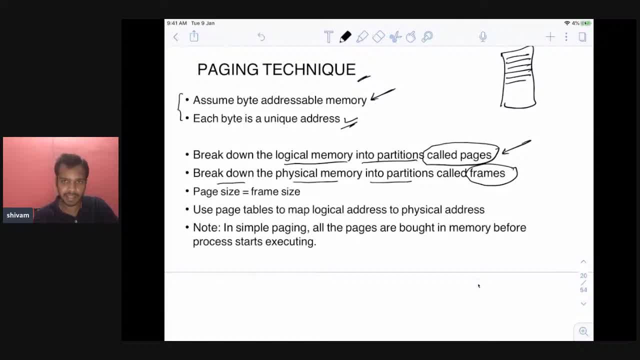 you are breaking down into, breaking down into pages, physical memory. you are breaking down into frames. the names are important here. also, when you are breaking down, the page size will always be equal to frame size. see what is frame. okay, i will show the example in the next slide. you will understand more. and these two sides are mostly equal in operating system. 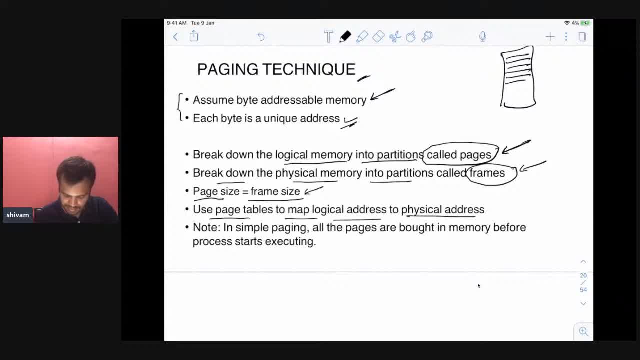 and also you will then use page table to map logical address to physical address, right? so logical address you need to map to the physical address. that will be done using the this page table. also, remember, in simple paging all the pages are bought in memory before process start executing. so i will say this is very important. see, in simple paging i am 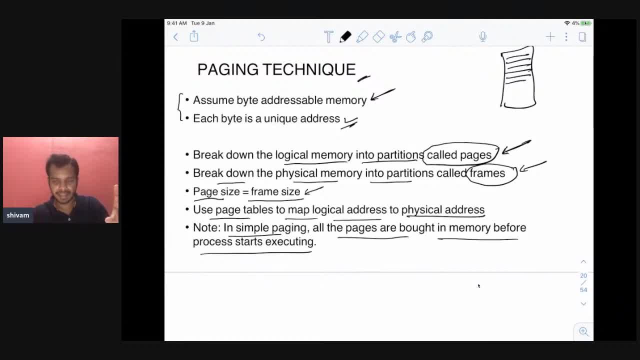 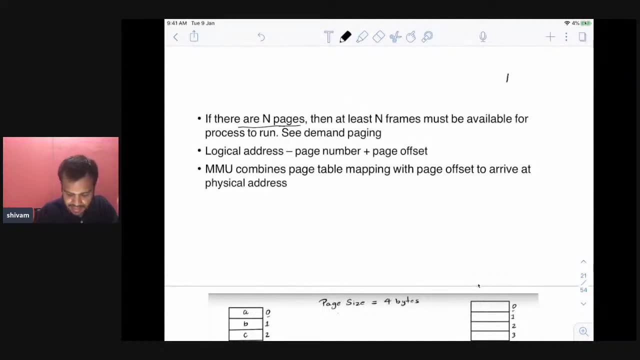 talking about a simple paging here. in simple paging, what happens? all the pages that are required by this process will be bought at once into the main memory. then only the execution will start. this point is very important. okay, also let that means: if there are n pages, let's say process has been divided into n. 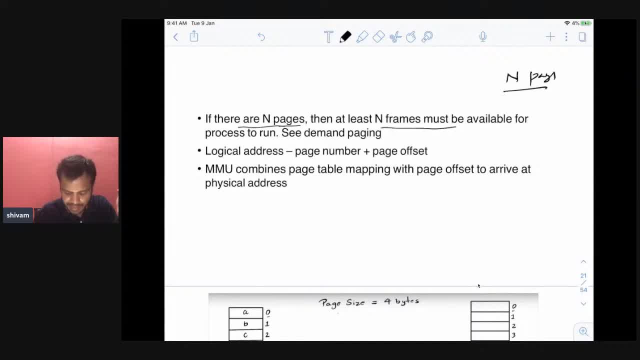 pages right. you at least need n frames right and frames must be free before this process can start. but we will see like how we can avoid this limitation when we go to demand paging. also, logical address in paging is a combination of page number plus page offset. so i will explain that. what are those? now? mmu combines page table mapping with page offset. 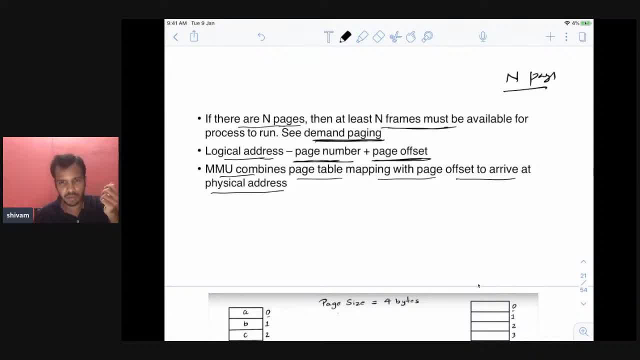 to arrive at the physical address. see, everything is possible in paging, right, so you can see. the process of paging is a combination of page number plus page offset. so i will explain this translation of logical address into physical address with the help of page offset, page number, page table is done by mmu, that is called memory management unit. this is very important. this is 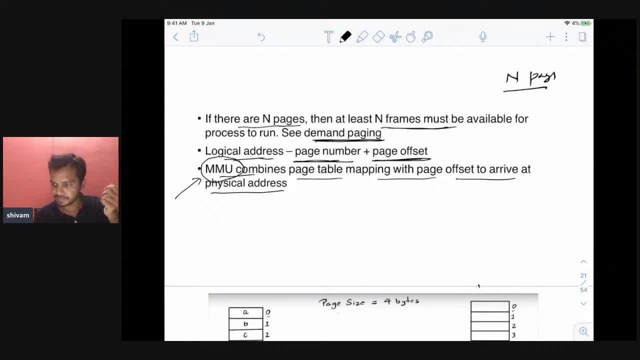 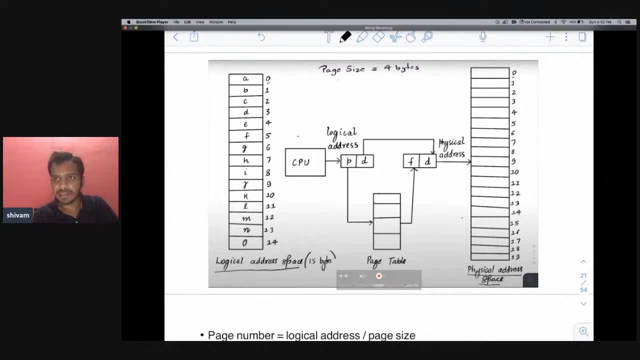 the hardware and this does all this, uh, everything. see, this example is very important. if you understand this example, you will understand everything in paging. let me see the battery of this: 42 percent, okay, so basically, you'll understand everything in paging if you understand this. see, this is your logical address, right? this is your logical address of size 15 bytes, right? 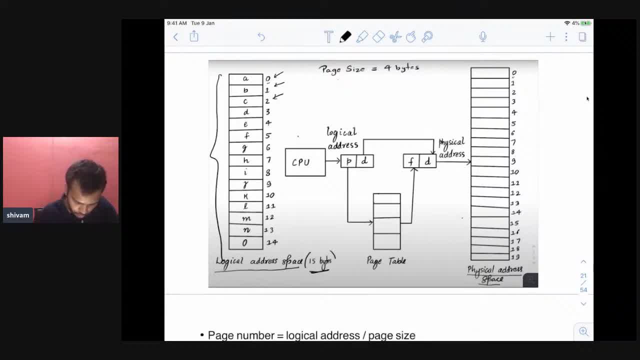 this is the zeroth byte. this is the first byte in your second byte till 14th byte. right, because i am starting from zero, right? this is your logical address that has been divided into 14.. this is your physical address ram that is of almost, if you see, of 20 bytes, from zeroth byte to 19th byte. 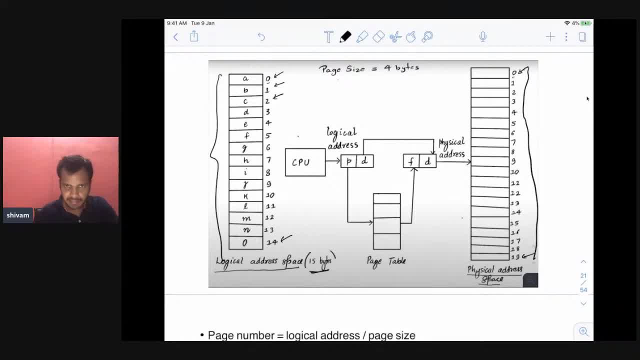 right now understand this. so cpu will basically get the logical address right. okay, let me do one thing more. see now, let me divide. first, divide this into pages and frames, right? so, as i told you, page size and frame size, both are required, and this page size normally is fixed. 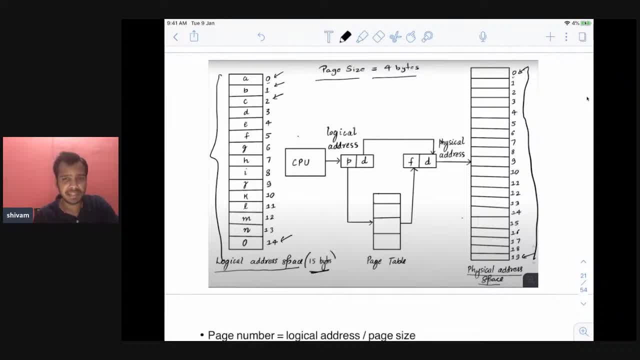 it will be four, by anything it will be, let's say so. typically system it's in kb, but in simple example i'm taking this is of four bytes, right? so let's divide this, uh, the logical memory, into pages of four bytes each, right? so this is the first four byte right now. next one: this is the next four bytes. 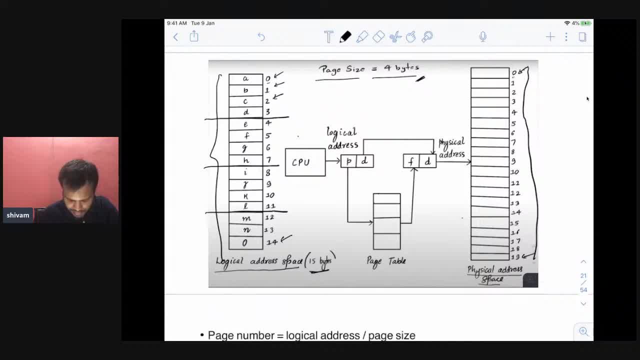 this is the next four byte and, of course, at last you have only three. so this will be called your first page. this will be called your first page. this will be called your second page. this will be called your third page. so, basically, you have divided logical memory into four pages. 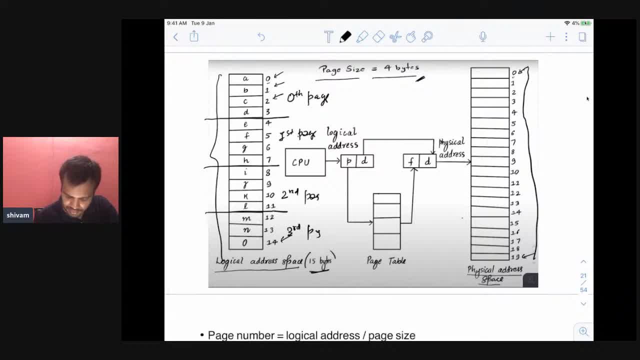 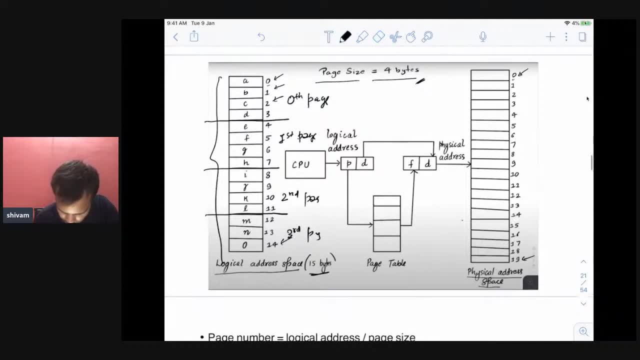 right, each of size, four bytes. now. similarly, you will divide this also- let me just clear this: you will divide this, this also into four, four bytes, right? so so here is your one division. so i think it will go something like this. so this is basically, this is your frame. 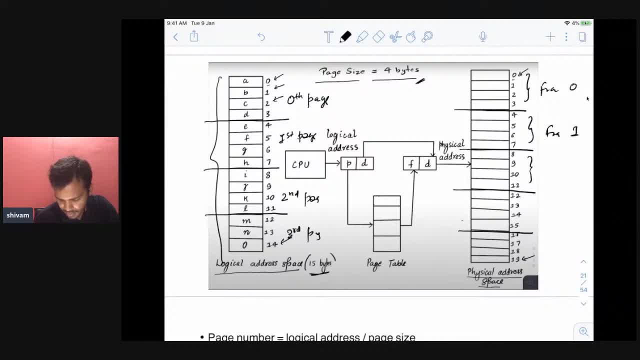 zero. frame one, frame two. so this is very important, understand this. frame three and frame four: right, these are the frames, these are your pages right now. what will happen? see, i told you. now, using the page table, you can map this right. let's say, i will explain that with an example. see now for every page. 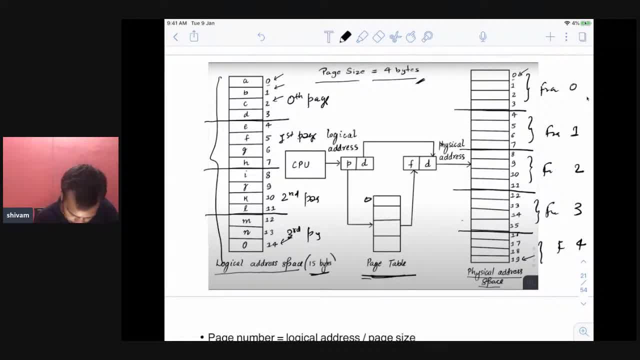 what will this pay table store? this page table? this is zero, this is one. this is type of array. this is your page number. basically this is a kind of mapping right, like you have array right. this is a kind of mapping right, so page number is mapped to frame number here in this page table. remember? 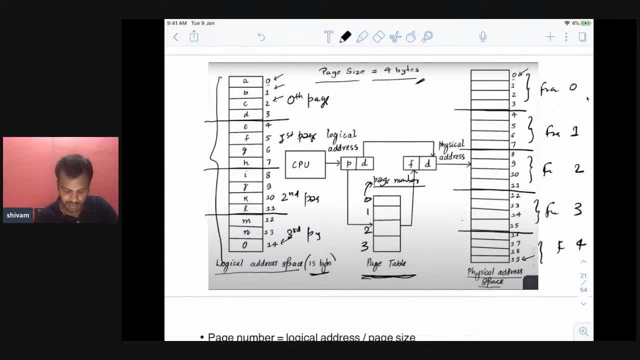 this: the mapping of page number to frame number is stored here. now, let's say it will be done by kernel itself. kernel will allocate, let's say first frame to, let's say this zeroth page, and i will take one onion, two and num, And let's say this is the first page, this first page, let's say the third frame. right, 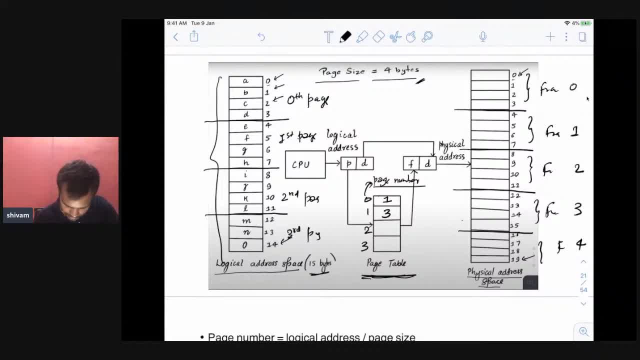 Now let me write this down here. So this is ABCD, right. So for this, which which frame is allocated for 0th page, the first page. so which frame is allocated, the first frame, the first frame is there. So basically, A, B, C, D will be here. this is page 0 is mapped here. 0th page is mapped. 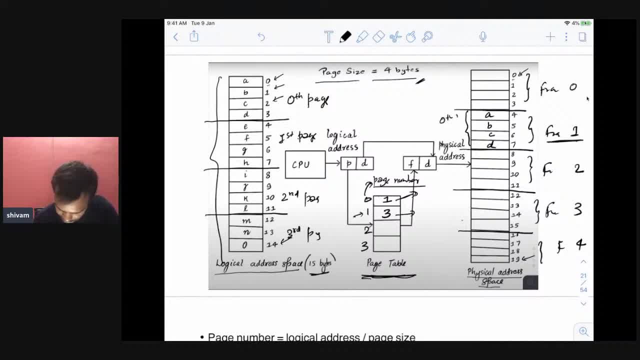 here. So the first page is mapped to the third frame. where is third frame? this is third frame. where is the first page? this is the first page. E, F, G, H will be here, right? So this is how it is. I will not fill all these numbers, but you can basically the kernel. 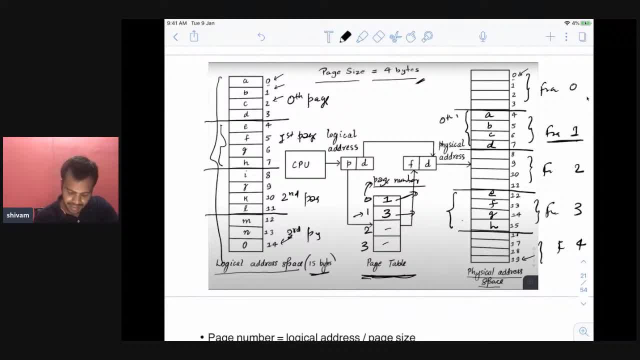 will fill this space table and the mapping will be done right Now. let's say, if you want to do some calculation, let's say now that if you logical address is, let's say, six, right, The logical address is six. Now you want to convert this into physical address, like how it will be done by MMU. 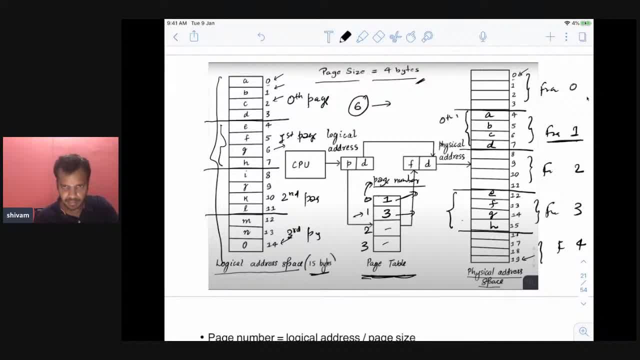 Let me explain that. See, first you need to convert this into page number and offset, right. So for six, basically for six. what is the page number? page number is one. What is the displacement page offset? So if we see, page offset is 012, right. 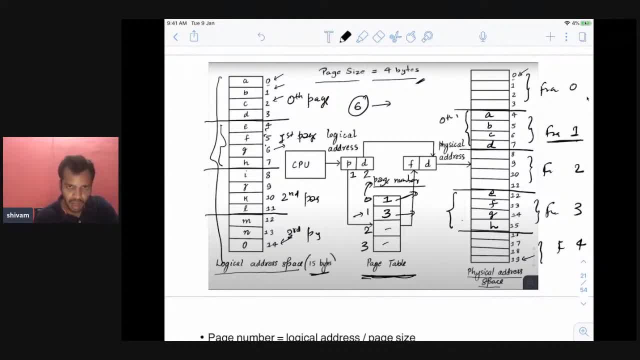 The offset is two. I mean offset means within this page, how much data is displaced right? It is displaced by two right. That's why two. Now for page number one. basically, the MMU will look for the page number one. what is? 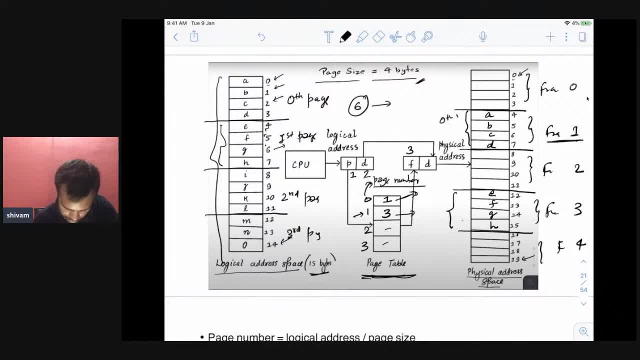 the frame number. The frame number is three. Let's put three here. And what is the offset here? Offset is two. right Now let's calculate the final address. So size of each one is, if you see, is three. so three into, I mean, size of each frame. 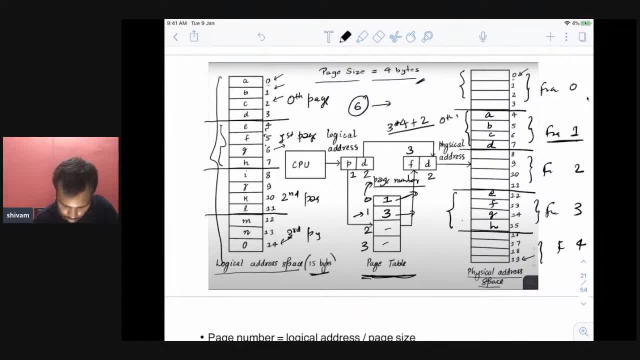 is four, right. Three into four plus two. if you do, it will be 14, right. So basically, this G, this 14 G, right here. you see, this G was stored here right In logical and we have mapped it here right to the 14th address, right. 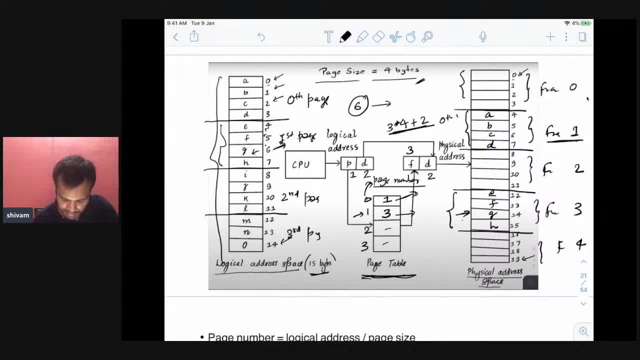 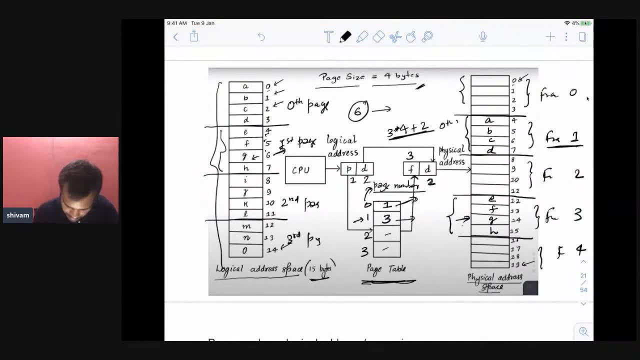 And how I did this. see, once I got the frame number and the displacement, what I did is: see I can cover here. there is no space there, but see, there are. I mean, we know that the frame number is three, right, 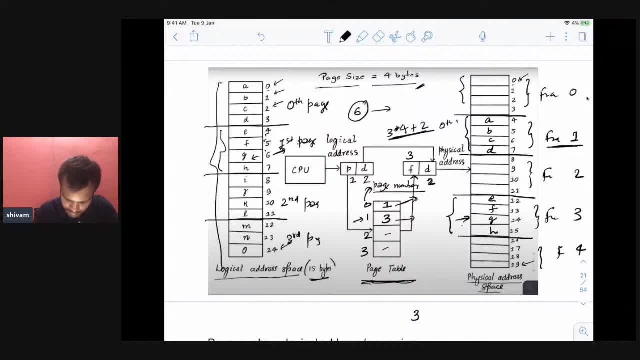 And we also know that each frame is of size four bytes. four bytes, So we multiply this by four. right Now we went to the 12th byte. We also know displacement is two, So we added two here and we arrived at the 14th byte. that is the mapping. 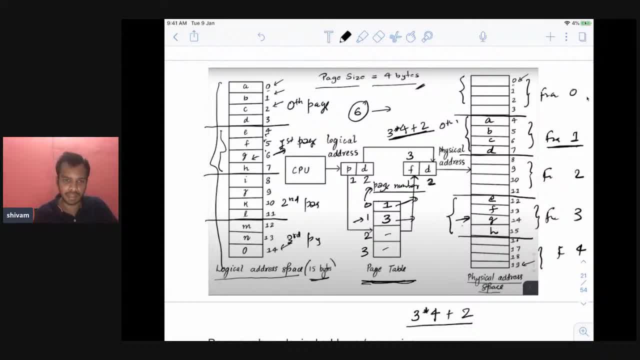 And I hope you would have understood this- like how this mapping happened. This is very important: how this mapping actually happens with the help of page table in which the this mapping is stored between page number and the frame number, and the MMU does all. 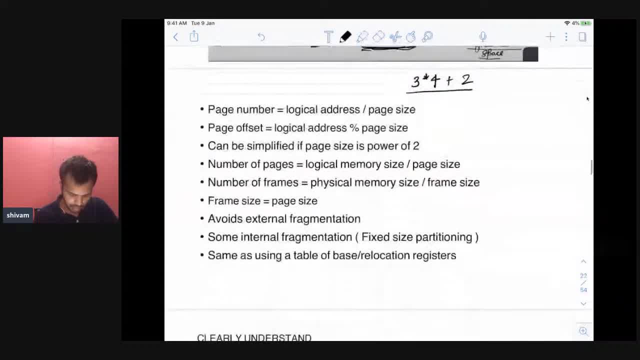 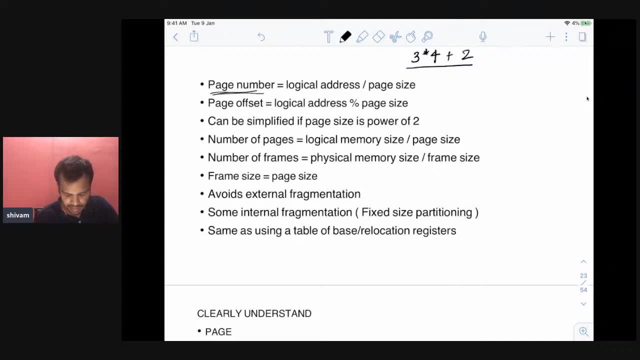 these calculations and arrives at the physical address. Okay, now let me just. okay, I've explained everything. Now let me explain that, if you want to know the formula for page number, its logical address by page size- In that the logical address was six, page size was four, right, 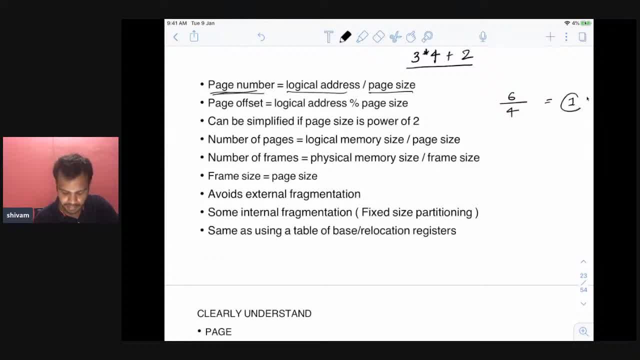 If you can have divided that, you would have got one. that was the page number And page offset is logical address. model of page size, that is six. models of four would have done. would have got two. that is the page offset. 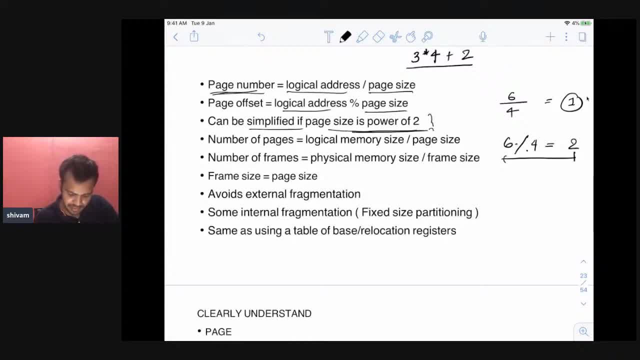 And this can also be simplified in page size, power of two. I will do this simplification for you after some time. Also, what is the number of pages? the number of pages is quite simple: logical memory, size by page size, right. 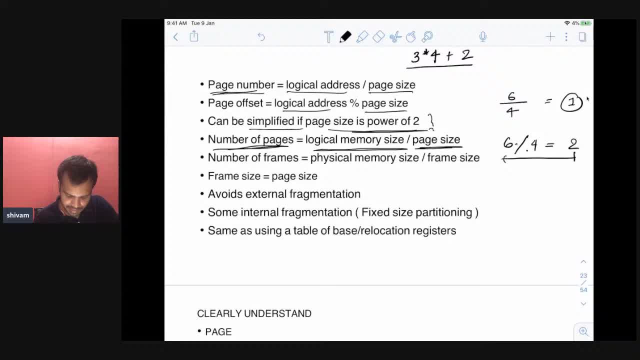 If you divide this two you will get the number of pages. So in the page size you will get the number of pages. Okay, So in the previous example, if you see in the previous example, you have like 15, 15. 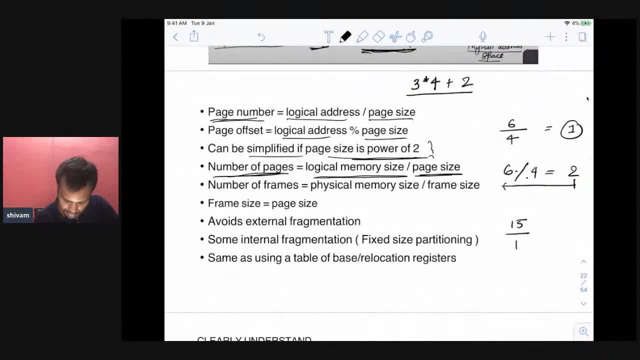 bytes, right. If you divide 15 by four, right, you will get around three point something, right. So you have to round this off to four. that is the number of pages. Number of frames is physical memory size by frame size. 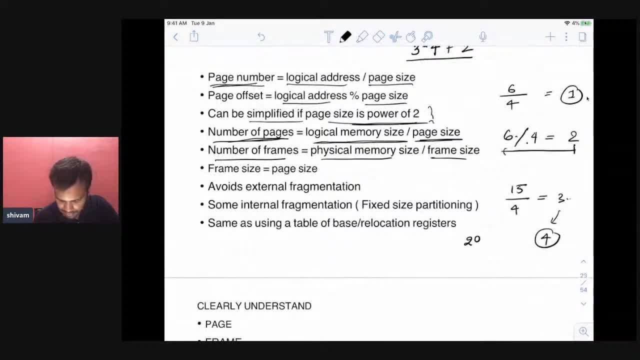 See, physical memory size here was around 20, now if you divide 20 by four you will get five. So we had five frames there, right? That is number of frames. Also, as I told you, in operating system page size is always equal to page size. 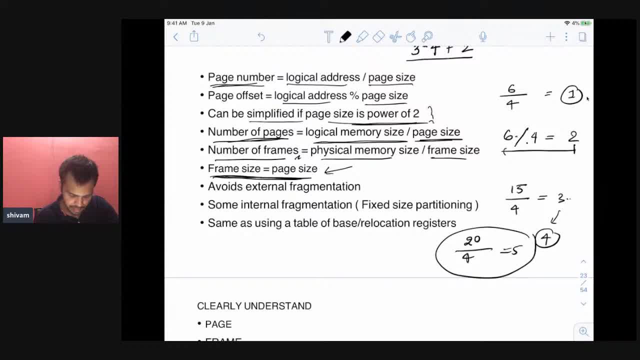 Okay, Okay, So the frame size is always equal to frame size is also a voice. external fragmentation, education here, right, Because? because it's not continuous, right, You can put it anywhere, right, It's not, there's no different fragmentation, but some, sorry, some internal fragmentation. 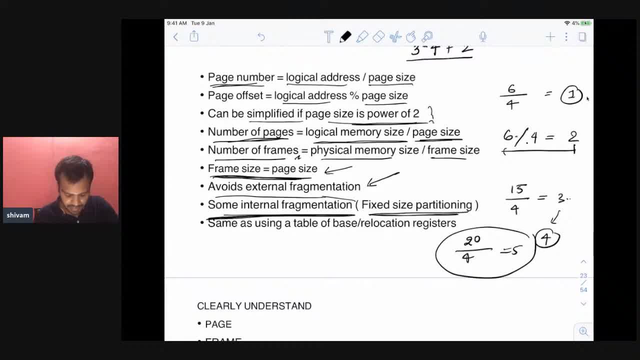 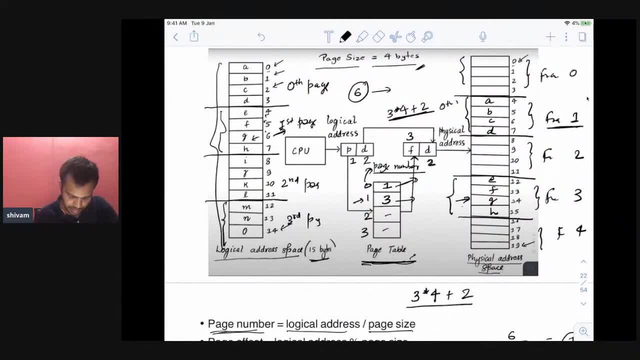 will always be there, because this is a kind of fixed partitioning, So internal fragmentation will be there. Take this example where you have only this three, but three bytes. right, These three bytes are there. If you're putting this, let's say somewhere into this frame. 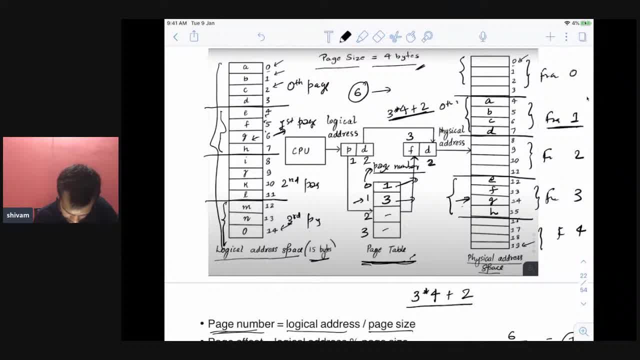 Let's see, this is the uh frame page number three for this. let's say, mapping was frame number two. so m and o, right, but now this one is empty itself. right, this is not occupied. this is internal fragmentation, right? so you cannot solve the internal fragmentation problem completely here, but you 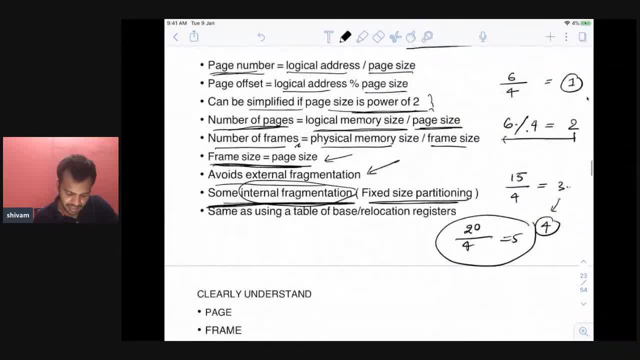 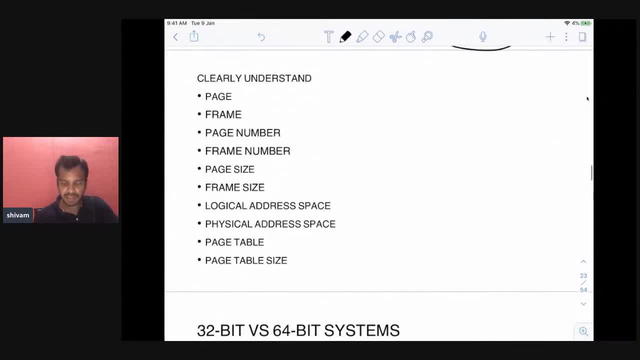 are trying to ready you. you have actually reduced it here, but external fragmentation is completely gone. some internal fragmentation is there, okay, and i will always tell you clearly understand these terms very important. if you do not understand these terms, do ask me in the comments or through message. do ask me all of this. this is very important, like what is page. 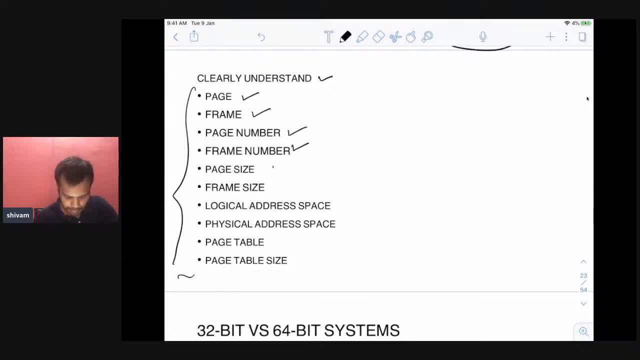 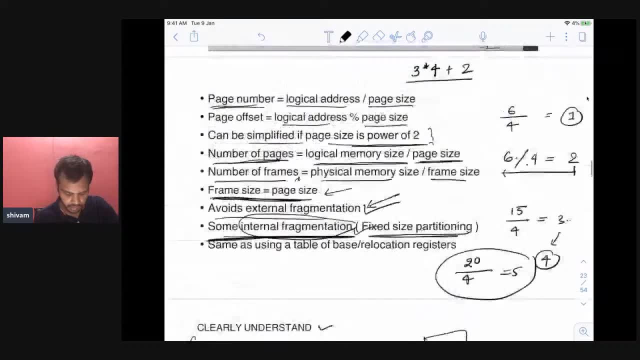 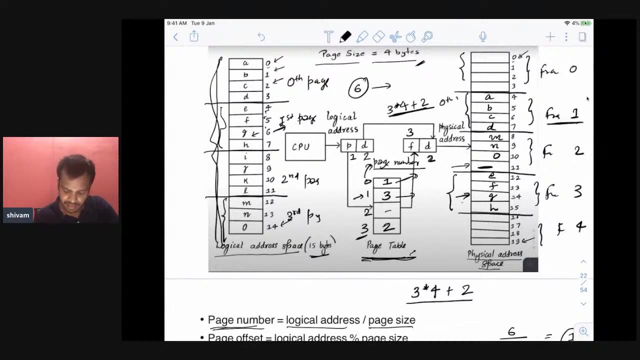 what is frame? what is page number? what is frame number? what is page size? what is frame size? what is logical address space? so the logical address space is this, the one i showed you here. right, this is logical address space. right, this is, and this is normally kept in the pcb. this is not actual address. this is actually the physical address frame, the ram. 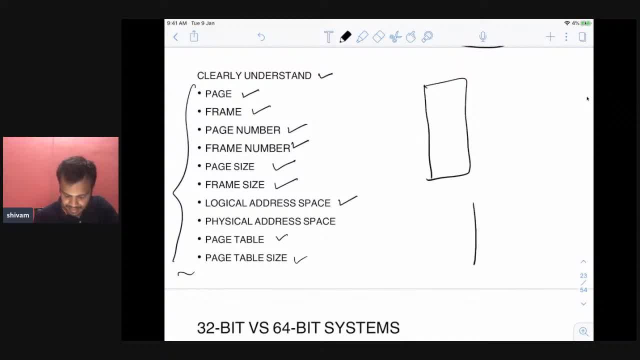 and then you have a page table. what is see? what is page table size? if somebody asks you what is page table size, see, this is a page table, right? let's say there are like zero, one, two, three, three pages. for each of these pages there will be a frame here, right? one, three, two, four. let's say 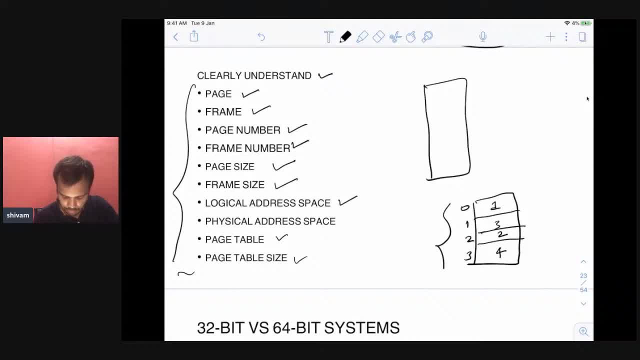 mapping here right now what is the page table size. so you have basically four entry, right, and there are four. see, this table will also occupy some size, right? that depends on the size, i mean how much bits this one is taking, right? so you have to see what is the frame number size and multiply this into that. you will get the page number. 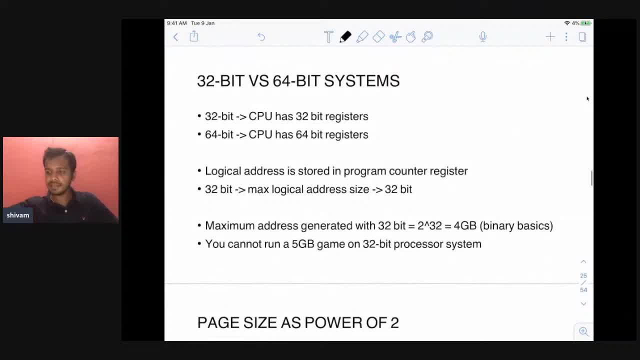 for page table size. okay, let me bring some more. now let's move on to 34 system, 34 bit by the 64 bit system. right, this is quite easy. most people do not understand this like body 64 bit and 64 bit. sorry, 32 bit and 64 bit system, but i will explain. 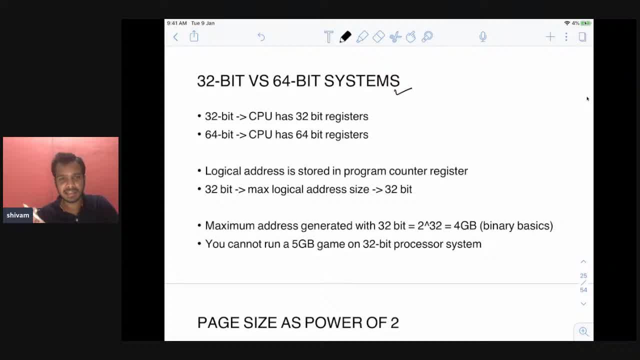 in a very simple way. understand that when somebody, when a system is 32 bit system, that means the cpu or cpu, all the registers are of size 32 bit. right, understand this. if your system is 64 bit, all the registers of the cpu are of size 64 bit. understand this. this is: if you understand this, now you'll 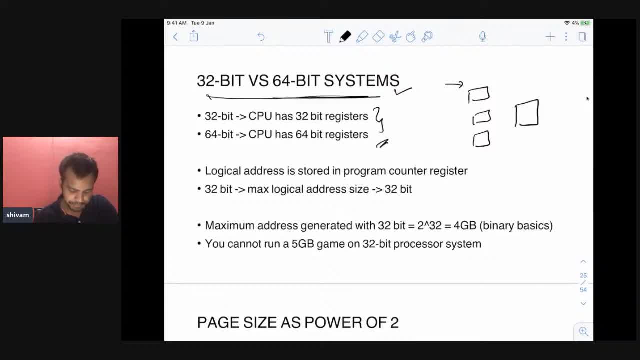 understand more about the systems. i mean, what does this actually mean? now you understand this, you, for every process, you have some logical address, right? this logical address is stored into program, which is again a register that is near to the cpu. now, let's say, if you have a 32 bit, 32 bit register, 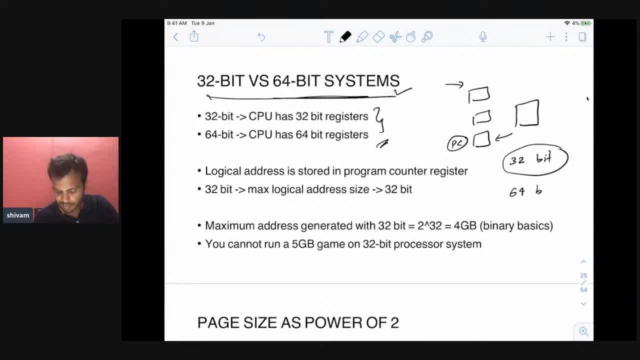 right and your logical address is 64 bit. but you cannot store this 64 bit into 32, 32 bit register, right? understand this right. so see, logical address is stored in a program counter register. so if you are 32 bit, the maximum logical, what is c? if you have 32 bit system, what is the maximum size of? 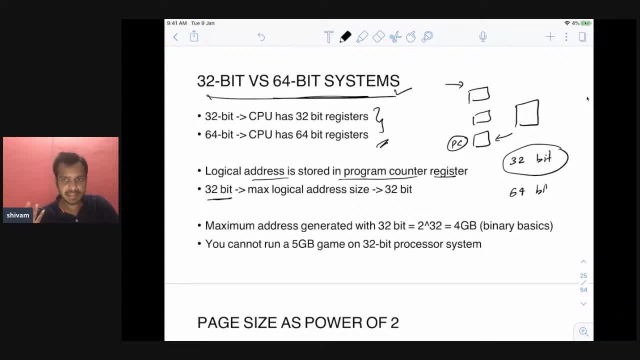 your logical address space, right? what is the maximum size? it's 32 bit, right. it cannot take more than 32 bit. so logical address cannot be more than 32 bit if the system registers are itself of 32 bit, right, because this logical address need to be stored in some register itself. 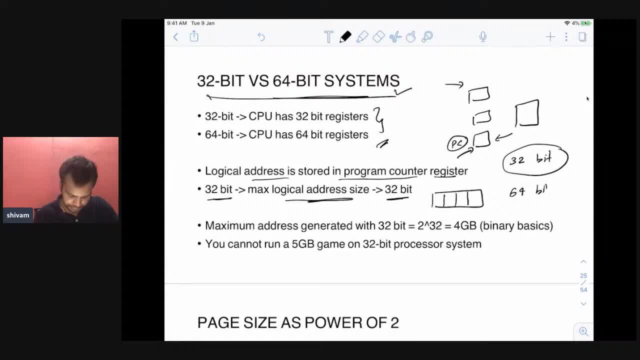 and if the register size is not 32 bit, then you can store it. so what is the maximum address generated with the 32 bit? see, this is basic binary, right? if you have four, three bit, how many numbers you can? uh, how many numbers, different numbers, you can produce with three bit? right, you know two power. 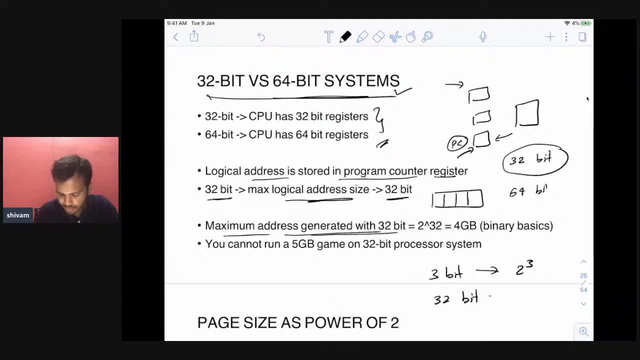 similarly for 32 bit. how much, uh, how many address will be unique address will be there two power 32, right? this is basically equal to 4gb. i mean this is binary. you convert it to about 32 bytes, it will be 4gb. now you understand that you cannot run a 5gb game on a 32-bit processor system. 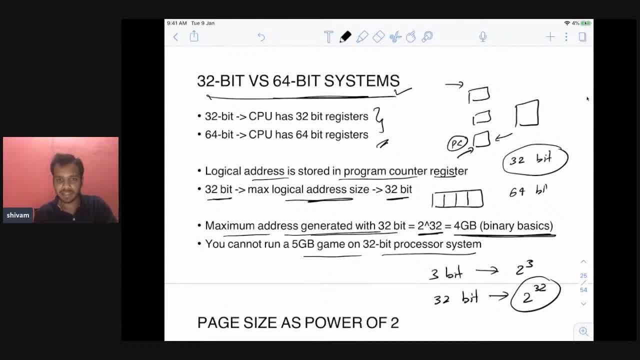 why? because 5gb game is more than 32-bit right logical address in 5gb game. if your process size of process is more than 5gb, then your logical address size will be more than 32 bit. let's say it is 34 bit. let's say, but your system registers are offside 32 bit itself. then how can? 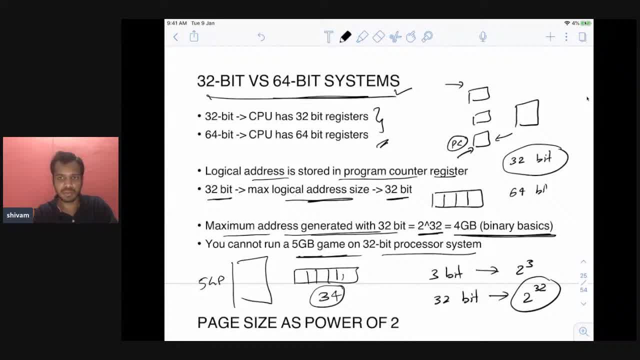 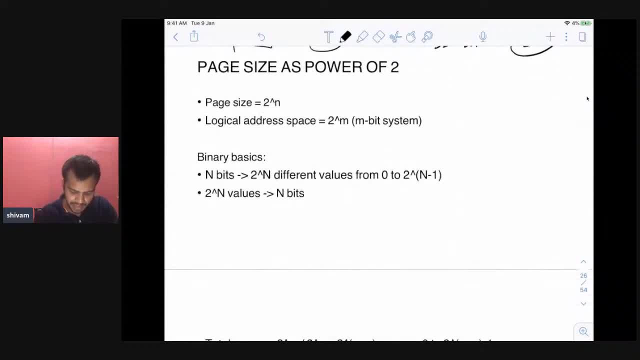 you store that 34-bit logical address into 32-bit register. that's the tough part here, okay, uh, okay, let me simplify also page size as a power of two, right? i'm simplifying this, let's say, because i told you right. the calculation was like: if you divide logical address, i mean division by. 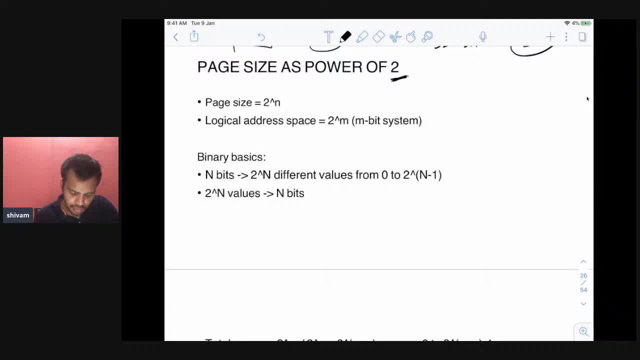 page size. you get that right. that is quite complex. it's better to do like: keep the page size as a power of two. that's what the kernel also keeps it. kernel will always keep the page size as a power of two for simplifying the calculation- and this binary calculation becomes very fast for the cpu. 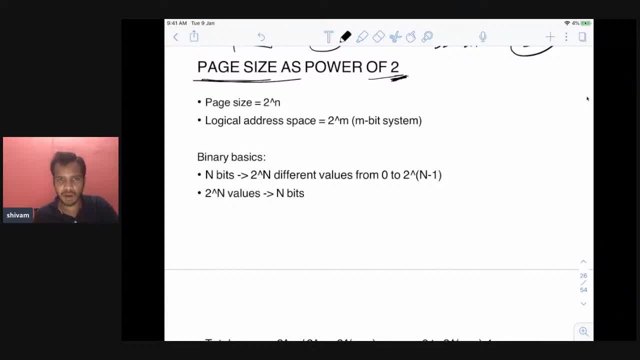 that's why the page size will be a power of two. and see, logical address is always a power of two, right, because either the system is 32 bit or 64 bit, right, it's always a power of two. see, now, assume that the page size is 2, power n and logical address space is power to power m, the, i mean the. 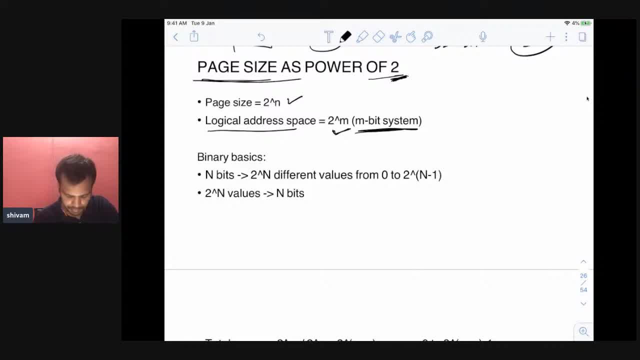 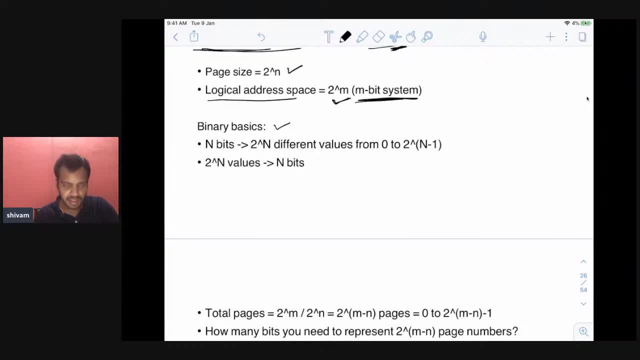 system is m bit system. that means logical address. space is of 2 power m. Now, if you remember the binary basics, if you have n bits, with the help of n bits you can represent two power and different values from zero to two power: n minus one. 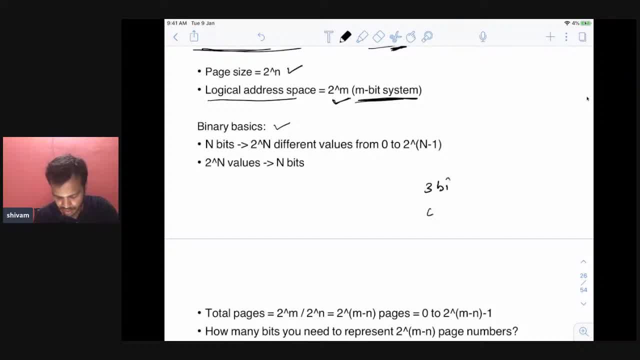 right. And if you have three bits right, you can represent value from zero to seven. these are eight values, right. But take the converse also: if we have two power n values and if you have eight values, how many bits you require? you require three bits, log n. if you do log of two, eight you. 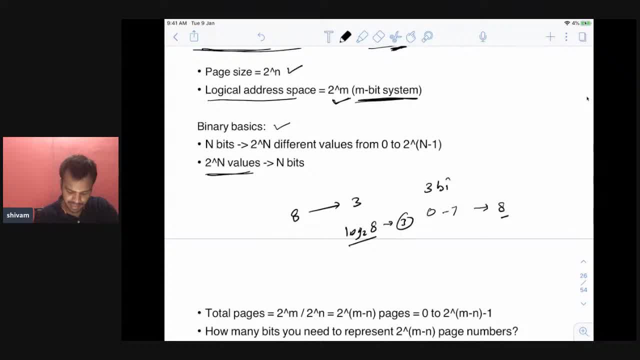 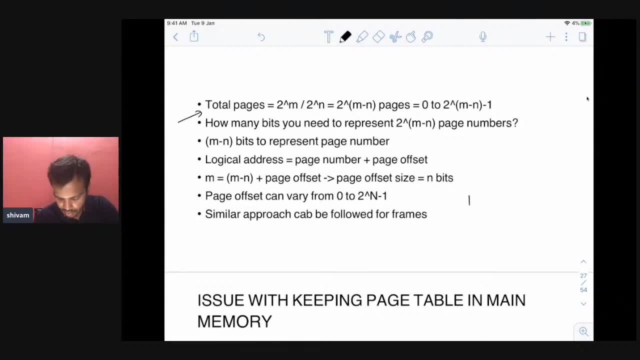 will get three bits right. So that's the answer And that's the basics of binary that we will use here. See now what is the total pages? total pages is equal to. I told you, total pages is equal to logical, total, logical address. I gave you the formula right, divided by page size. 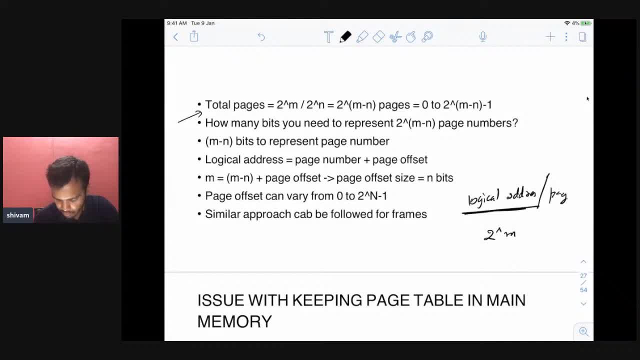 Now, why a logical address here? I took it to get to power m. what is the page size? that is two power n. Now you, what you get is total pages is equal to two power m minus n pages, the total number of pages that you get here, right? 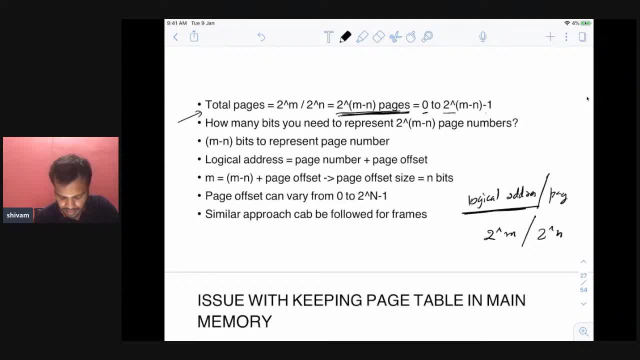 And the pages will start from zero. It will go to two power m minus n minus one. right Now, how many bits you need to represent two power m minus n pages? see basics of binary. Now you have pages starting from zero, going to two power m minus n minus one. 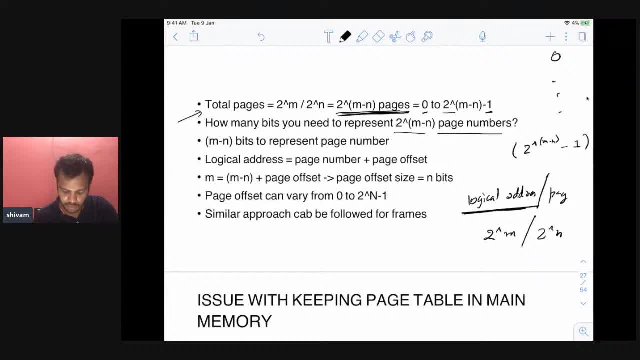 Now how many bits you need to represent this. all these pages. of course you will do the log of this. you require m minus n base to represent the page number. So if you want to store the page number, see page number. page number is integer, right. 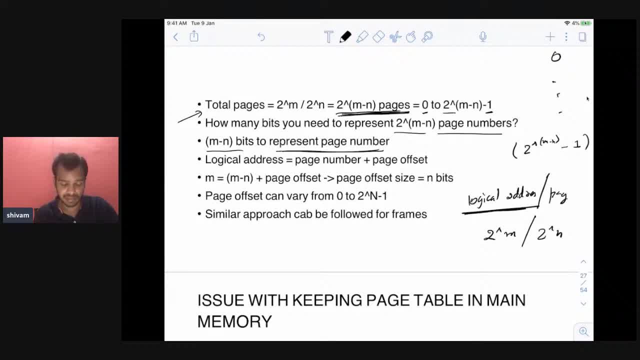 It will take some bytes. It will take some bytes or bits, right? So you need m minus n bits to represent the page number and understand this. Now, logical address, we know, is a combination of page number and page offset, as we saw there. 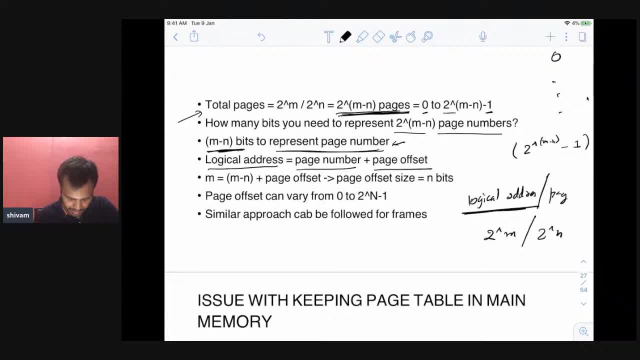 right in that. But we know that. see, I have put this formula here. logical address is of size m. page number we already know is of size m minus n. I have put it here. We have to derive this page offset. how many bits are required for page offset? 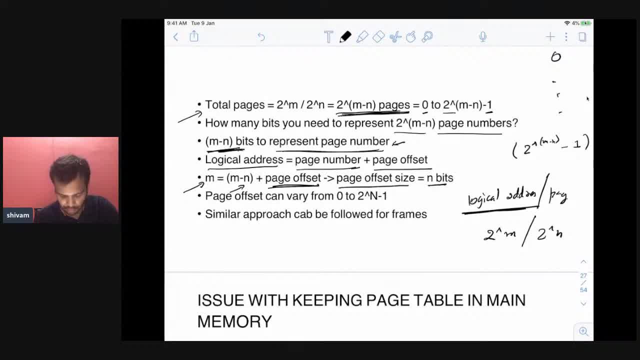 So page offset will be n bits from this formula, right, If you take this here, do the bit offset right, So you will get n bits. So you will get n bits from this formula. So in basic evaluation you can get page offset size equal to n bits. 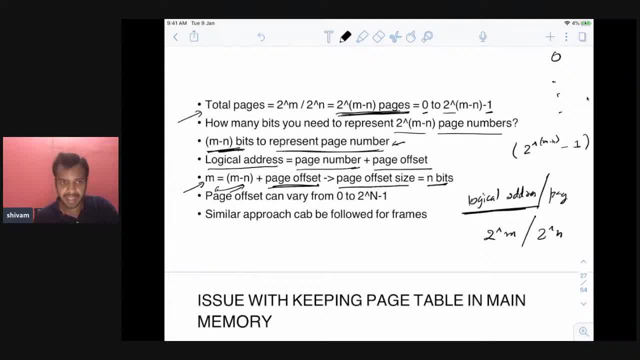 So you need n bits to store the page offset. You require m minus n bits to represent the page number And also page offset see. another way you can tell that you require n bits to store the page offset is see. page offset can vary from you know, from 0 to 2 power n minus. 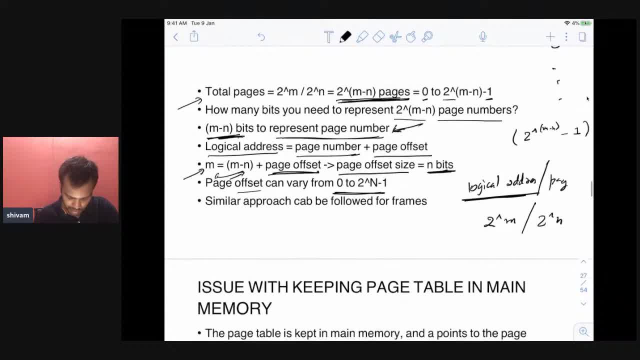 1, right, Because I mean: see what is page offset. if you remember page offset within a page right, Within a page itself, you have the page offset right and it can vary from zero to page size itself. right, you cannot go beyond this right. 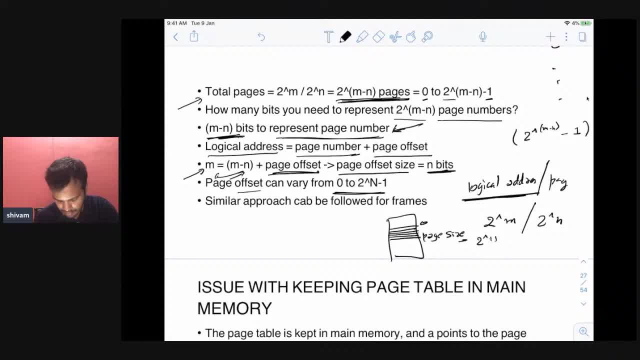 so zero, your only page size. here we have two, power and right. so of course, again, convert this into log. take the log of this. you will get n bits itself right. so both way you can calculate it, and also i am not going to calculate. do this calculation for number of frames and 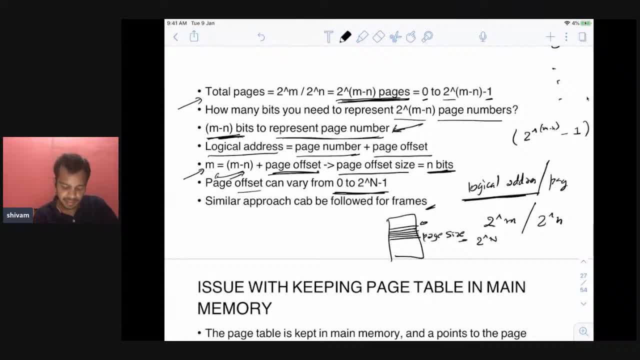 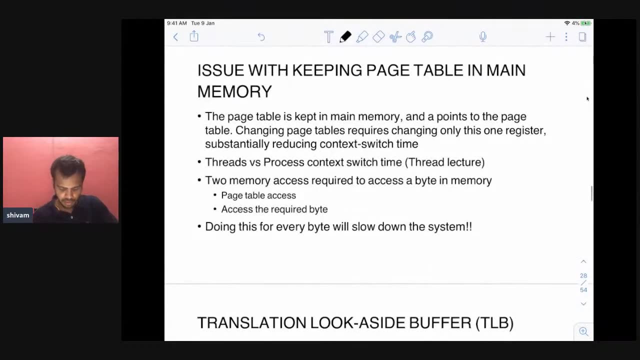 what is the size for frame and storing the frame and everything. see, follow the same approach and do the calculation for, let's say, the main memory size is of power 2, power x. right, do this same calculation for frame. also same thing. you can apply it. okay, now let's go to issue with keeping. 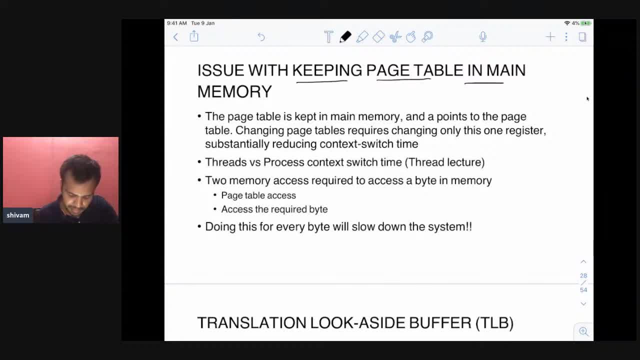 page table in main memory. right, there are some issues with keeping the page table in main memory. the page table is kept in main memory, see what is the issue with. i will tell you what is the issue, see, i told you that the fastest one is the register. 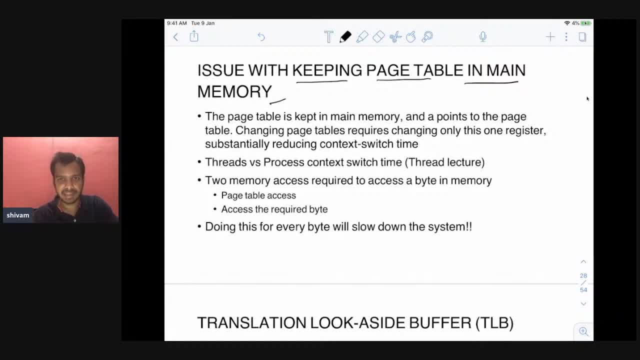 then the cache and then the main memory. right, main memory also takes some time for the cpu. i mean to face that instruction. let me connect the charger with my discharge. i'm sure that nobody is getting bored. i mean, uh, i will answer the questions at the last time. 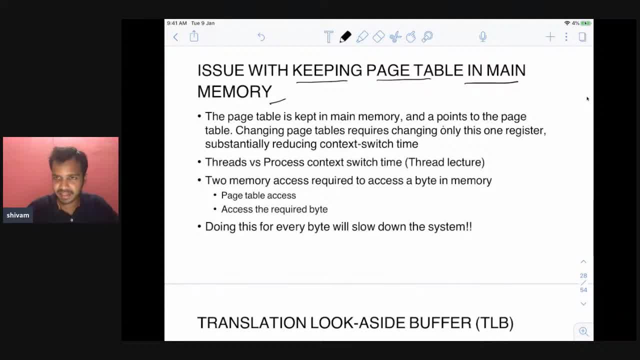 because it's still in this session. it's almost one hour now, so, yeah, and be there with me. i mean, i am. i hope that you are not getting bored in this session, and we are in this session because i want it to cover all the memory management in one session itself. okay, now the issue with keeping 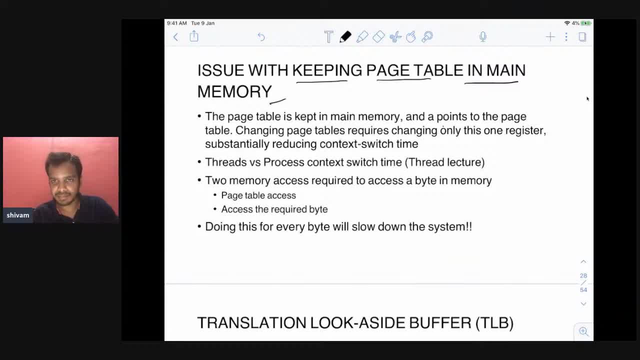 page table in memory. is that? see, i told you maybe it's not the fastest memory for cpu, right, this is the third fastest. so it takes some time for the cpu to see if you keep the page table in here in the main memory. for every logical address you need to go to this uh main memory, find the mapping. 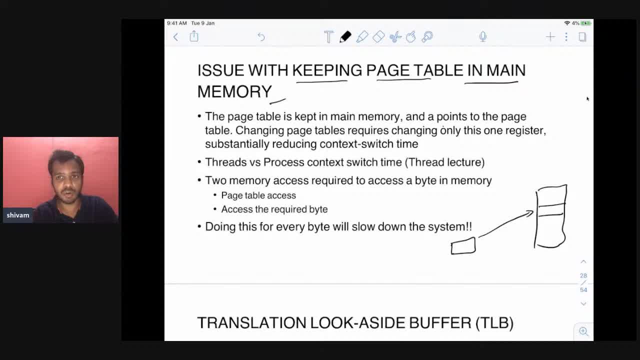 again come back. so you have to do for every logical address- and you know that how many logical address can be there? i mean there can be, i mean logical understanding can be in the main map. lot of, lot in numbers, right? so you do not want to go every time, every time in the ram, which is not 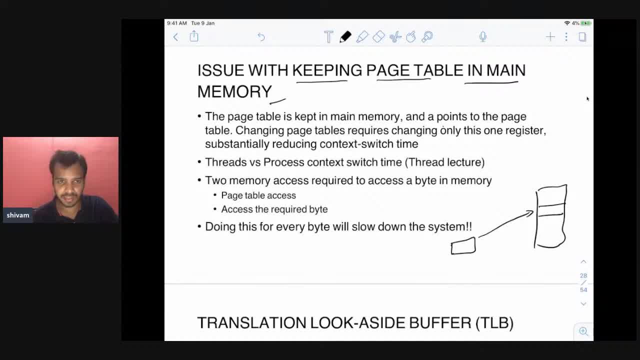 very fast, i mean compared to registers and cache. right, you don't want to hit that and okay page and point to the page table. changing page table requires changing only this one register substantially. contact. i have discussed this in the trade lecture when i was covering the trade one, that basically you have to store the base register of the page table in one of the 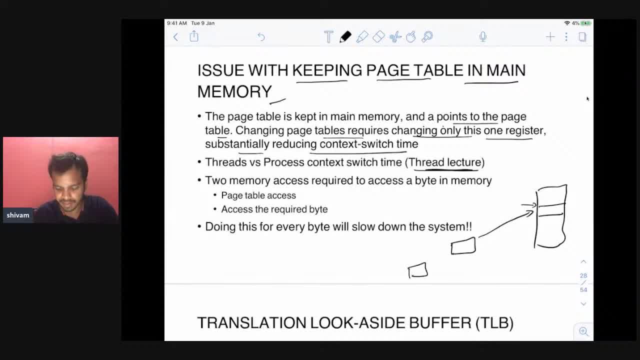 register here near the cpu and when you are changing the process, you just need to change this base address of the process table. but with if you are changing, moving from one trade to another within the same process, this will not change. that's why context switch time for between. 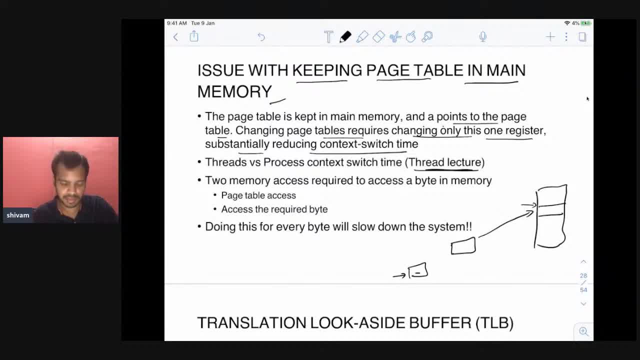 two threads is later than context switch time between two process and in this case, what happens? if the process, i mean if the page table, is kept in the main memory, then two access is required to two access is required to every type. see, if you are keeping the page table here, you require two. 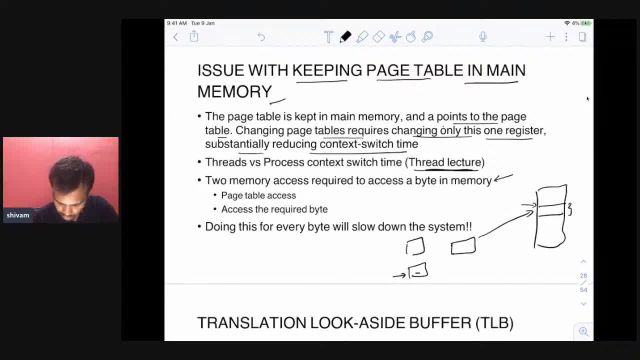 access for every. you are keeping the page table here. you require two access for every access for every instruction. why see? cpu will see the logical address here. first it needs to convert this logical address into physical address. this is the first access right now. second access will be once. 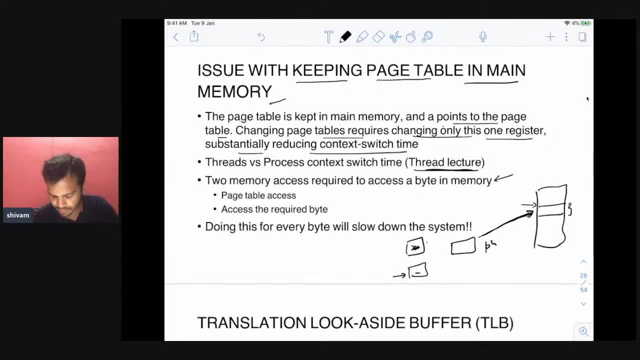 it has got the physical address, it again needs to face the data from this. what is the date instruction here? that is the second access. so you require two access for every instruction and if you are doing it for every byte, you understand how much the system can become right. you are hitting ram for 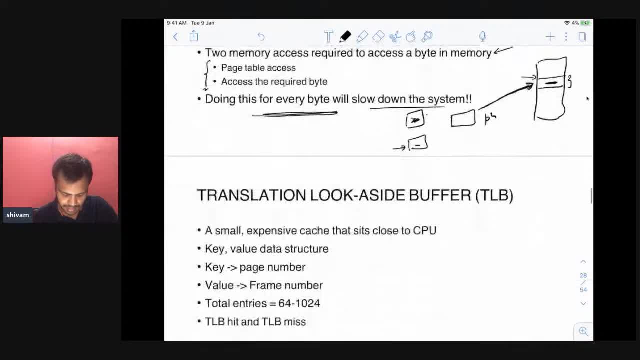 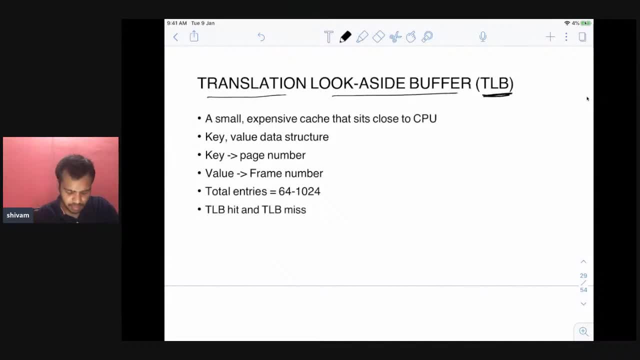 every byte time in every instruction, it will make it slow. that's why the solution is to use the ask station. look aside, buffer. this is also called tlp. this is like a very small and expensive cache that sits close to cpu. as i told you, the most expensive one is the register. you take the cost. 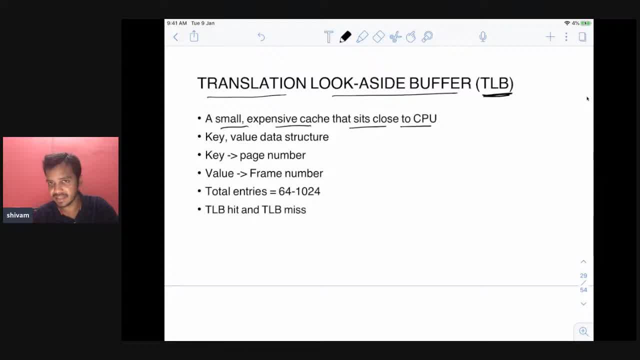 time. then it's the cache and that then is the ram at last with the disk. this is very expensive and it's very small. it's kind of key value, right, it's kind of key value in the sense that, see, it's kind of key value. you will store the page here, frame here, like for page one, the frame is two for. 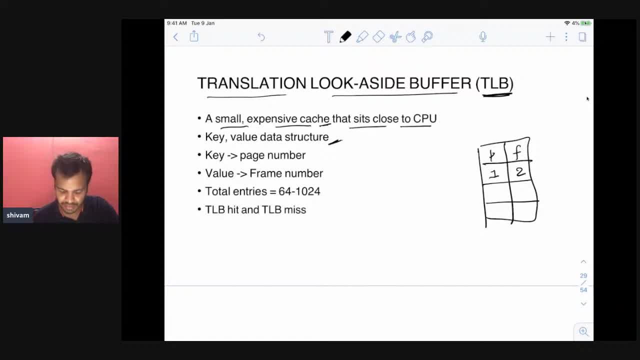 it's a kind of cache right. so it's kind of key value right here. key is the page number, value is the frame number right. very easy to get this. total entries is very small here. you cannot store more because it's very, quite expensive and you cannot store a lot of entries here like entries you can. 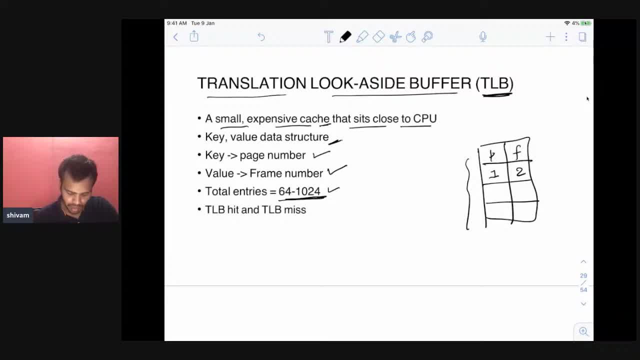 store in 64, 2000, close to 2000 also, what is tlp? see, this is a case right. in every case you will have hit and miss, right. so if that, let's say if you are going for, if you are searching for one at page number one it is found. here it's called a hit. 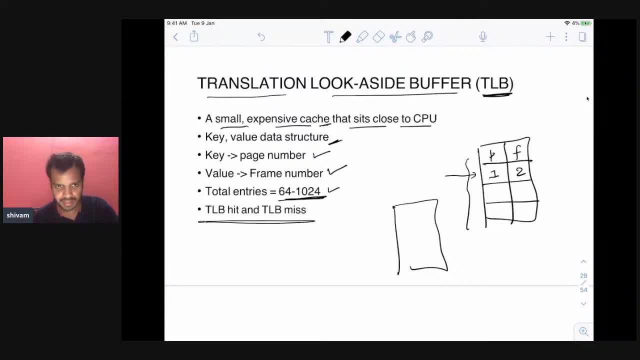 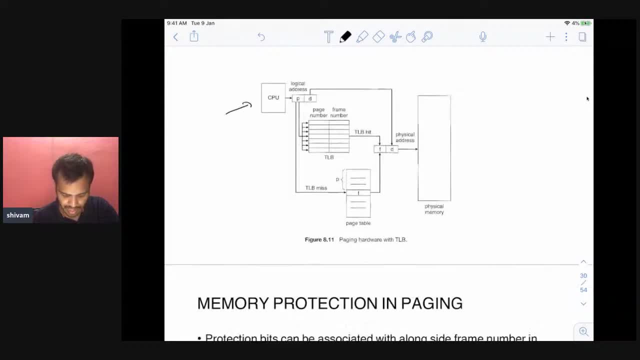 if- let's see if you are searching for page number two here, it's not there. that's called a miss. this is the working of this. see in this case what will happen? the diagram change so you have the logical address: uh, page number and displacement, but first the page number will. 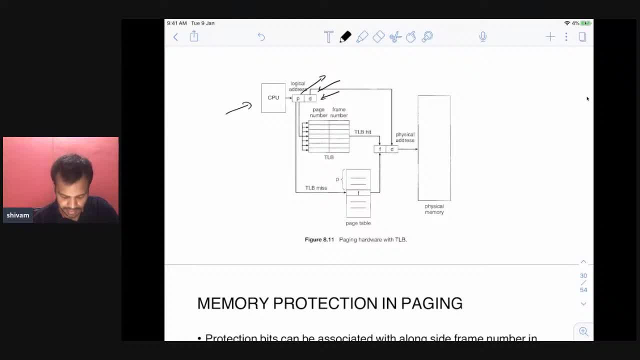 be looked into the tlb cache. so first the kernel will see that. okay, i mean mmu will see. check that if this page number already exists in this mapping, right, if it already exists in the mapping, that means that is the tlb hit and directly frame number can be obtained from there. and you do not. 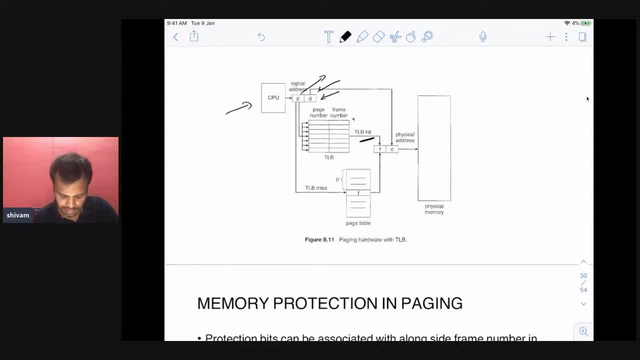 need to go to the main memory. right, it's quite fast. i told you this tlp is quite fast. but in case this page number is not present, in this case you need to go to the page table again, you need to hit the main memory and then you need to face the frame number and again put it here and do the 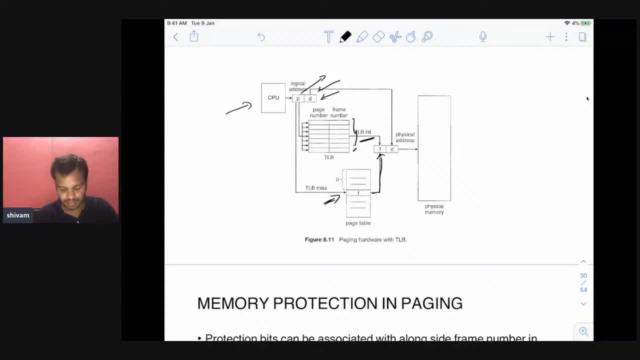 calculation right, but what will happen over the time? a lot of things will, i mean a lot of mappings will be cased in this tlp, and the- i mean the number of times you have to go to the page table in the main memory- will be reduced with the use of tlp. 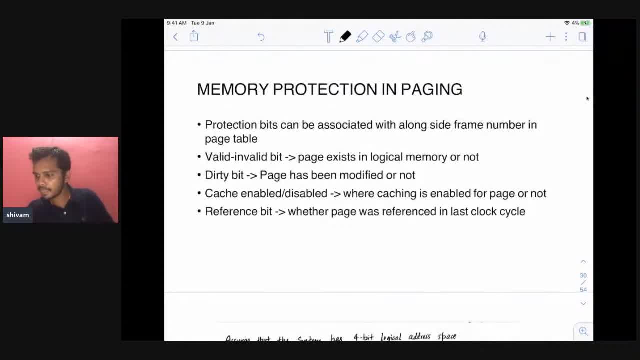 let's look at memory protection in pg. can you march? uh, he's asking: how do i remember this? okay, i didn't, i don't remember all of this. i mean i went through my all my videos, right, and okay, i remember most of this, but i mean i went. 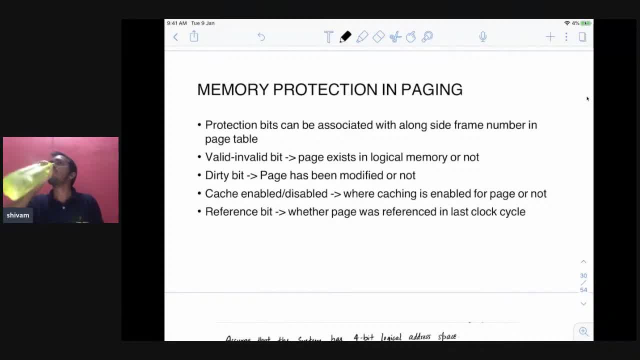 through my videos and prepared this and if i have, if i have the content here right, it also helps me in like going through it and because i have the content here right on the ppt. now let's go to memory protection in paging right now. see, protection, wait, see, you. see, i told you already. 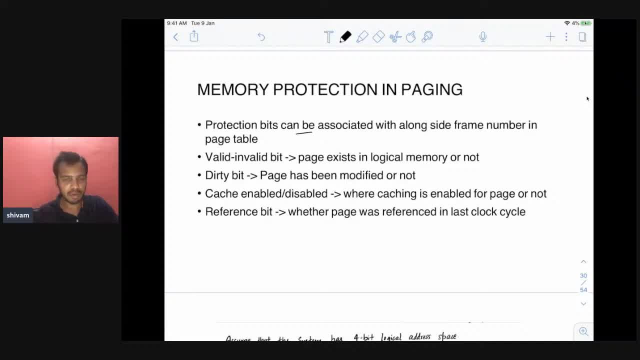 about how to protect the memory in terms of continuous memory, but i have not told you in the case of paging. so let's go to this now. what you can do is you can use some protection bits along with the frame number in page table right, i will show you right. you can use valid invalid bit. 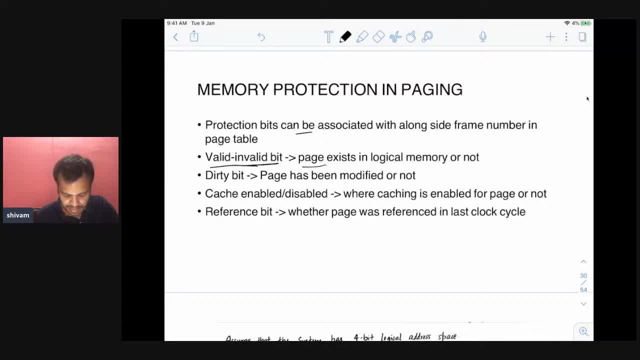 right. this is one kind of bit that means that will check whether the page exists in logical memory or does not exist. you can use another bit called dirty bit. that means page has been modified or not, right, so you can see that the process has returned to that page. that means it has become dirty. 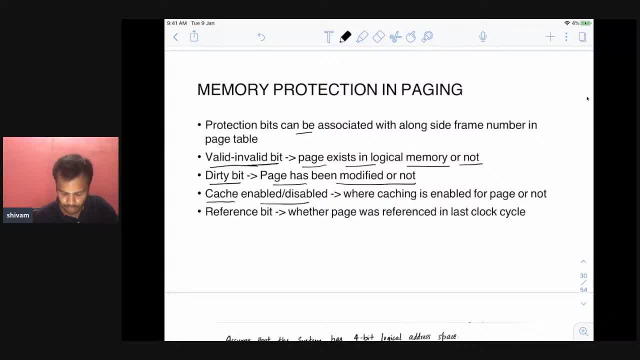 although there are others also, like cache enabled or disabled, where caching is enabled for page or not. if you want to cache some page in the main memory, then you can enable it and this is reference bit, whether page was referenced in last clock cycle or not. so this is normally used for. 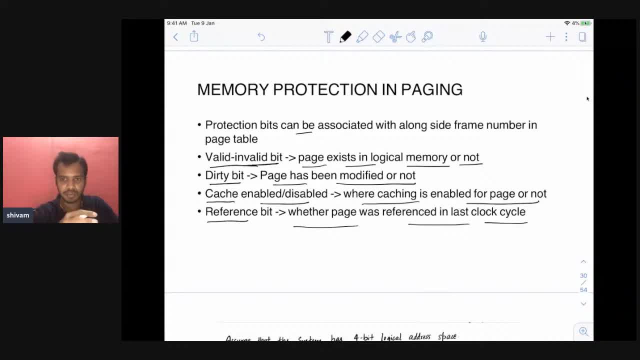 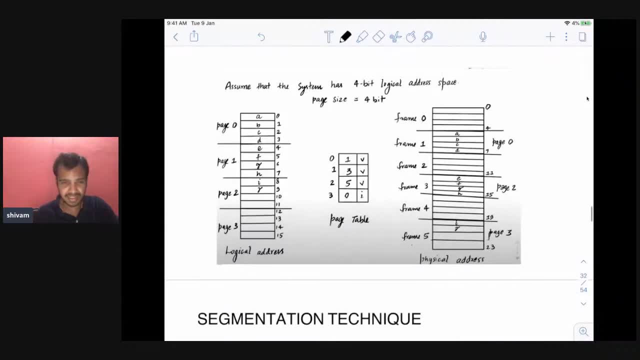 page replacement algorithm whether that page was used in the last time the cpu ran, i mean last cpu cycle. well, let's see this with the example. your theory is, and with example you'll understand. see this: i have drawn a diagram here. i'm not going to details here. 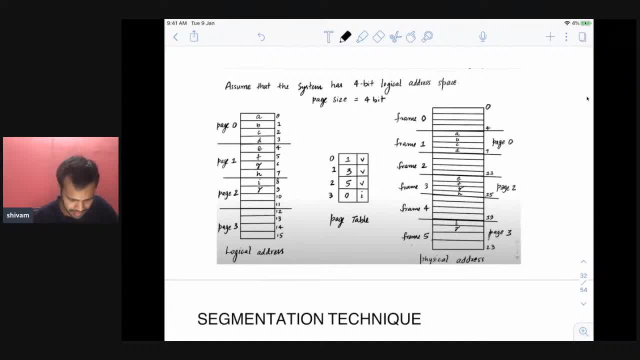 so if you see, azure system has four bit uh. so i have done this calculation, everything, i have divided everything, i've done everything here. now, if you see for uh, if you see here, see this page number three, if you see there is no content here, right, because i mean this process, this program was. 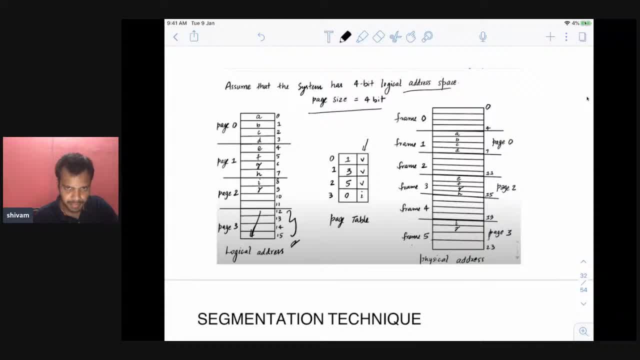 small right and i will use the invalid valid bit here. right, like for, uh, page number zero. it's valid because zero is there, right, is there in the logical address. page number one also is valid. it's there for two also is valid. but for page number three, if you see, i have said this as: 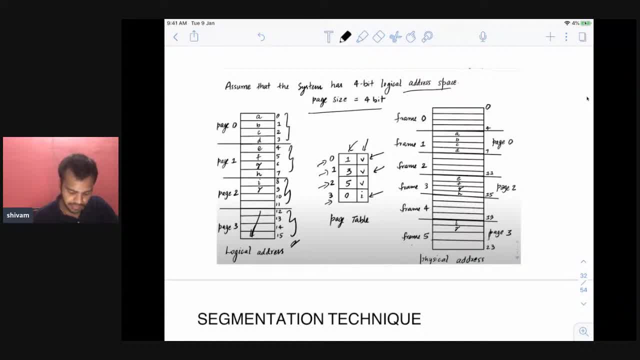 invalid right. that's why it can cause segmentation fault. so if the process is trying to access the page number three- right, it is trying to access number page number three, then segmentation fault will be caused, and that's how you can protect the memory here. quite simple. now let's go to. 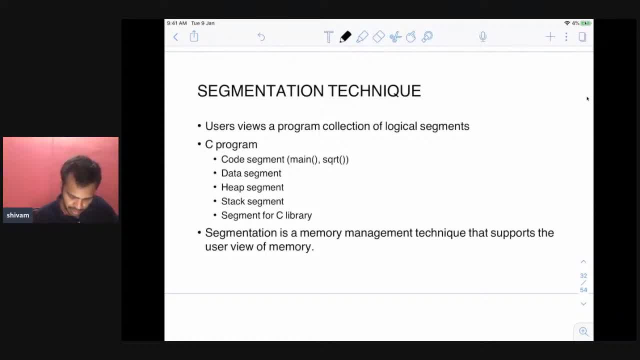 the segmentation technique. a user views a program collection of- see all about view i mean paging, simple paging, and if you have understood the simple paging, i will go fast here, because after simple paging everything is like example of that. how do you simple paging? so i will just show you. my users view the program as collection of logical segments. see how do you. 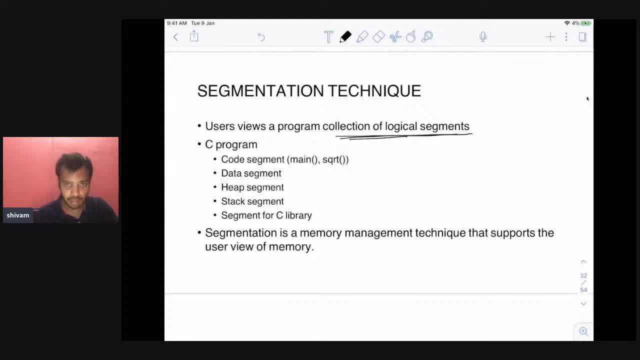 see a program, right, you see a program as kind of you- i mean logically, a user will see it as if you have c program. you will see that as code segment right, that you have main function. you have a square root function. you have add function, right? you will also see that they are data segment, right. 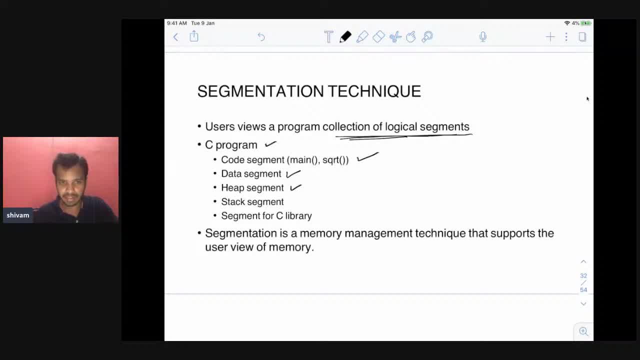 you are also doing map using malloc, right, so you know that. okay, you are allocating into the in the heap section. then you also know that all your local variables are there on the stack segment and also there are some many libraries that you will be using, right, i mean the c libraries. you 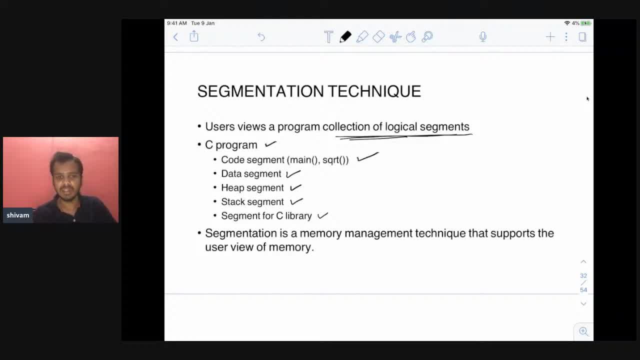 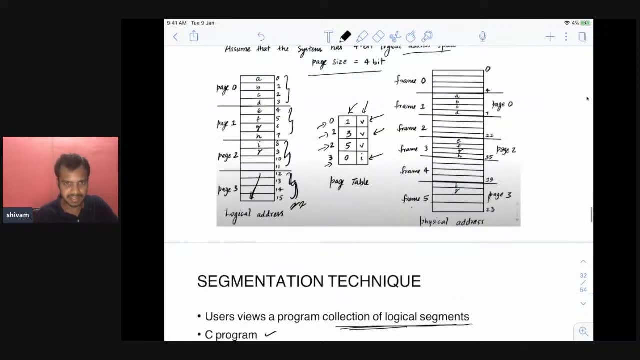 will be using. right, it is sort you are using or anything. you are using those and you are basically dividing in this programming to logical use. that's how most programmers think and segmentation is the memory management technique that supports this view of user view of memory. so this one was this one. you will never think of this way, right, the program is kind of this: you: 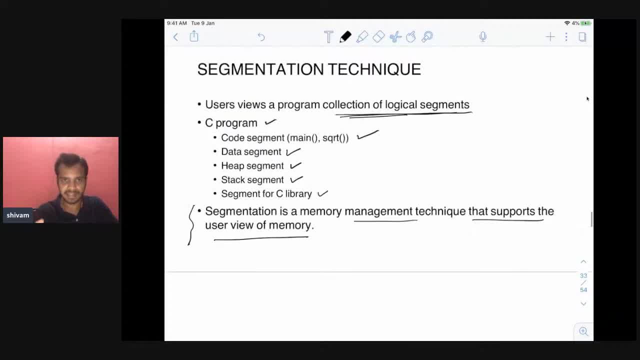 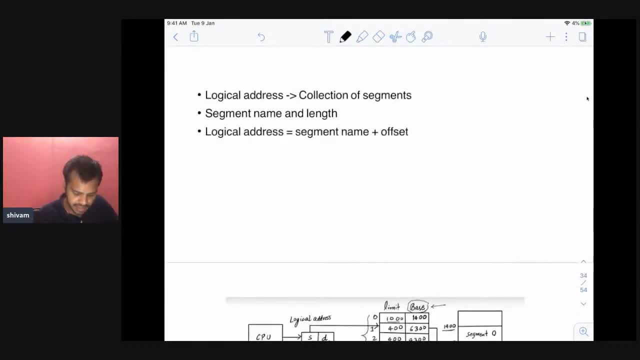 will never think, if the programmer will always think, that a program is divided into four or five memory partitions and there are like code, is there written there this what happens? logical address is the collection of segments. right, you do not have pages here. you have segments here, like i will show. 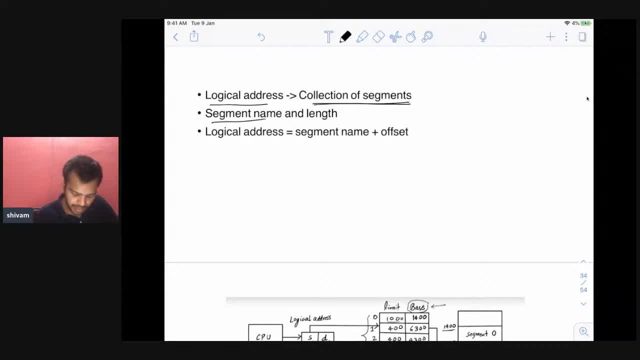 the example here. then you have segment length segment. for each segment there is a name and the length of it- how much is the length of that? and logical address. here is a combination of segment name and offset- see compare this to the page number right in. so in paging you have logical address you have like. 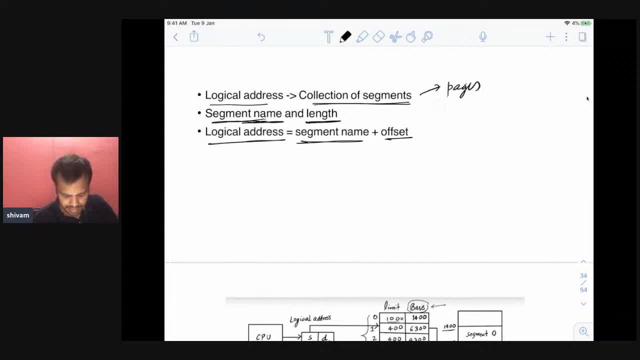 pages. right here you have segments and here you have segment name and length. right in pages you have page size and page number. here in logical address is combination of segment name and offset. there you have page number and offset right. quite similar to that, but a bit different. see this: 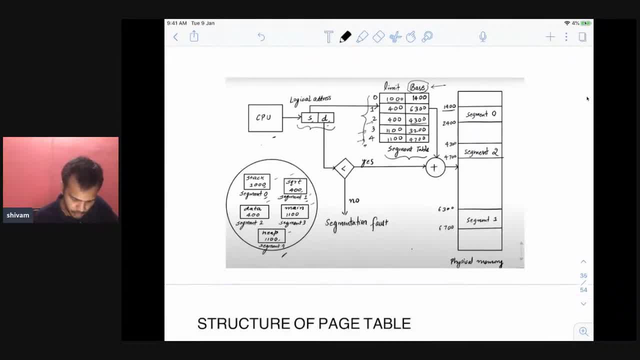 diagram and you will understand, see here, if you see, cpu logical address is divided into segment and we i have like five segments here. if you see, five segments are there and i have provided the size of each of this segment and what is the number of this segment? this segment zero, this segment one. 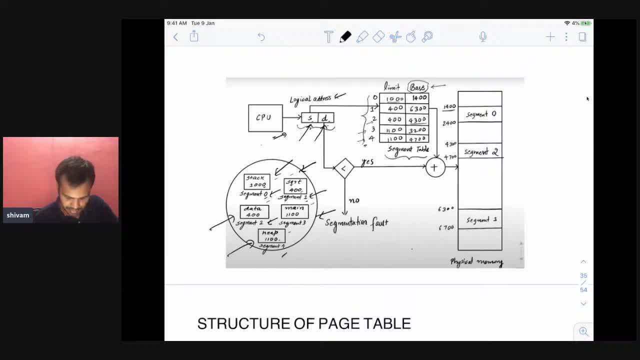 segment two: right like stack segment, square root segment, data segment: right, everything i have done. now this pick: here you don't have page table, you have segment table. in segment table, what is stored like for each of this segment, what is the size limit is called the size of this segment. 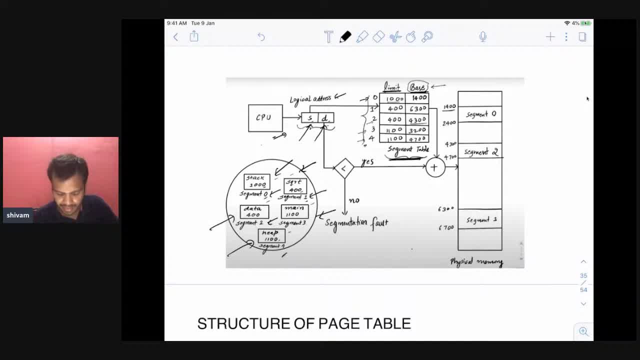 and what is the starting address of this segment in the main memory? that is called base address, right? so i've given some example here. see this: for zero, segment zero, if you see, the starting address is 1400 and this all will be done by the kernel. the kernel will assign the starting address for it. 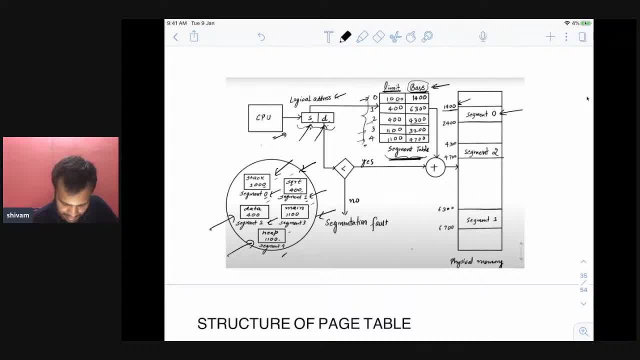 so if you see it is the starting address is 1400 and size is 1000, so it will go from 1400 to 2400. similarly for segment one also, you can see: uh, starting at base address 1600, so from 1600 it. 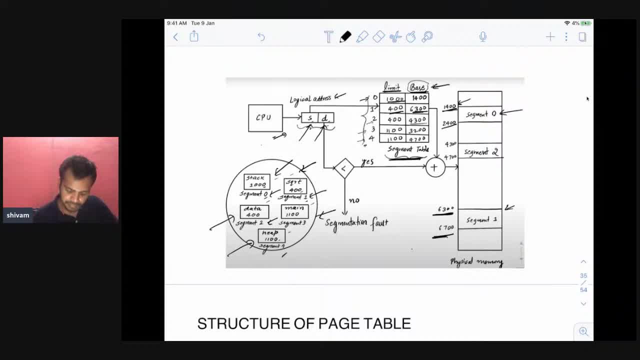 will go to 6700 because size is 400, right? so that's how it happens. now the mmu. what mmu will do is it will see the segment number displacement. it will see whether a segment this segment number, right? no, so first you will see the displacement offset. this offset should be always smaller than. 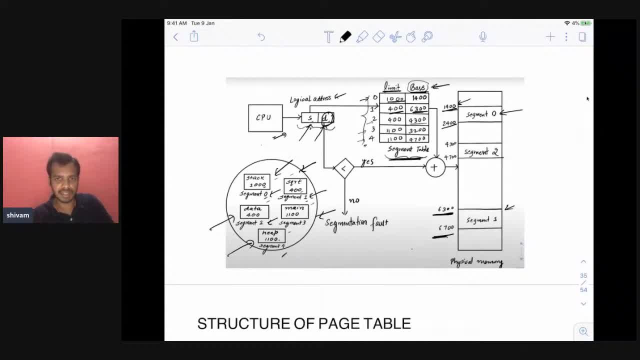 the limit. right, because limit is stored the process size. so of course offset should always be lesser than the process size. if it is not, segmentation fault will be raised. that's how protection is provided here. but if this- it is lesser than the process size, then what it will? 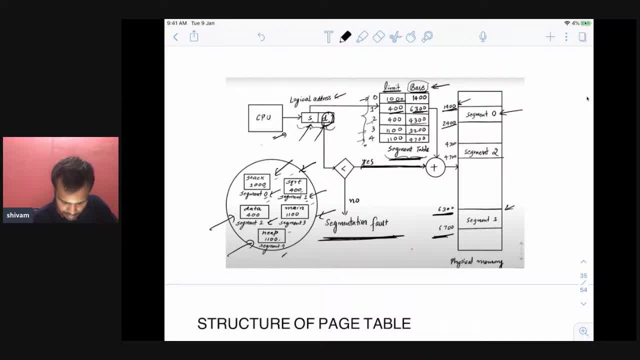 do is it will, uh, sum up this displacement plus the base address, right? so basically, it will say: you see, for this segment, for every segment, we have a mapping for zero. we know, for zero segment, we know this is the limit, this is the base for one, we know right. that's why let's say: if 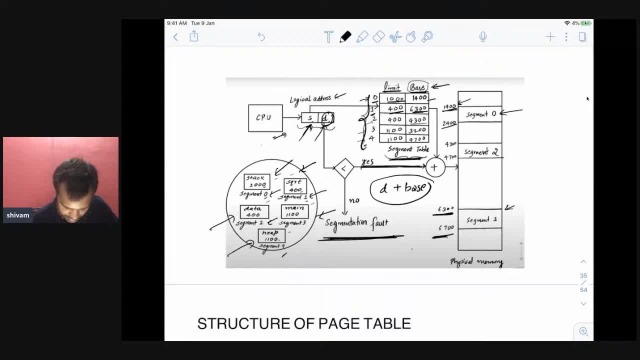 you are going to. i mean for, let's say at this, this address, let's say: your combination is zero comma four, right? this is the combination i mean. your segment number is zero and your offset is four, in this case, right? so you will see that zero is lesser than the size. so 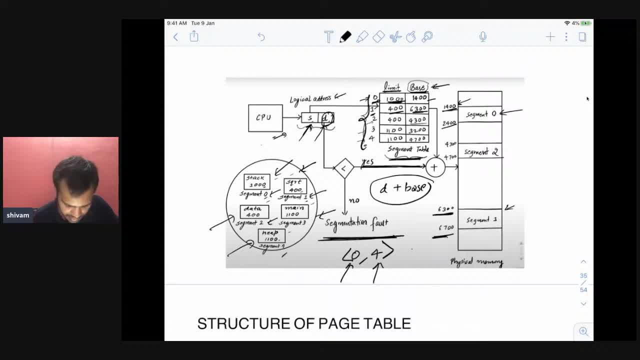 here you see in the segment table zero, the limit size is thousand. of course zero is lesser than what it will do. it will see that. okay, what is the base address in the zero? zero? if you see, the base address is 1400 in the segment table, So 1400 plus what is the offset, right? 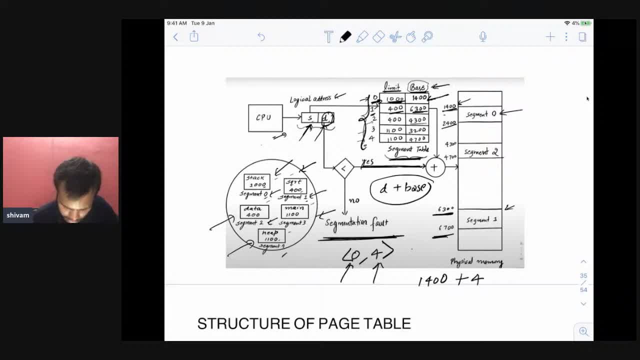 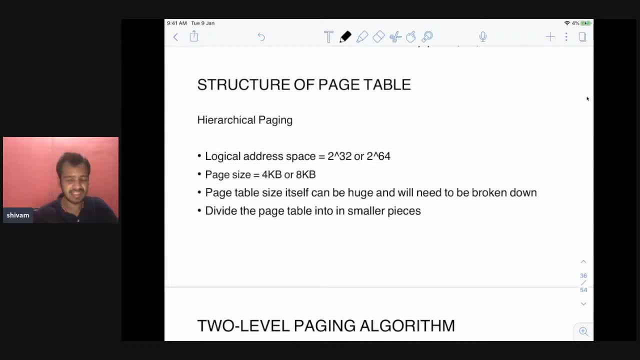 offset is four. So basically, somewhere here it will point to the physical address, which is this one. Now let's move on to the structure of page table. This is like see: page table can be of different ways, right? So I will tell you which one is used in modern operating. 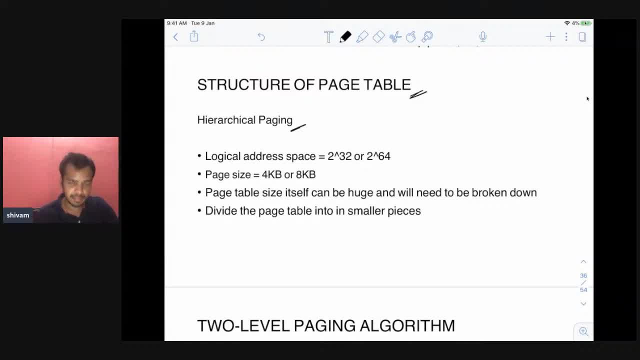 system. So in modern operating system- this one is hierarchical paging- is used actually, and I will explain this how. what is this actually? see? understand this. So why we need this hierarchical paging. I will explain this logical address: space can be very big right 2 power. 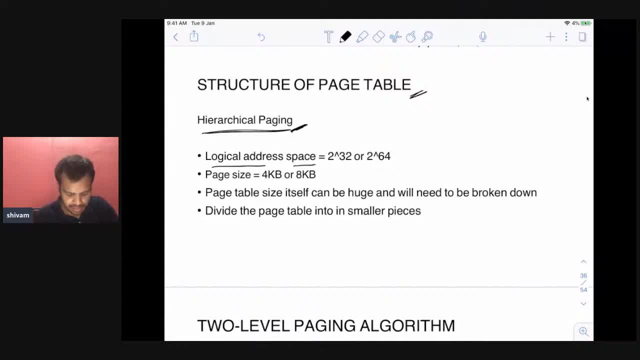 32 bytes or 2 power, 64 bytes, And page size is typically 4 KB or 8 KB in most modern operating system. Now you understand that the page size itself itself can be very huge, right? Let's say, see, you're normally. what is your aim? that you fit the page size right. So you? 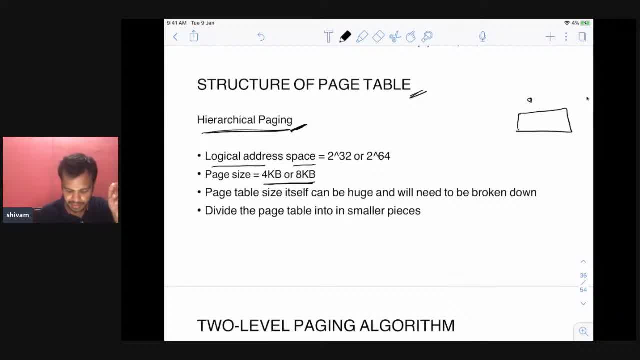 fit the page into the frame. a frame size is eight, let's say 8 KB, But what if the page table size itself is 10 KB? right Now you need to break down the page table also into two parts, right? You understand that right. So that's the issue with. I mean, if 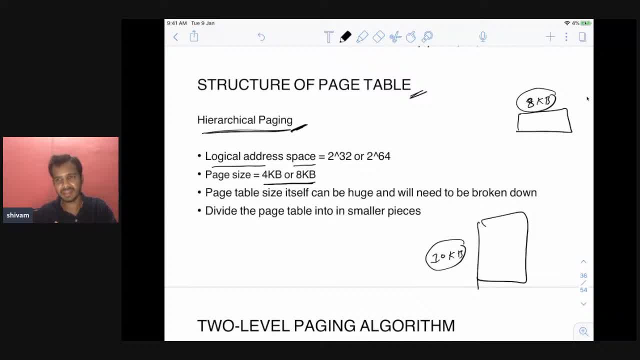 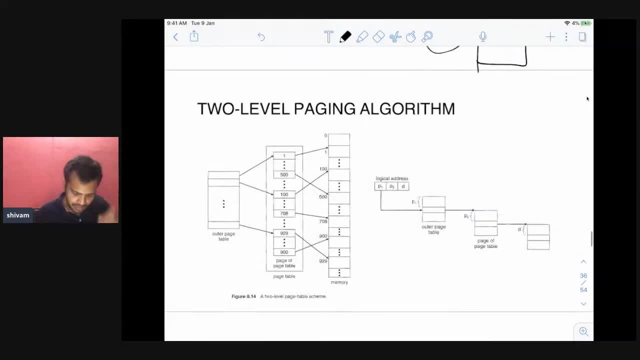 you have like very big logical address space, then the page table size itself can be very huge And then you need to break that down. So this is two level paging algorithm. So that see algorithm is quite simple. So you have two. I mean, I am explaining about the 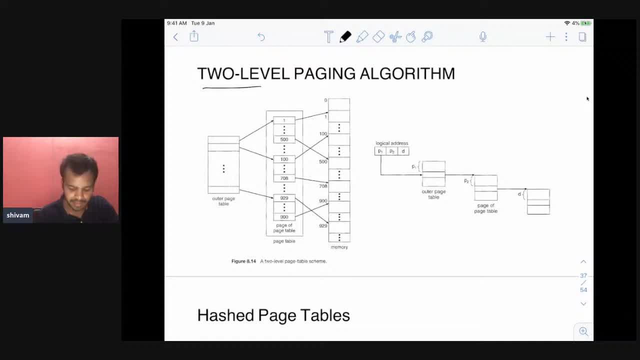 two level, But I am giving a simple example of two level here. So in two level what happens? so you have like one outer page table and inner page table, right? So let's say, if you have address from zero to 100, let's say, right, I mean, these are the address, So I will tell that. 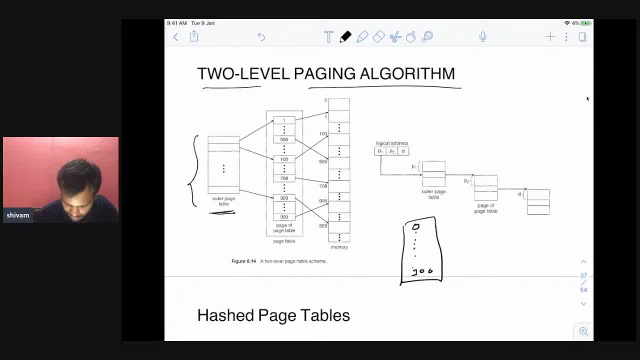 So this is our outer page table. right Now. what will happen? see, let's say zero to 10 is in this table, And let's give an example: 10 to 20 is in this table. it will go on. and let's say: 90 to 100 is in this table, last table. So this is your inner table. these 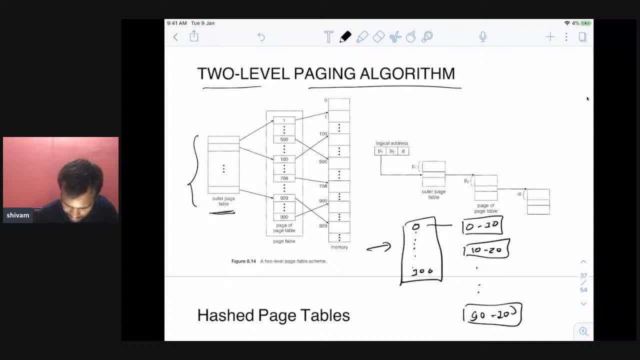 are your outer table. So this is your inner table. So this is your inner table, this is your outer table. there is a mapping here from. let's say, if the number is from like zero to 10, you have to point it here. If the address is from, let's say, 11 to 20, let's 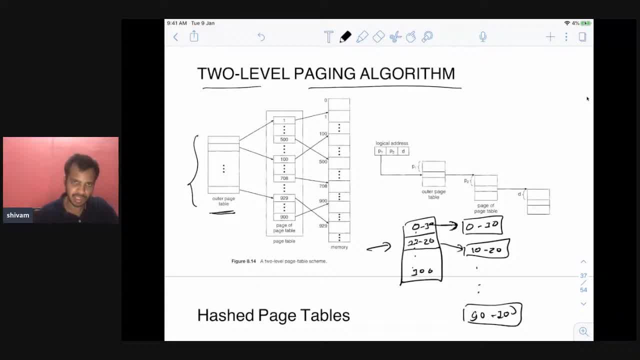 say, you point it here. you understand this right. This is how this tables are: two level paging. you have two levels. First you need to search in this first page table where that address is. Once you have got that, then you need to search this also. So you basically. have logical address as p1,, p2, p3,, p4,, p5,, p6,, p7,, p8, p9,, p10,, p11,, p12,, p12,, p13,, p14,, p14, p15,. p16,, p19,, p20,, p21,, p22,, p23,, p24,, p25,, p26,, p27,, p28,, p29,, p30,, p31,, p32,, p34,, p35,, p36,, p40,. p41,, p42,, p44,, p45,, p46,, p47,, p48,, p49,, p50,, p52,, p52,, p53,, p54,, p55, p56,, p57,, p58, p59,. p59,, p59,, p60,, p60,, p60,, p60,, p59,, p60,, p60,, p60,, p60,, p59,, p60,, p60,, p59,, p60,, p60,, p60,. 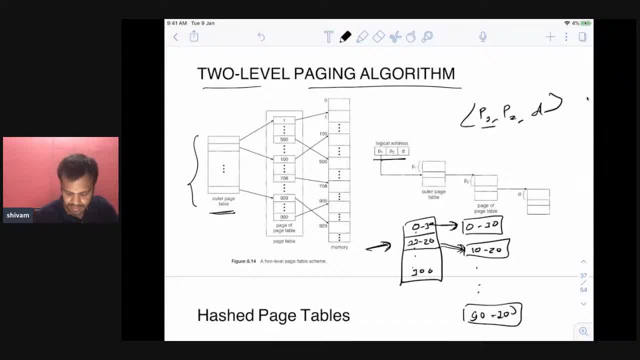 p01,, p02, and displacement. So basically, p1 is the pointer to this one, right. What is the pointer here? P2 is the pointer to this second interface table and D is the displacement. First you go to the p1, right. Then you know that, okay, in this p1 you will find the value. 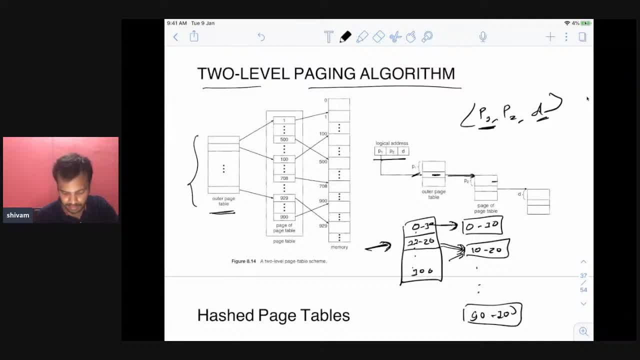 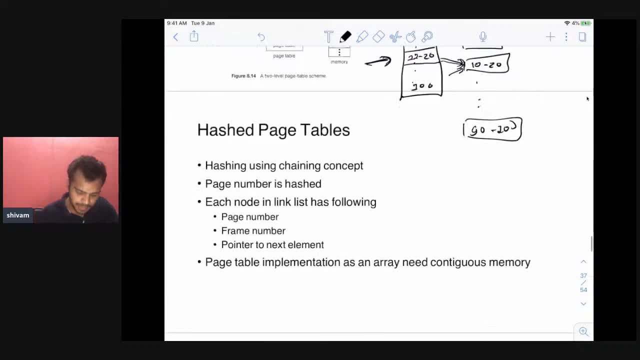 you will go to p2, you will find the final value of frame. from here you will do frame plus D and you will arrive at the final address. Then you have hashed space tables also, Like if you have, I mean, if you know that there is a concept of hashing with chaining right. 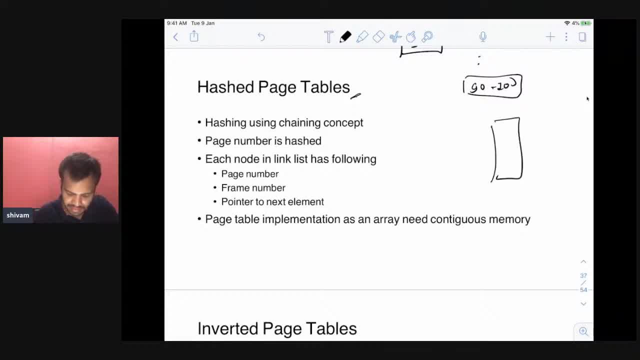 Where you have like a hash table, right Hash table is there And whenever you have collision you create a kind of hash table- Sorry, linked list right. So this with this also, you can implement it. So here what happens. 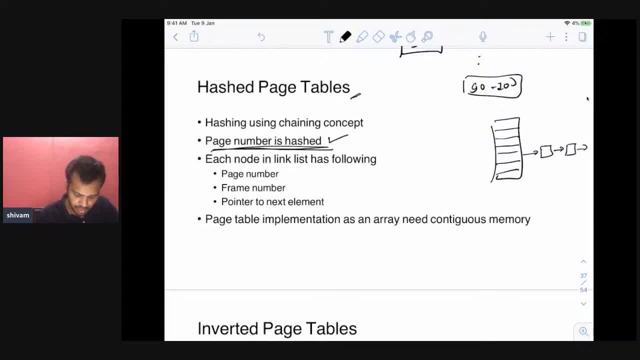 page number is hashed and each node in the linked list will have a page number, frame number and a pointer to next element And page table implementation as array. see, if you want to implement this page table as an array and you know that right Array size. 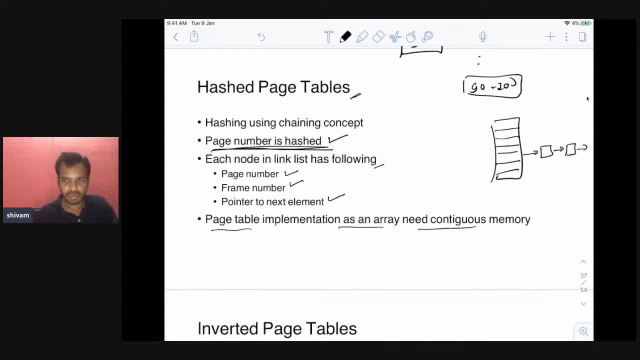 is limited normally, right? The size of array is normally limited, So you want to go for linked list, right? So let's say what you can do is you can create a very simple, I mean kind of linked list and array with linked list and hashing, with chaining, And let's 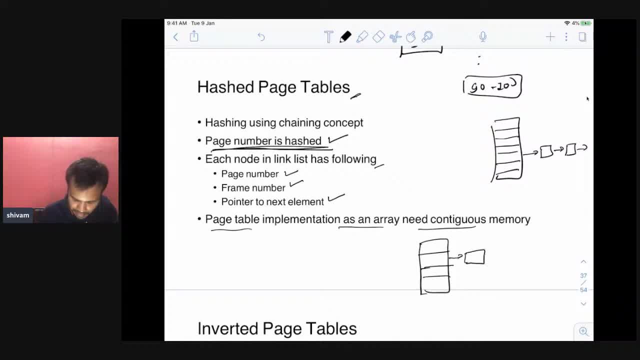 say, and you can have right. So let's say multiple pages will map to this. Let's say two, this is one, right. Now, multiple address, if this is a size, is one, two, three, four, right, You will take modulo of the logical address, modulo four And of course there. 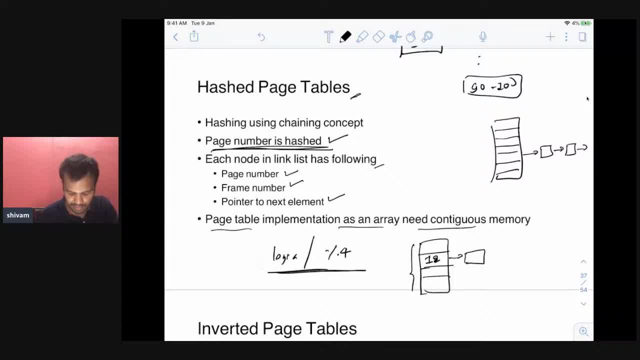 will be collision, right, Because many will give this modulo four as one, right. Then you will have a linked list here. right In this you will have what is the page number, Frame and the equivalent frame number, right. So of course, now you can basically let's. 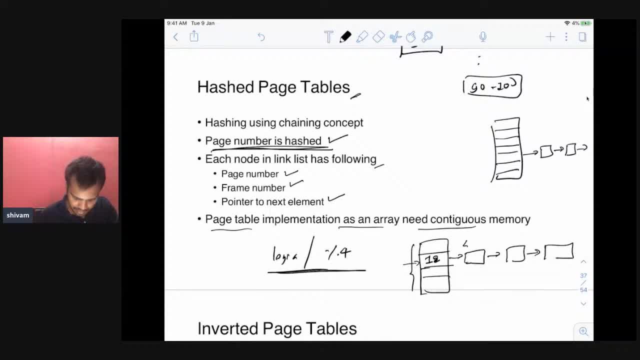 say, let's say- I'm just giving an example- that nine is there right And let's say 13 is there right? These two are the logical address right Now. both will map to the modulo, one right. Both will give the modulo as one. So in this you are storing the frame number. 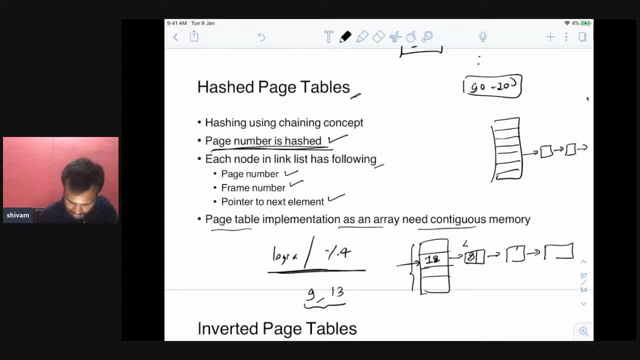 for logical address nine, and this you will store for 13.. And here, here it will be the frame number for this. Here it will be frame number for this. You can easily find the frame number for this by iterating here. So the last one is the inverted page tables. So each 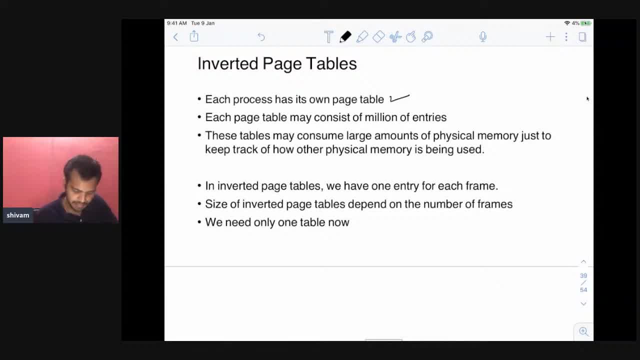 process has its own page table here. See, normally in operating system, each page table will have its own page. sorry, each process will have its own page table. right, Now you understand that? right, Each page table can have millions of entries, right, And this. 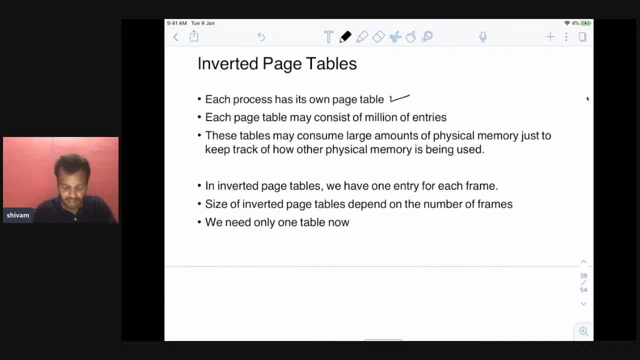 page table itself can take a lot of space in your RAM right. So that's why inverted page tables can be used in those cases, Because these page tables may consume large amounts of physical memory- just to keep track of how other physical memory is being used. 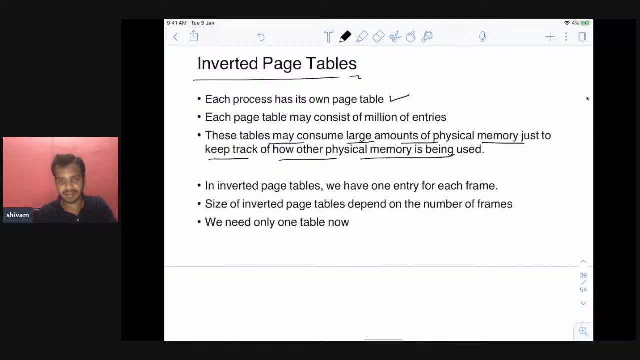 So page table you are using for what you're using for keeping track of the how much physical memory is used, right, But your page table itself, like each page table, is of a size of millions. of entries are there and you have multiple process, So this size can be. 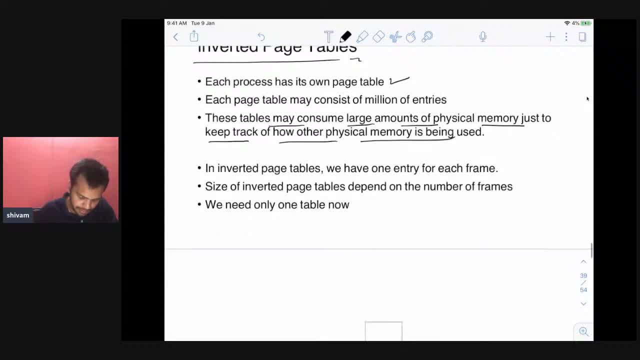 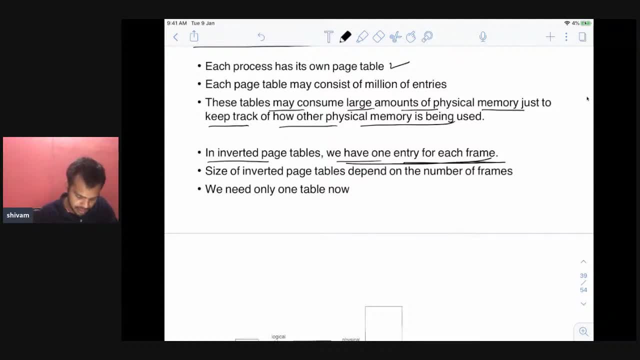 huge here, right? That's why you can use inverted page table. In inverted page tables, we have one entry for each frame. we have only one entry for each frame. Size of inverted page table depends on the number of frames. See, for every frame, you will have one entry. 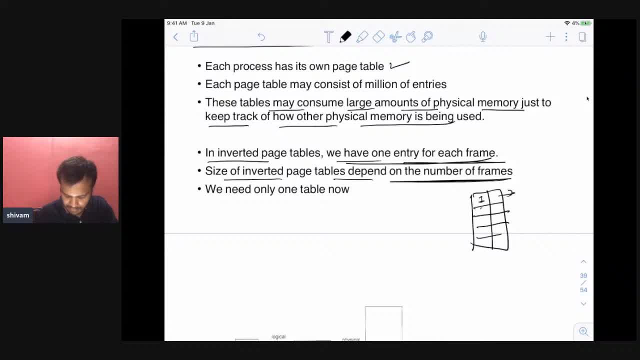 For first frame you will have one entry. for frame two, you will have. for frame three, you will have for frame five, for frame six. So the size of this is limited by the number of frames And we need only one table. now See, for each process you needed multiple. 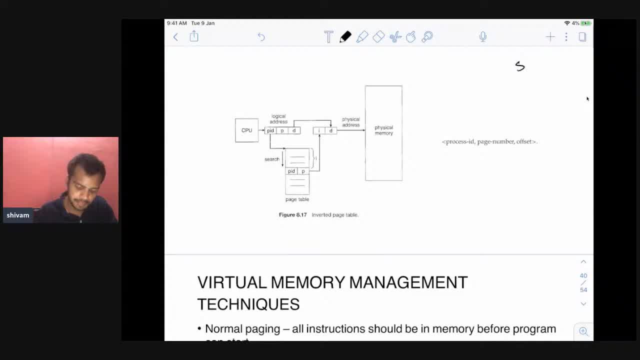 page tables right. So if we have five process, we needed five page tables. But in this, if you use this approach of inverted page tables, you need only one page table for storing all this. See here, the here, the here it is different. you will have PID, the page number and a displacement. 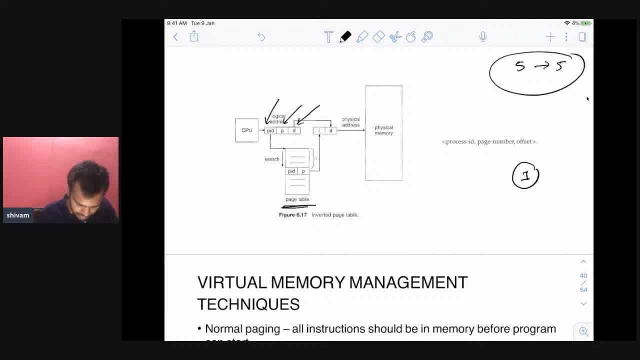 right And this page table. for each PID and P right, the frame number will be stored here in this right, So you can find it from here. where is the time for this process? PID and page number. let's say page number something. what is the equivalent frame number right? 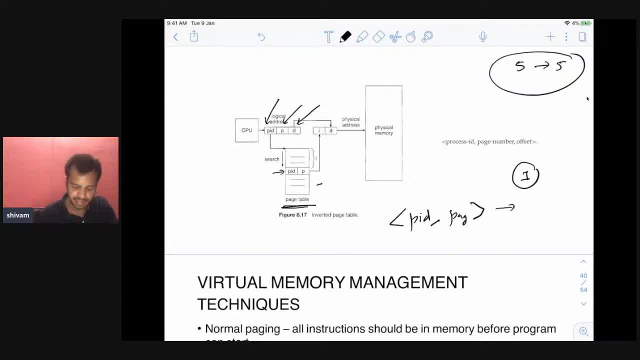 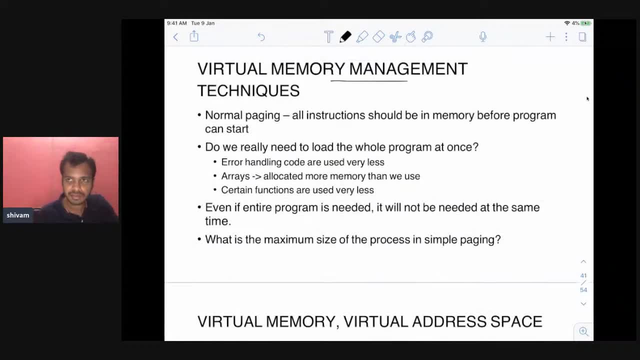 you can find it from here, And then the simpler calculation can happen here. this is inverted page table. Now let's move on to virtual memory management techniques. So this is the second chapter. So how much time is 615?? Okay, I think I will be able to complete after. 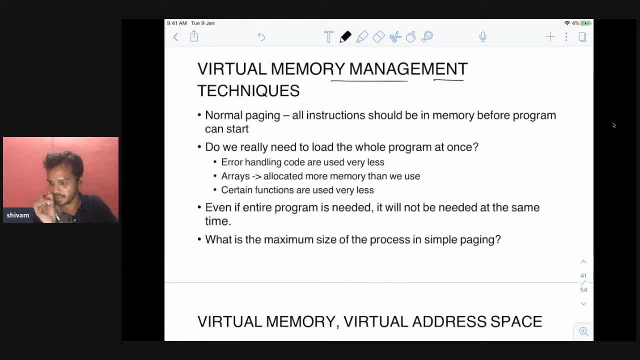 some time. it will take some half an hour more, mostly be there. So see, I have completed everything. Now we are moving to the next chapter, that is, virtual memory. we have completed, completed a simple paging, And simple paging, if you understand in simple paging what happens. 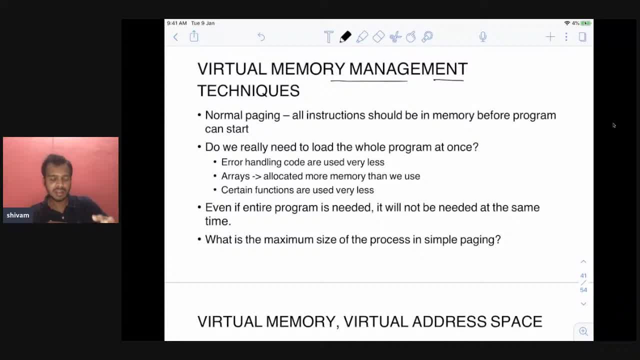 we are bringing the whole process, or don't say process here. So we have broken down the process into pages, logical pages. we are bringing all the pages into the main memory First. then we are running the program or process, But now we will look at other techniques. 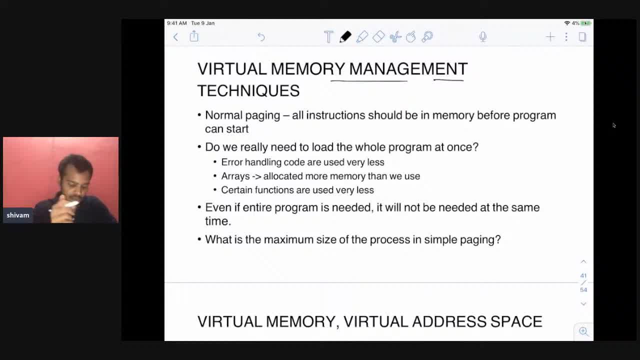 in which we do not need to load the whole program at once. Now let's look at that. That is concept is called virtual memory. See, I do a normal paging. all the structures would be in the memory before program can start. See, now do we really need to load the whole? 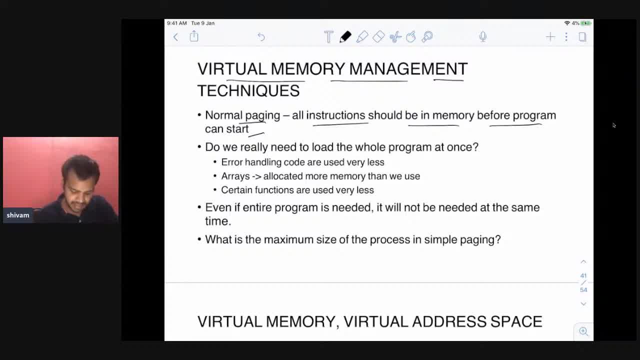 program at once. Ask this question: do we really need? See? there are some like error handling, right, Which will run very less frequently in your code, right, When only errors occur, right. Also, normally in your programs you will allocate the array as 10, power, 5 or 10. 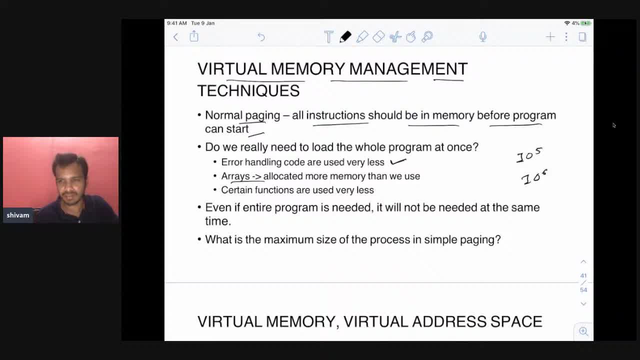 power 6 size of this. but you will not use all of this, right? All of those are mostly right. you do not need all of those in your memory at once. Also, certain functions you do not call multiple times, right? If you have some function you call throughout the 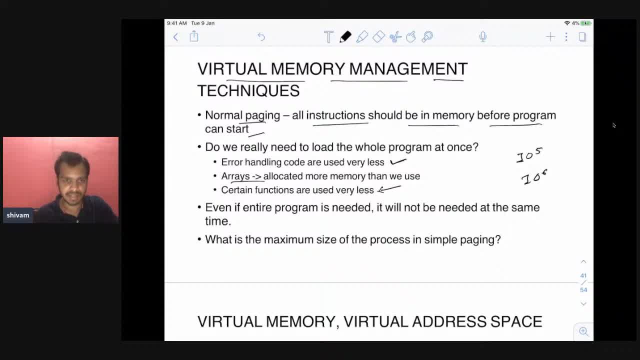 program, you call it only once, or maybe you do not call it itself, right, Let's, even if the entire program is needed, it will not be needed at the same time, right? So you can, even if your program size, let's say one KB, for what all the one KB of code will? 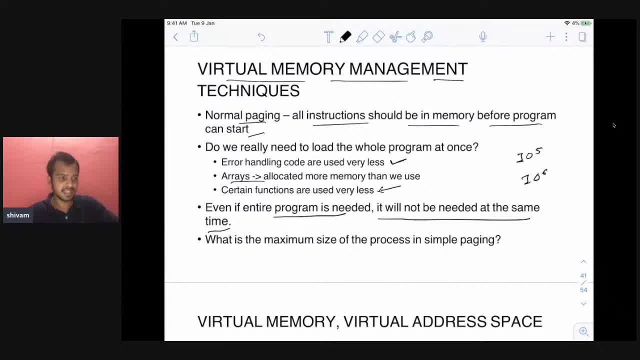 not. you do not need to execute at once, right? It will execute it in the sequential manner, right? Also, what is the maximum size of process in simple paging? right, In simple paging, what happens? See, the maximum size of the process is the your size of the RAM, If your. 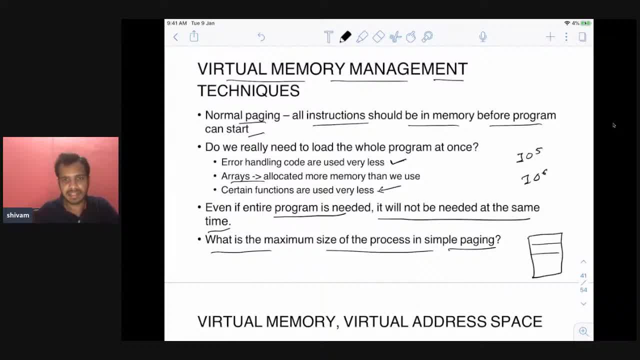 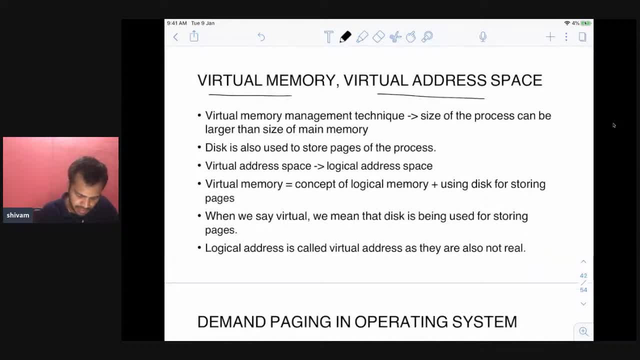 process size is greater than the RAM. you cannot basically run that right Now. let's understand what is virtual memory and virtual address space: See virtual memory management technique. size of the process can be larger than the size of main memory. This is important. So what is virtual memory management technique? 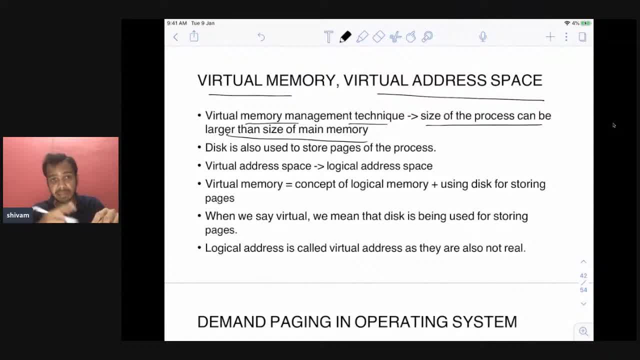 In this technique, size of the process can be larger than the size of main memory. I will think how I explain that, basically with the help. So main memory is already there. We can also use disk to store the pages of the process. So basically here what you're. 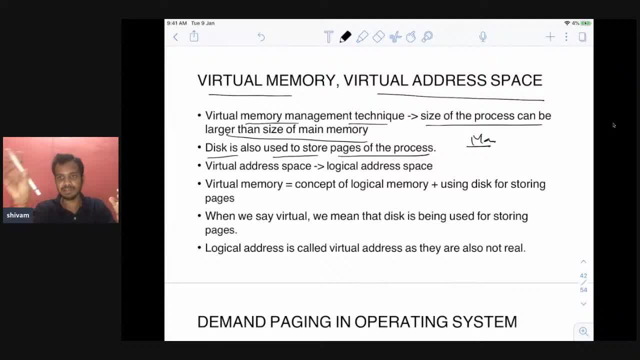 doing, you are using the combination of disk as well as main memory to store the pages. That's why size of the process can be larger than the size of main memory. So, basically, if your program size is of 4 GB, your RAM is of size 3 GB. right, Then, what you can. 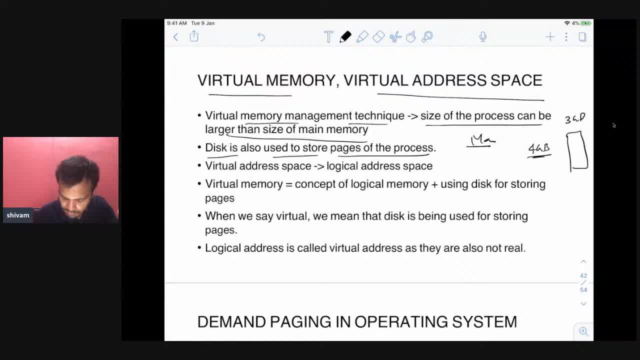 do is 3 GB of program you can put in the RAM and 1 GB you can put on the disk, And we will see how this will work actually later. And you will be confused between what is virtual address space and logical address space. See, actually both are same. Virtual means what? 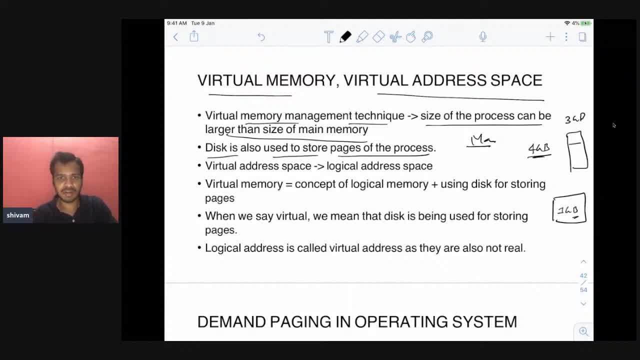 Virtual means not real, right. So logical address are also not real address. Physical address is the only address that is real, So virtual address is also not real address. So almost similar to logical address. same thing, See we will in virtual memory also. 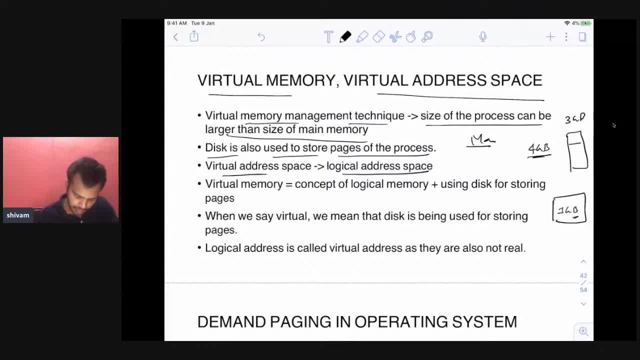 we will use the concept of paging itself. You will see Also, virtual memory is concept of logical memory, plus using disk for storing pages, The same concept we used before. plus we will use disk here, And when we say virtual we mean the disk is being used for storing. 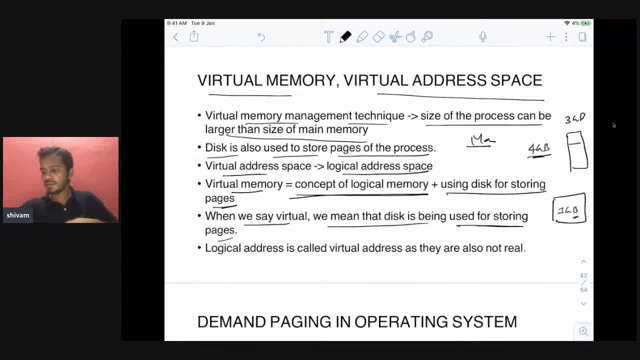 pages. That's what virtual means. Yeah, five people are still there. Okay, so this is the concept of paging. See, whenever you are getting the word virtual right, If somebody says you virtual memory, then think about that. the disk is also being used along with. 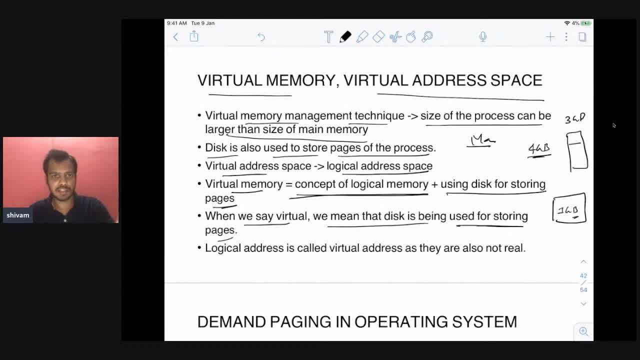 the main memory to store the pages. That's what virtual memory normally means And of course, when this is being used to store your process and the disk size, we can be huge right. One TV, two TV, right. So of course your process size can be greater than the RAM. 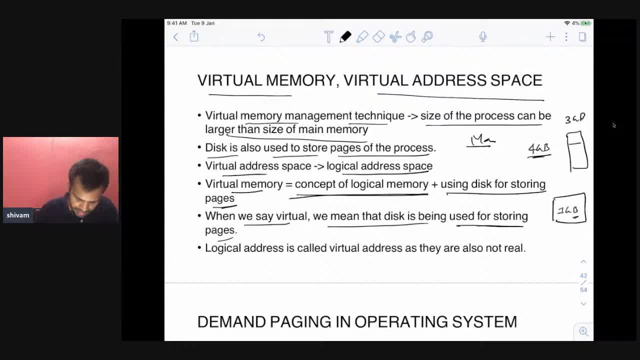 at that moment. Also, logical address is called virtual address, as they are not real. Now do not get confused between logical address and virtual address. both are quite same. So virtual name is basically see I, logical address can also exist without virtual address And 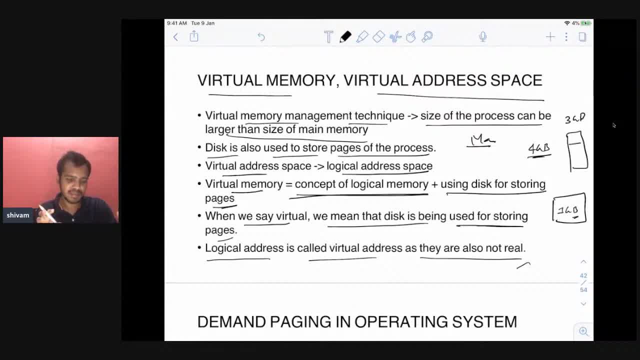 my meaning is that see virtual memory only. understand virtual memory. use only when you have, when you're using disk right For storing. In the previous case, we are not using disk for storage and we were calling it logical address. Okay, now how this happens. let's. 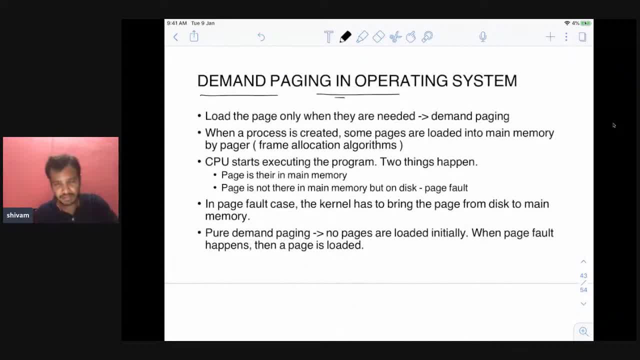 understand demand paging in operating system. This is very important. Again, see, we have understood the simple paging. Let's understand the demand paging. This is actually quite easy if you understand the simple paging. So load the page only when they are needed, right? This is called demand. 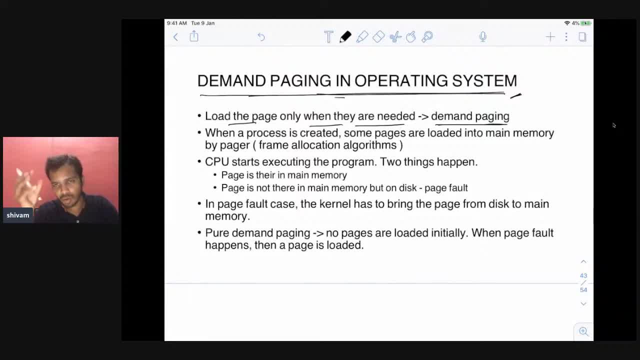 paging. So see, in simple paging, as I told you, all the pages are loaded at once in the main memory and the program execute. In demand paging you will only load the page when there is a demand for that page, That means when some instruction is being executed from that. 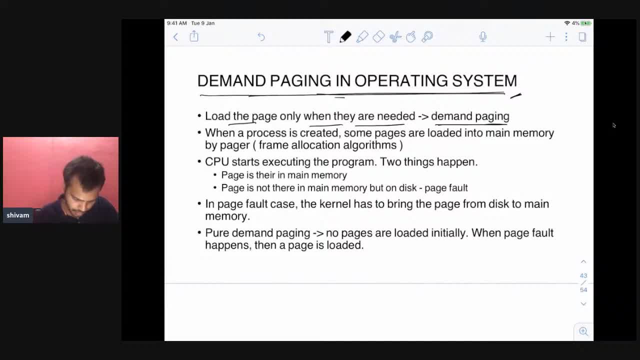 page, then only load that page. Now, when a process is created, some pages are loaded into main memory by pager. So in typical what happens when a new process is created? some three or four or some pages initially will be allocated for that process And this: 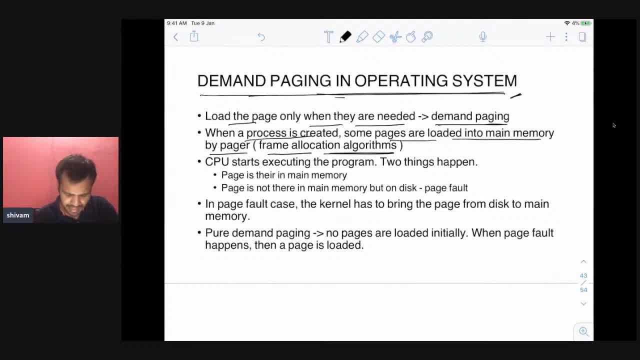 depends on frame or allocation algorithms. So that is different. I mean how, basically, how many initially, how many pages you are going to, I mean allocate for this process? right, That depends on the which frame allocation you are using Now, once the CPU start executing. 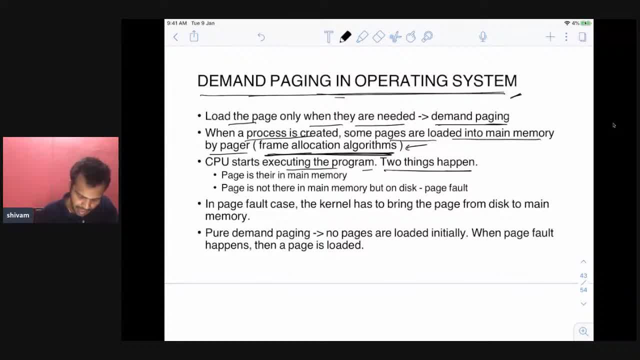 the program. two things can happen, right, Either the page is there in the main memory, right? So let's say, for example: this is your logical address, this is the physical address, this is your pages, these are your frames. let's say zero: zero is already loaded. 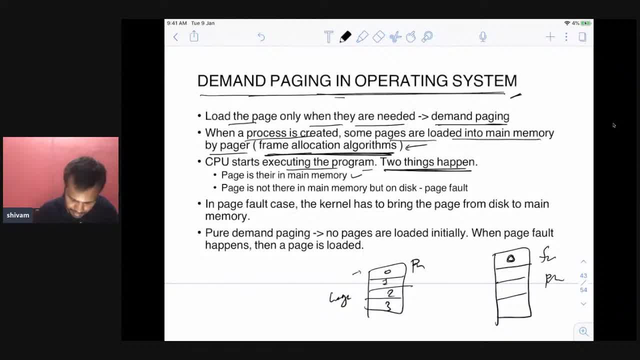 at initially, when the program is starting and all the others has not been mapped. Now CPU starts executing. They're in the main memory. So this is the main memory, right? Initially zero is there in the main memory, so nothing will happen. it can actually execute. 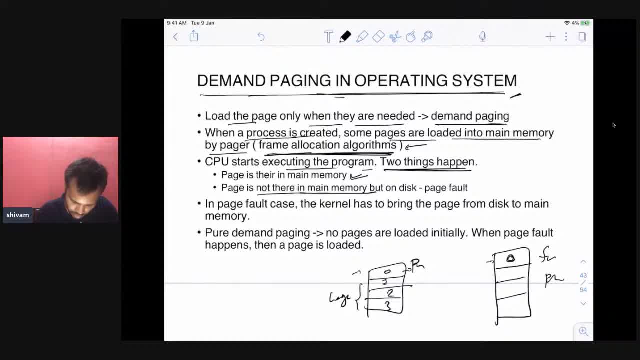 But other condition can also happen: page is not there in the main memory, let's say, when it is going to the instruction in page number two. two is not in the main memory, And that is what will happen. page fault will happen in that case. So that is important. What is? 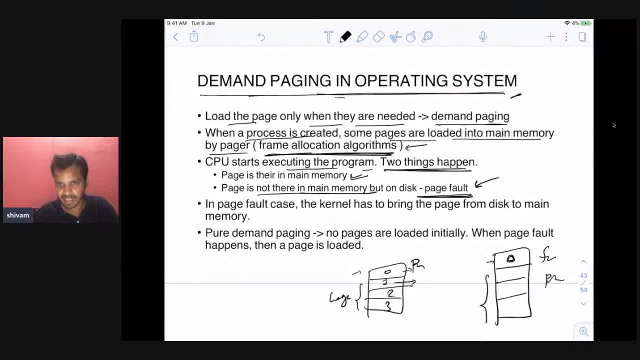 page fault. Page fault means if a page is not present in the main memory and that page instruction is being executed, needs to be executed now by the CPU right And that page itself is not present in the main memory, then page fault happens In page fault. what? 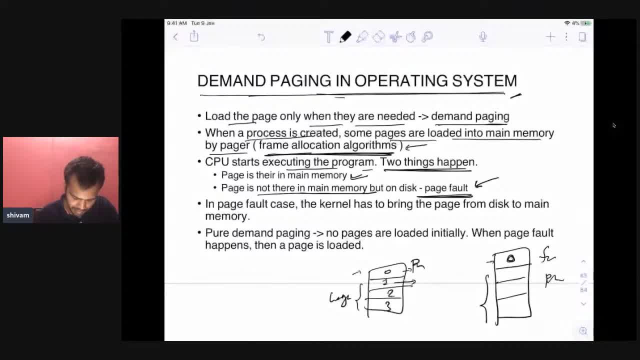 happens. the kernel has to bring the page from this to the main memory, right, This happens. I will explain that, And this is also this is this is demand paging. there is also a pure demand paging. What is pure demand paging In this? what happens in this case? 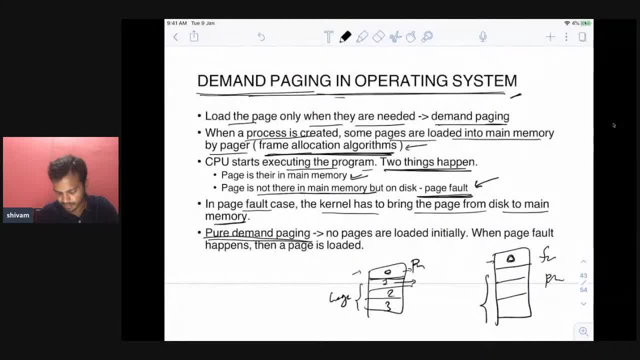 I loaded the page number zero initially into the this frame, right, But in some case what will happen? no pages will be loaded, are loaded initially, when page fault happens, then only page is loaded, So CPU will start executing from zero instruction, and this: 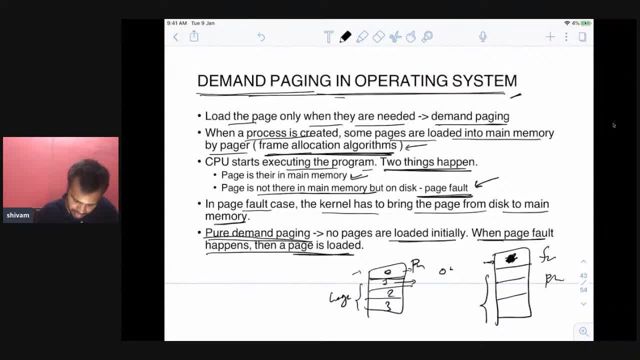 will not be loaded And when it is trying to execute this zero instruction, a page fault will happen because page number is not there. then it will load this page number zero, let's say here, and similar. it will go on. this is called pure demand paging. Also, how does 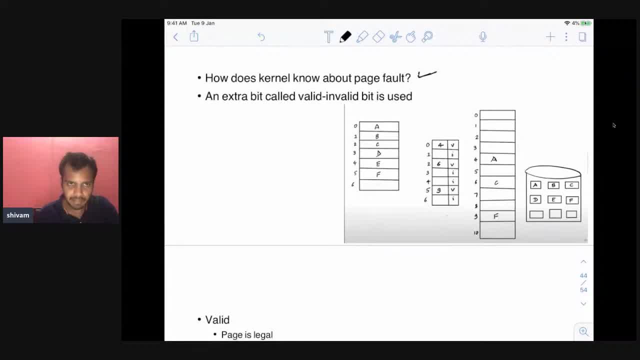 kernel know about the page fault. This is important. So when page fault happens, how kernel will know about this? So for this an extra bit called valid invalid bit is used. See here for every. if you see, for every page number, every page number, there is a 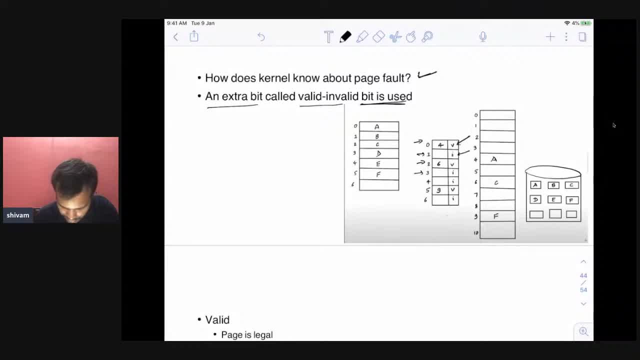 bit called valid or invalid. Valid means: see this zero is valid, So this is valid. this is valid. sorry, if you see this zero is a right. content is a. this is already there, So this is valid here. But the page number one is not loaded in the main memory, So the 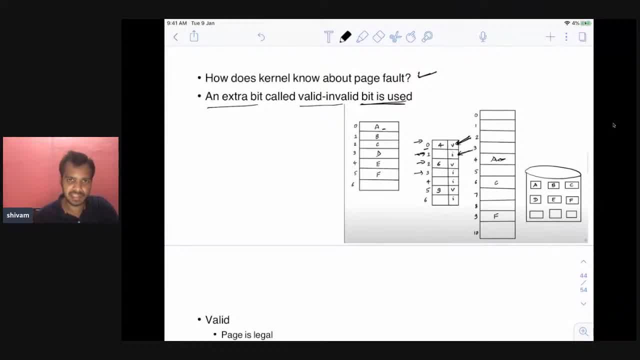 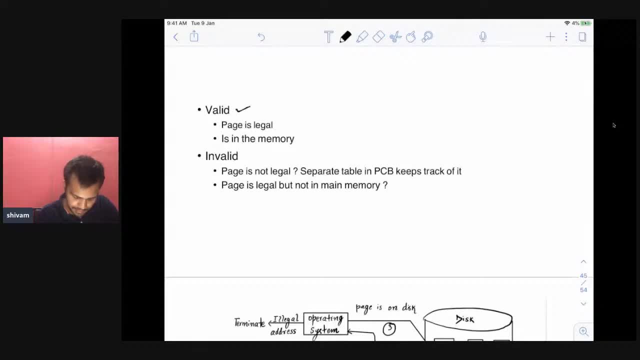 bit is set invalid. That's how kernel can know whether the page is in memory or not. See. but two conditions can happen. if the, if this entry is valid right, That means page is legal. What is the meaning of legal See? legal is that means this address is within. 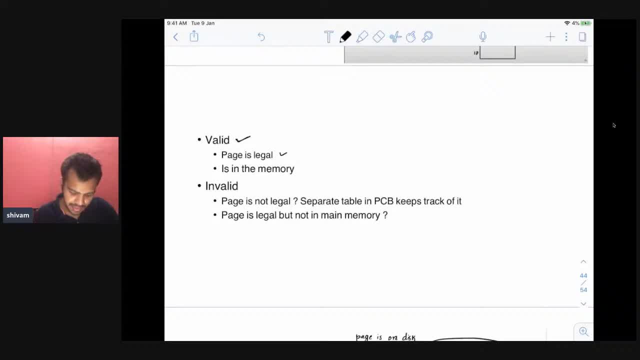 the legal address of the process will have logical address right. And page is legal means that whatever address you are trying to execute, this comes within this address. space is a legal address And also valid means both the things. page is legal is also there. 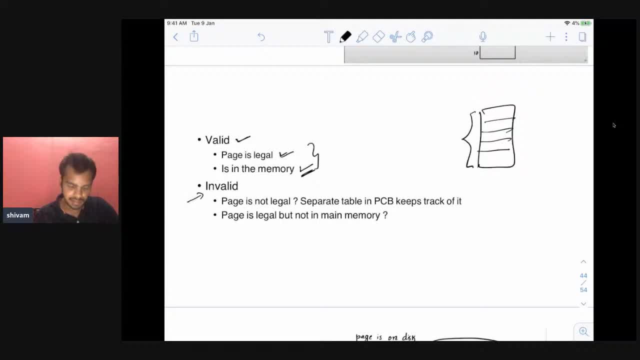 in the main memory. But for invalid there can be two cases. invalid means it can be. either page is not legal right- That means there is a kind of segmentation fault here may happen- or page is legal but not in memory. both of this can happen. So how do you differentiate? 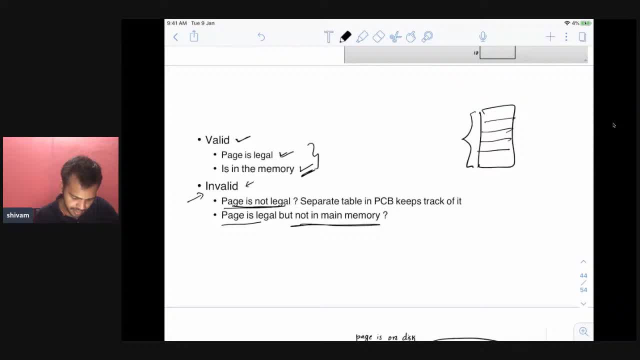 this. So see for this part whether page is not legal. for this. what happens in the page PCB? the information is stored like for each page number. it is stored like whether that page is legal or not. that is stored separately in a PCB table. that is stored from. 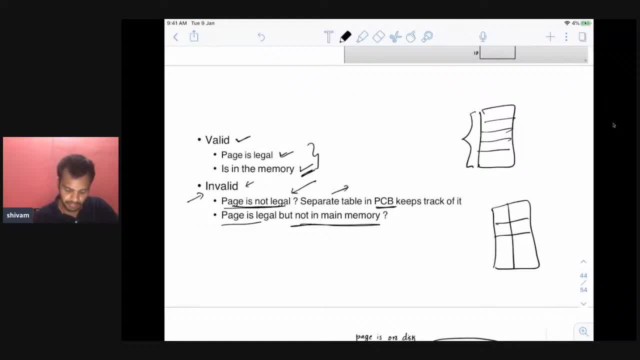 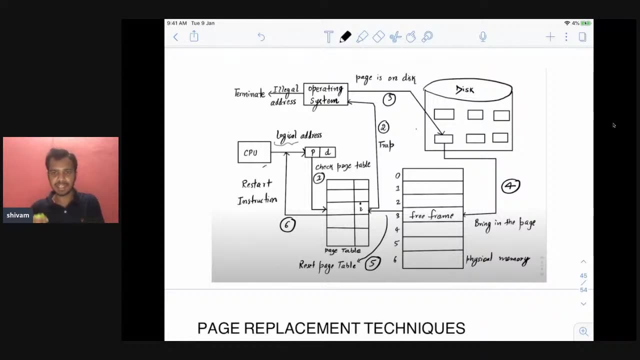 there the kernel can check whether the page is legal or not. Once this is done. after that you can identify whether it is in memory or not. Okay, this one is very important here. Now we are at the last. now. So page replacement techniques and algorithms, and it will be done. 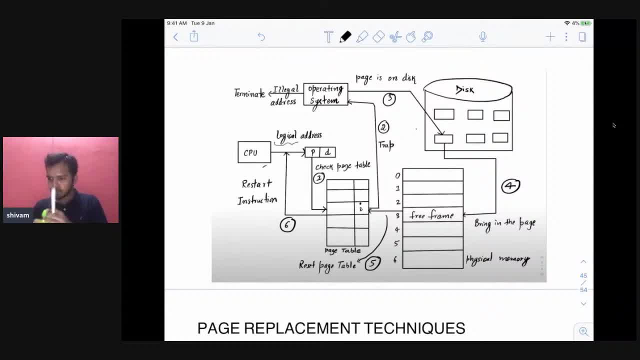 mostly. So see, this is very important. So, how demand paging works. you have to understand this diagram how demand paging works. see what happened. So I have marked down the steps also, like what is the first step, What is the second step, What is the third step. So 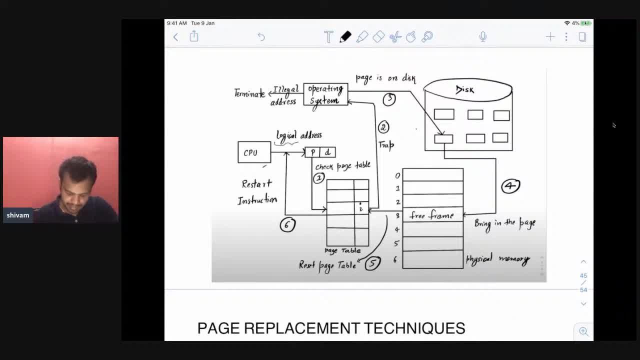 understand this. see, when the logical address is phased right, then first you will check the page table right whether that end frame number is there or not. right Now, let's say you, you will find out that it's invalid. 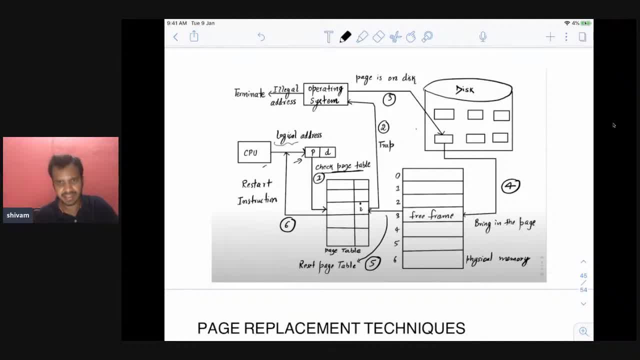 So if it is valid, it is quite easy, right, You submit with the offset and go to the address, But we are talking about the case when it is invalid. So if it is invalid, what will happen? See, what is the second step. So if it is, if this, let's say you are trying to. 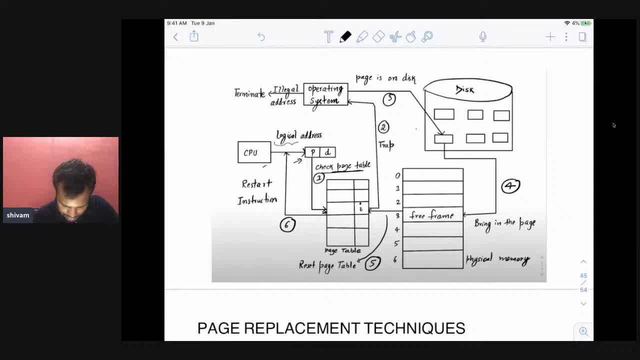 access this page. right, this page, this. you see, the flag is invalid. That means a trap will be, a trap will be executed And now kernel will come into the picture. So the kernel will check first whether this is a legal address or not. 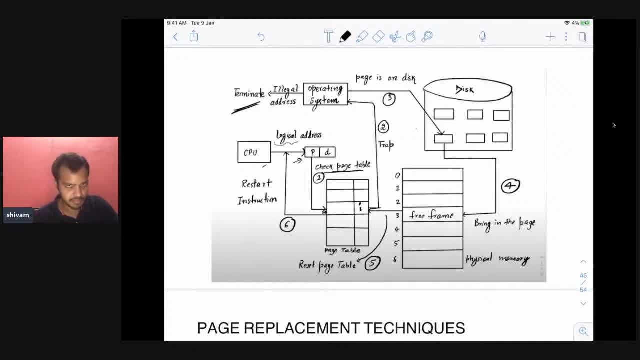 If it is illegal, you will terminate the process with the segmentation fault, right? Because see, I told you, right, if the bit is invalid, you have to check two conditions: whether the address is valid, sorry, whether the address is legal or not. And the second, of course, 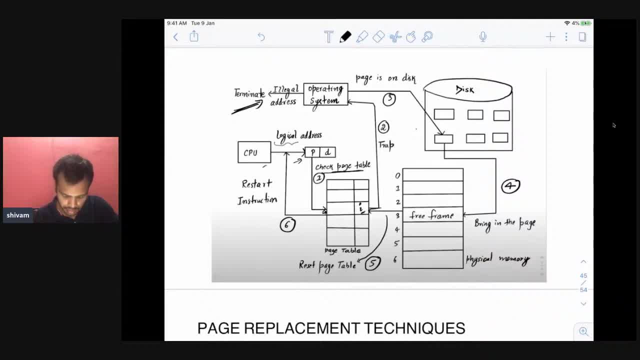 if the address is illegal, then it means that you have a page fault Now. if you have a page fault now, the operating system will go to the disk right and find the page number. Let's say this was 01,. this was 2, right page number 2.. This is the page number 2 in 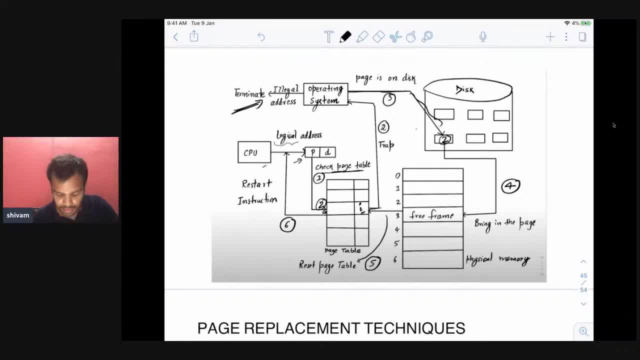 the disk. So it will go to the. the kernel will go to the disk and find the page number 2 in the disk. It will go and load this page number into one of the free frames, right. So that's what so page is on the disk. then fourth step is bring the page into the main. 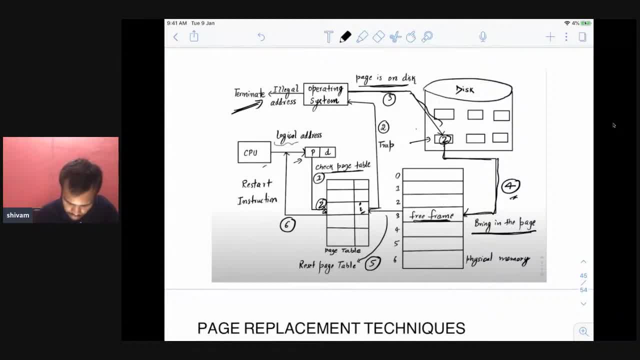 memory. Once this is bought- so the main memory- you will need to reset the page level right. Let's say: this is the frame number 3, then you will say this for 2, mapping will change to 3, this will become valid right After this. once this has been done, again you 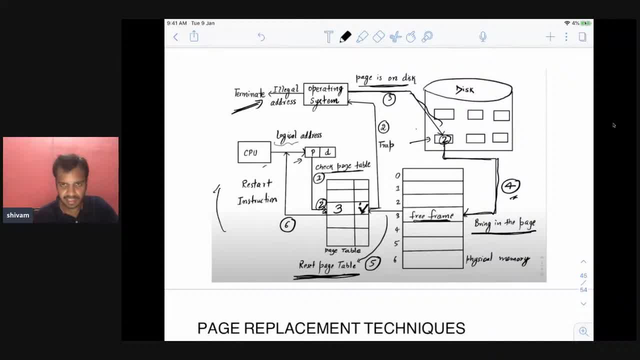 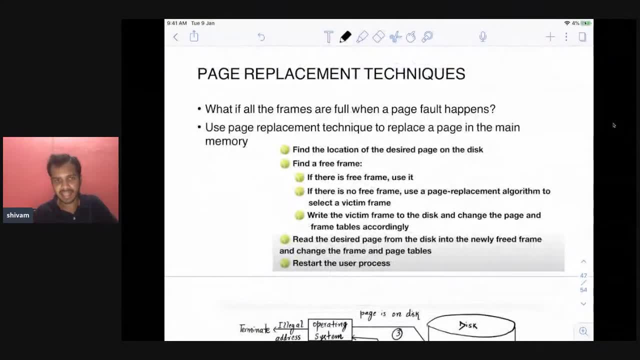 will go and restart the instruction. So this is the typical flow of demand paging. But one more thing can happen, right? You do not? I think you will understand more. I will explain that one more thing can happen, right? What, if? okay, let me go here. 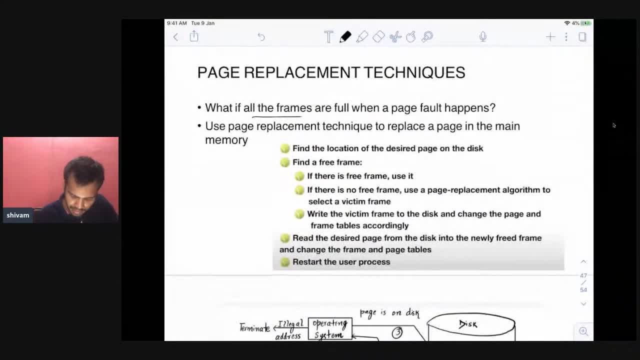 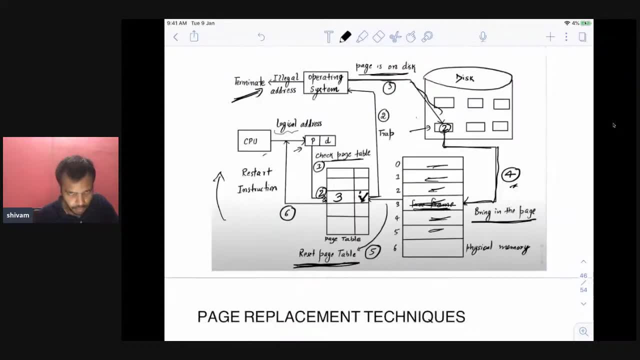 So what if all the frames are full? then a page fault happens. right, Let's say there was no free frames here, all were full. But a page fault has happened and you need to bring this, page number 2, into the main memory. But all the pages- I mean no frames- are free. 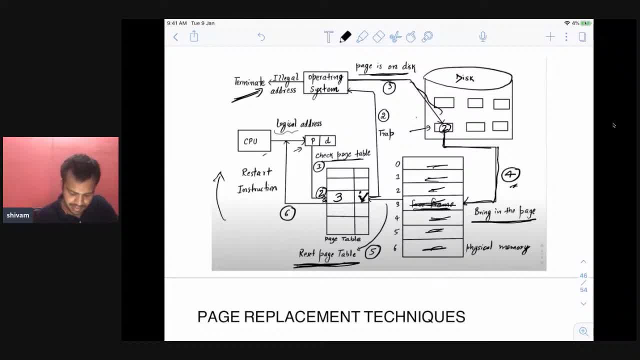 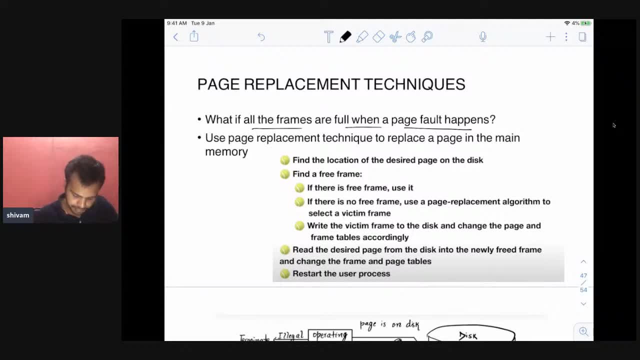 here Then what to do? Understand that case here. In that case, page replacement techniques come into the picture. You need to replace a page which is there in one of the frames. you need to replace that. So use page replacement technique to replace a page in the main memory. 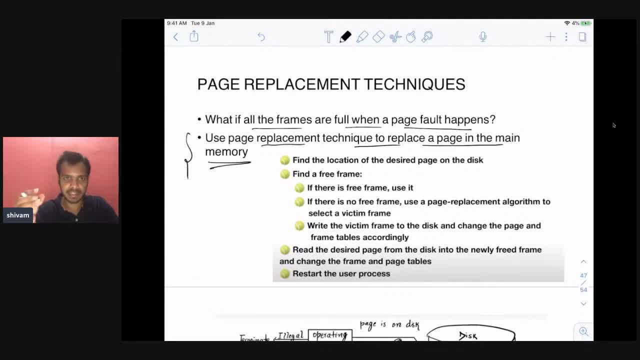 So that's, that is called page replacement app technique. right, You need to replace one of the pages in the main memory. So basically, the algorithm is quite simple: Find the location of the desired page on the disk. first, locate that page on the disk. Now find a free frame. 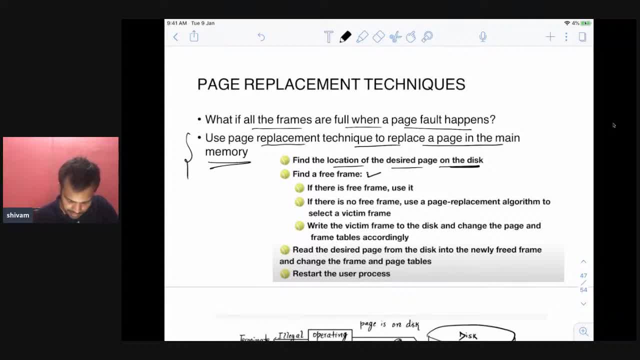 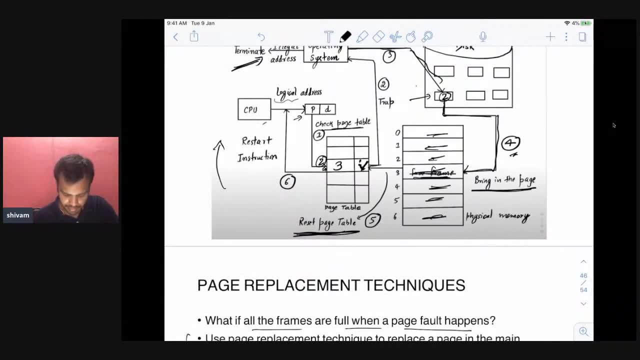 right Now. see now you have to see that if there is a free frame, you need to replace that. If there is a free frame, you can easily use it. That's what we did in this case. right, There was a free frame and we used it. But if there is no free frame, use a page replacement. 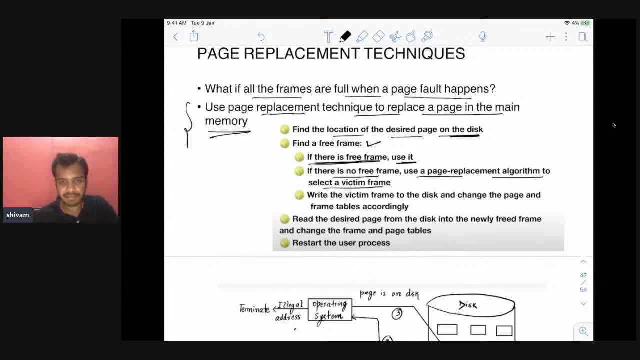 algorithm to select a victim frame. What is victim frame means is that you have to kick out one of the pages from the main memory and you need to replace with the one you are bringing from the disk. That is what the victim frame that you need to kick out Write the. 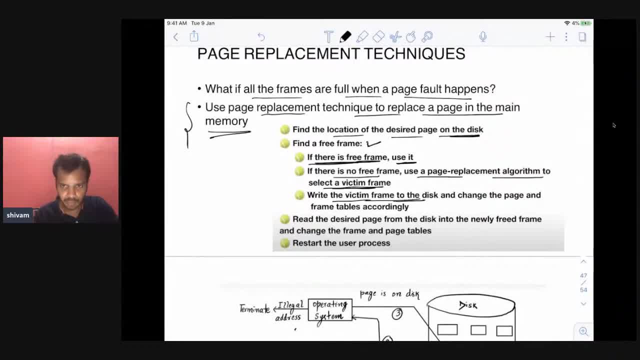 victim frame to the disk. Now you also need to write this victim frame to the disk and change the page table and page. You need to change the page table entries and everything, Then read the desired page from the disk into the newly freed frame and change the frame and page tables. Okay, let 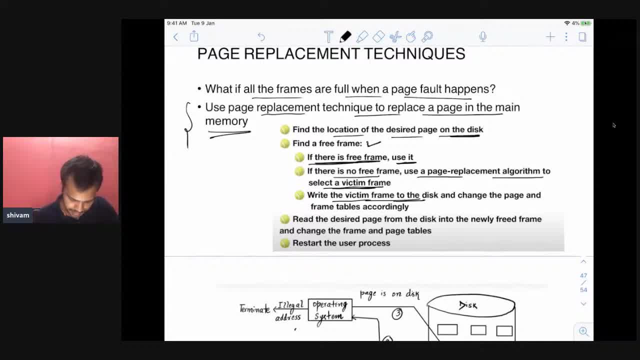 me explain the diagram. It's too much of a theory. See this You have initially. this is the case right. There are two pages right, One and two. if you see page number one and two For one it is invalid. That means it is not there in the main memory. Another is: 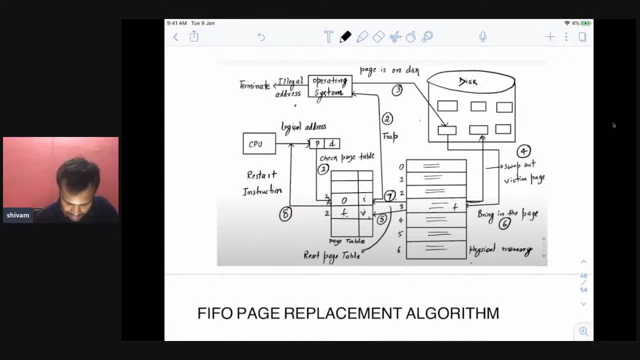 page number two, which is valid, and it has been given frame number F right Now. similar thing will happen. Check page table first. You will check page number two first. You check the page table first, right. Then after you check the page table. you saw that for. 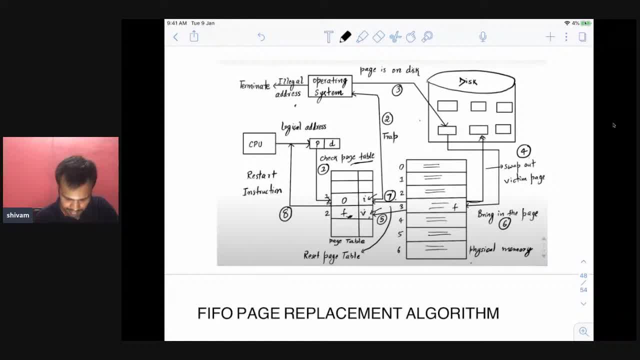 page number one there was invalid entry right. I mean this page. there is a page fault, Then the kernel will go and check that whether the address is illegal or legal. If it is illegal, terminate it with segmentation fault. If it is legal, then go to the disk. 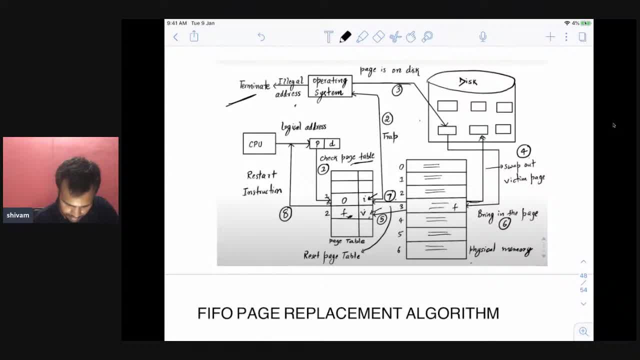 and find this page number one here right. PIN number one is here. It will locate that on a disk. Then it will try to. basically next thing is what? Next is? you have to check if it is possible to bring in a page right. But here you have seen all the pages I mark. 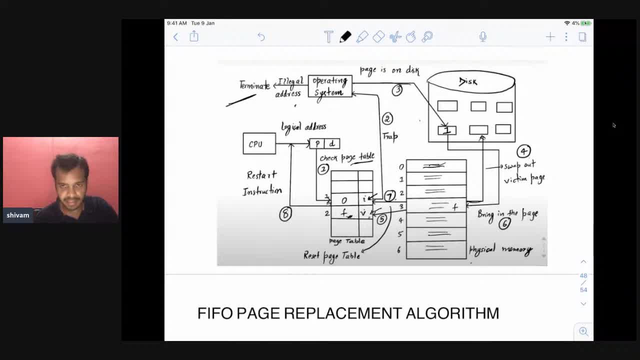 like this. all the frames are not free here, right? Every frame is occupied here. Now you have to select one of the frame Like that is called victim frame and kick that out. right, That's what happens. Fourth step is to find the victim page and swap out Using 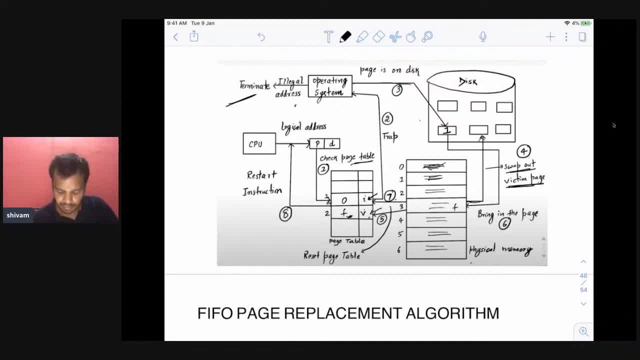 some algorithm, you will find the victim page. Let's say, this was the victim page here. You will kick out this to here. that is, page number two will be kicked out here, right, And then this will keep it down. Thank you. 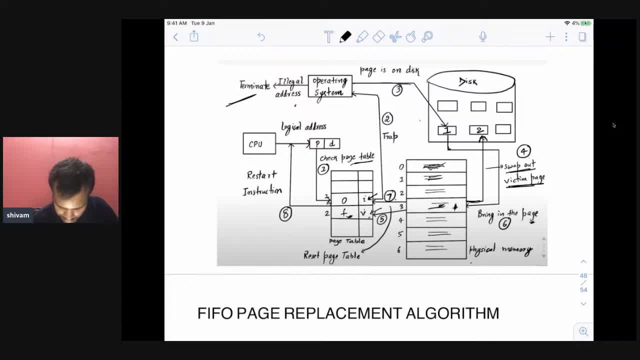 bring in the new page that this is one. you will bring it, this page to here, page number 1 to here, right in the frame number app. you will bring the this one once this is done, see. after this is done, one important step is that you will reset the page table, see. 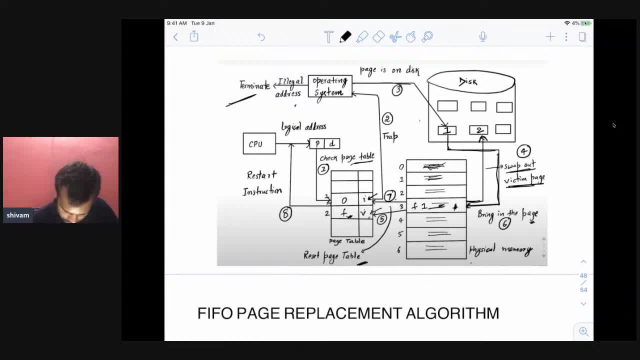 for page number one. so actually you needed to reset the page table when you kicked out right, then only you needed to do this, because i have see after four, this is the fifth reset page table. right, You need to reset the page table. So this, this will become a kind of 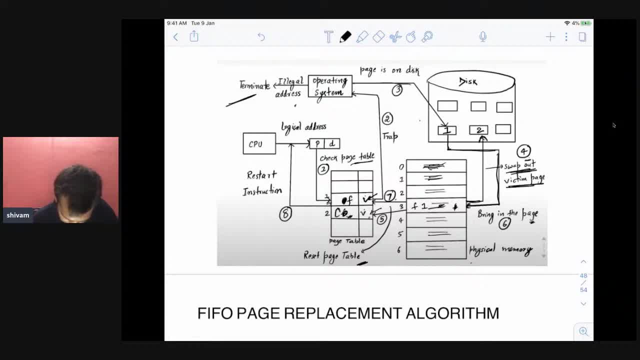 app and valid. this will become zero and invalid And because you have this and the kicked out and this has a bottle, the page table will also change And again you restart the instruction. So this is page replacement algorithm. Now see, this is the last part. there are three. 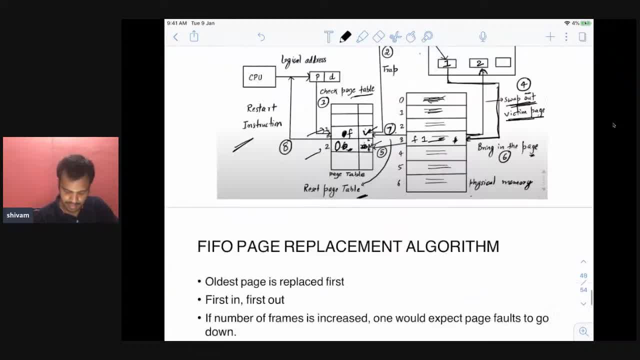 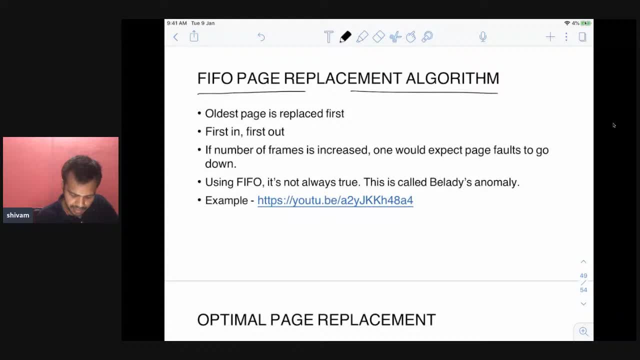 page replacement algorithm right. I think you have understood this case. I will see the comments if there is in doubt and I will cover that. Now that you have FIFO page replacement algorithm right In this, what happens? the oldest page is replaced first, right? That? 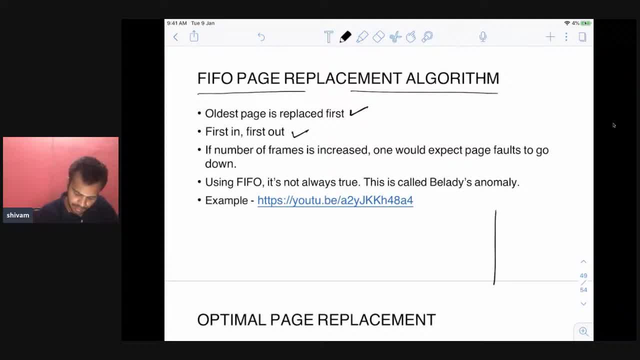 is the first in first out. See, in this RAM multiple pages would have been bought in right: P1, P2, P3, P4. all would have bought it right. There is a time for this was T1, right P2,. 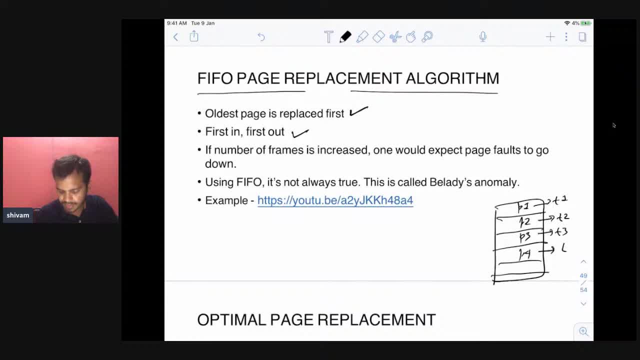 P3. I'm assuming that T1 is more than T2, T2 is more than T3 and T3 is more than T4. That means P1 was bought first, P2 was bought after this, P3 was bought after this. So this: 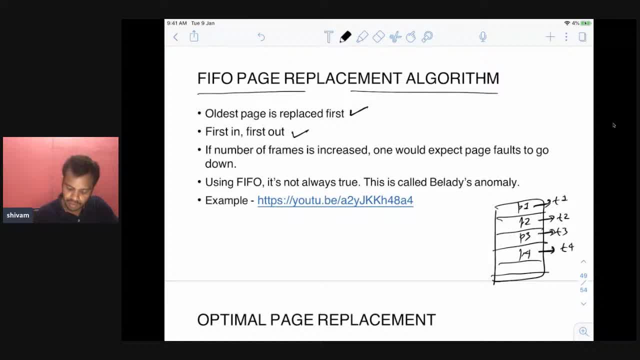 was bought after P2 and at last P4 was bought. Now, if you have to kick out one of this, you will kick out the T1 and the P1 page, because that came first. Now, in this case, what happened is the number of frames increases. one would normally expect that the page faults should. 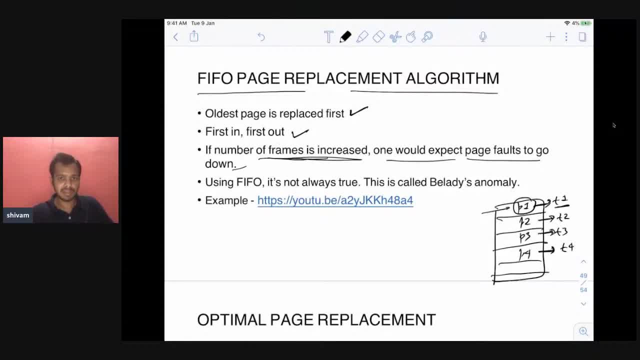 go down. right, If you increase the number of frames, right, that normally will think that right page fault should decrease, right. But in FIFO what happens in some cases does not. it's not always true in the FIFO case, FIFO page replacement algorithm And this: 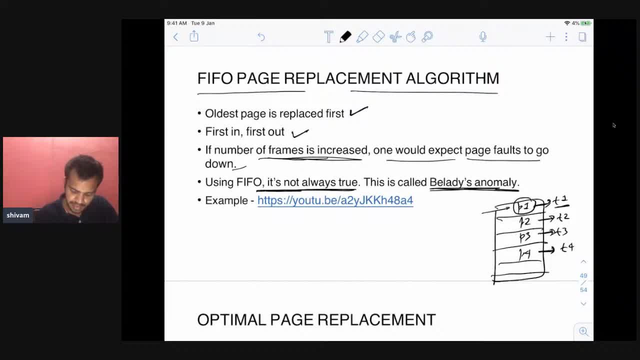 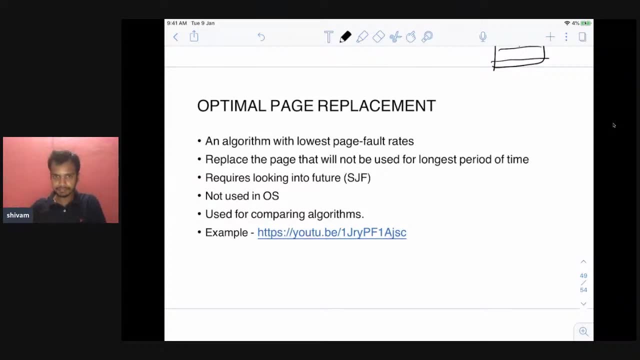 is called the Berardi's anomaly. This is very famous anomaly and you can read about this. I made a video also on this there. The example is here for FIFO, page replacement algorithm. You can see this. Okay, then after FIFO, you have optimization error. 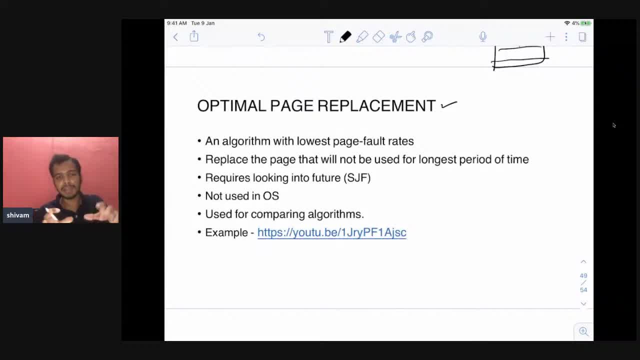 page replacement, right. so in this. so the optimal page replacement algorithm is the best algorithm actually, which will give you the minimum number of page fault rates, right, but i will tell you it's not ideal one. i mean, you cannot implement it, basically. so it will repeat: the algorithm is: 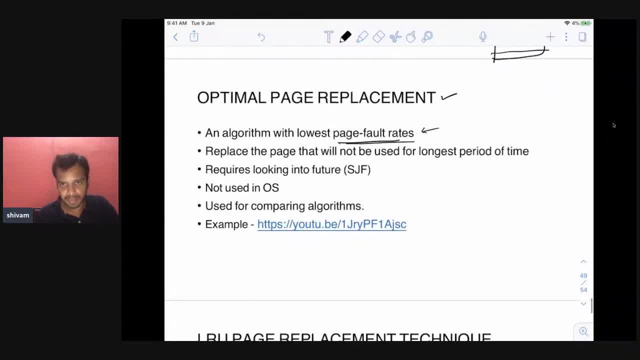 so, in this fifa, what was the algorithm? we replaced the oldest page, which was there, right? this algorithm is replace the page that will not be used for the longest period of time. so, basically, you have to look into the future, right, you have to look into the future. 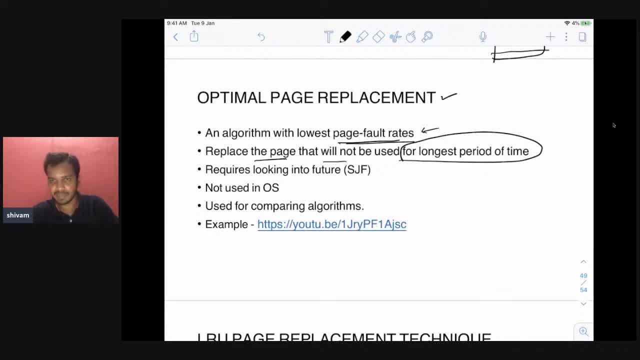 and see which page will not be used for the longest period of time in the future, and you need to. that will be the victim frame that you can kick out, basically, while doing page replacement. see, this is quite similar. see, this is looking into the future. but how will you look in the future, right? this system cannot look into the future, right, with instruction. 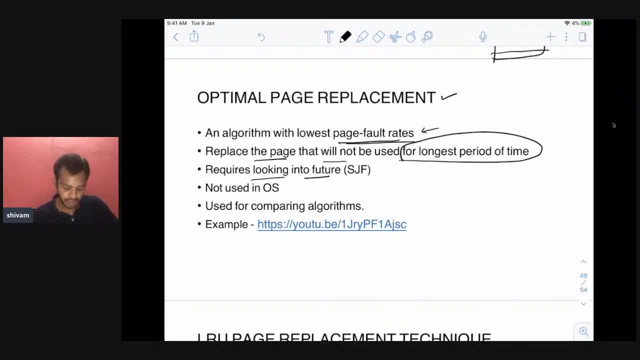 are going to execute. executed next right. you cannot look into that. it's kind of similar to sjf right, if you remember sjf right. sjf also looks into the future and the future time right and both are not. you cannot implement both. you cannot implement sjf also. 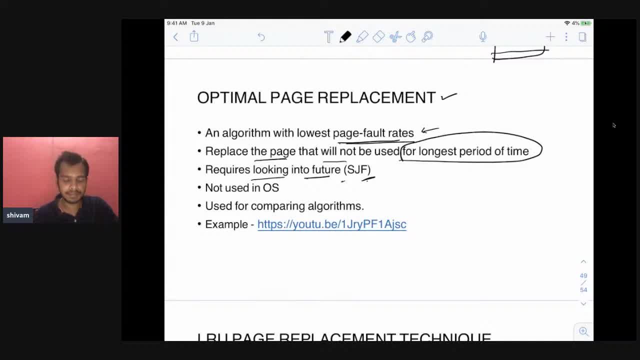 you cannot implement optimal page also and you will ask that, and why optimal page is there? replacement algorithm is there. it's only for comparing different algorithms. so this is the idea algorithm. this is the ideal algorithm with the lowest page fault rate. now you can compare other algorithm with this one. which one comes closest to this one will be the winner, kind of. 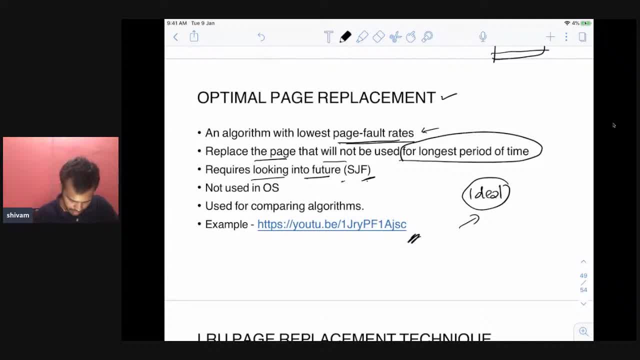 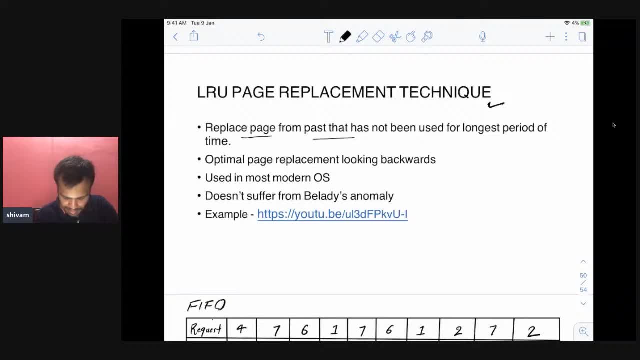 you can see the example i have given here, and the last one is lru page replacement technique. so replacement, uh replace page from the past that has seen the optimal page replacement algorithm looks into the future. the lru page replacement algorithm looks into the past. the concept is quite similar here. 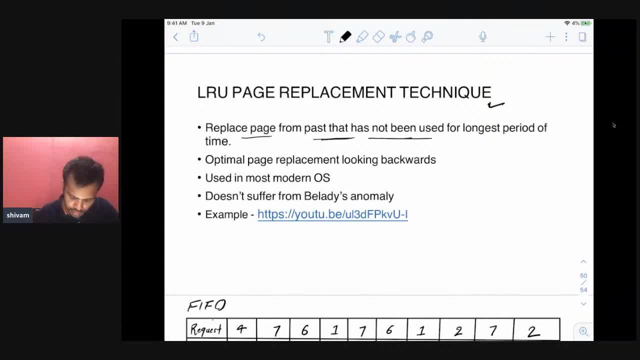 so replace page from the past that has not been used for the longest period of time. so go to the past always you can go right. future you cannot go, but past you can always go. so look at the past page and which pages has been accessed and then kick out that page which has been not been. 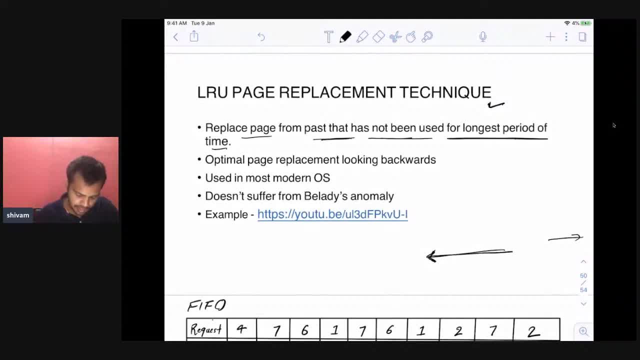 used for longest period of time. i will leave some examples here. this is optimal page replacement. this is all actually used in the modern opt-in system for page replacement algorithm. this is this one is one is the used and like both optimal and lru, they does not suffer from the abilities. 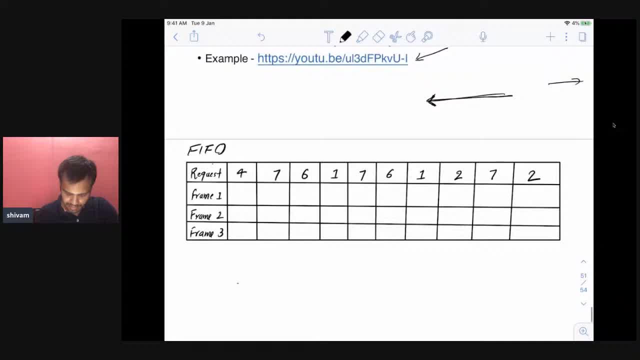 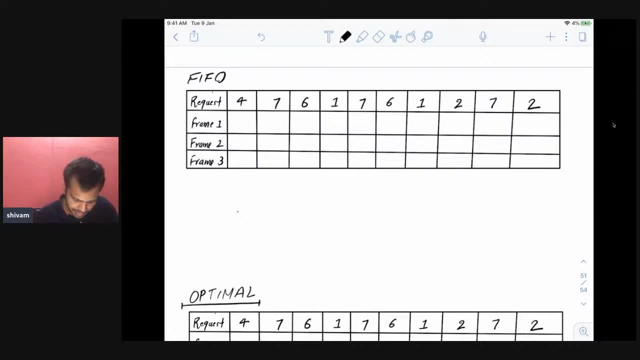 an example will be here. okay, let me, uh, show you like five people are. let me show you examples also here. it's quite simple. see here in fifa, what you do see initially see this: this is your. you have three frames in the main memory and this is the page number that you are going to access, right? 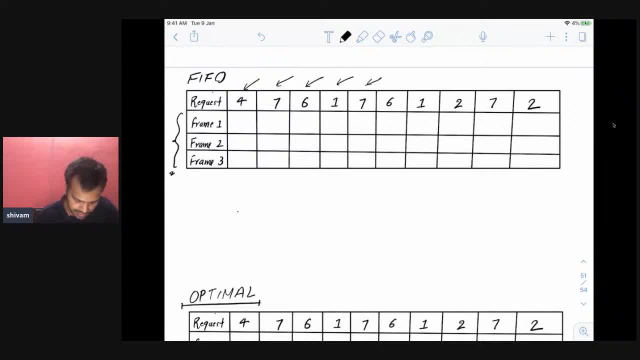 four, seven, six, one four right. this is the page number. so initially, if you see, the page number four is not there in the any frame, right? so you put it here and of course there will be. this is called page fault. page fault is here right, because that page need to be bring from or from the disk. 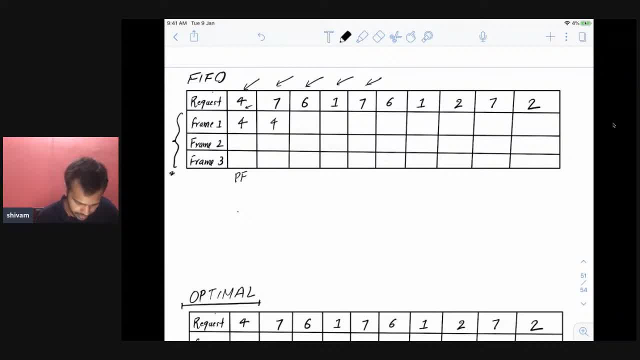 to here. right this here now. you have four here already now seven. is there now again seven also? you bought it here. you have page fault here again. then you bring four, seven, six and see for six also one access. there was one empty frame, right, so you allocated it here, right. but this is also a page. 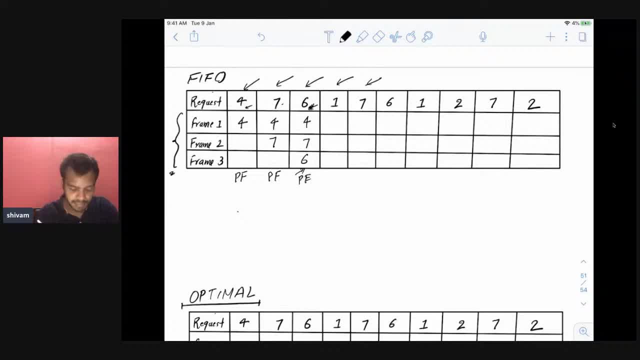 fault. right, because you are bringing the page number six from disk to the this frame, number three. now, when one comes right, is one there in the main memory? no, now you need to replace one right now. which one you will replace from these three? which one came first among four, seven and six? 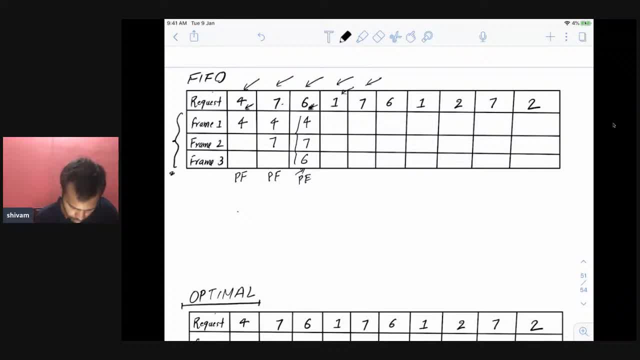 of course the four came first right, so you need to replace four with one. and again, there is a page fault here. again, see seven. if you see seven is already there right now, you do not need to do anything. there is no page fault here. no page fault in this case, because page number seven is already there in the main. 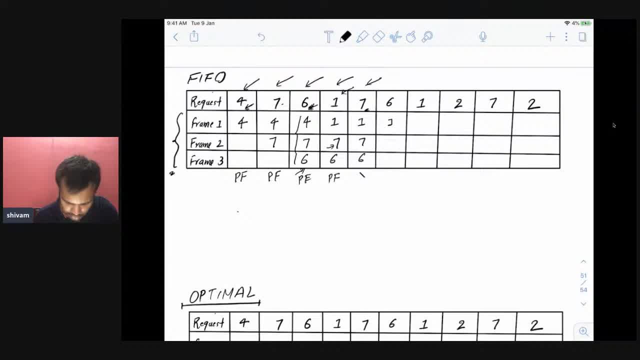 memory. when six is there again, six is also there, no page fault. uh, one also is there no page fault and one is already there, right? so there is no page fault. two, no, two is not there in the uh ram now you need to replace one among one, seven and six. so one came just now. i mean one came here, sorry. 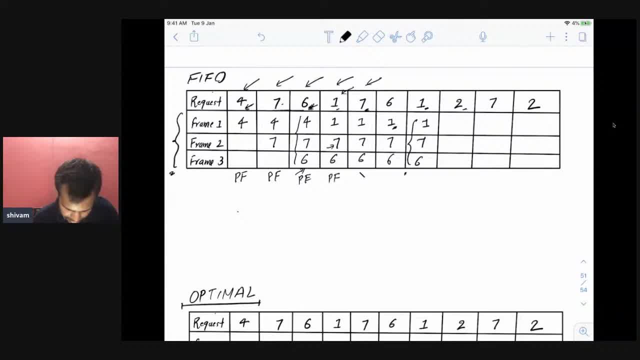 six. so seven among seven and six. if you see seven came the earliest right, so you will replace seven, right, one, two, six, right, because see among this, if you see among one, seven and six. so, uh, if you see one came here, right, uh, no one came here, seven came here. so sorry, seven came, one came here, okay. 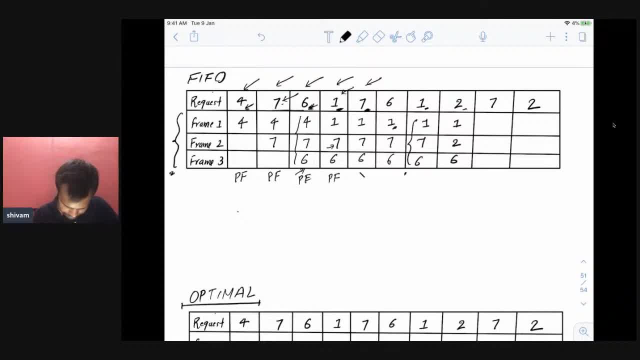 seven was accessed here, but it did not come. okay, i think six came out. yes, right, with all the off and on this thing, right, six. okay, let i have to clear the name. i got a bit confused, see, uh, if you see here now, you replace here one seven, six. is there right among one seven and six? 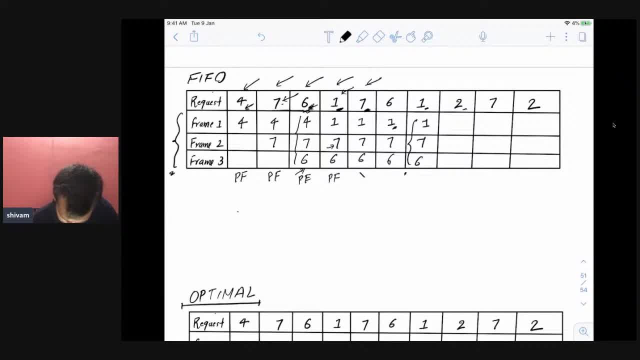 one has. okay, come here, right. and if you see the four, seven, seven is already there from here, right. and six came here, of course, seven. seven has come first. right, it will be one, two, six, now again seven is there, right? again, you need to replace one, or am i doing it wrong? 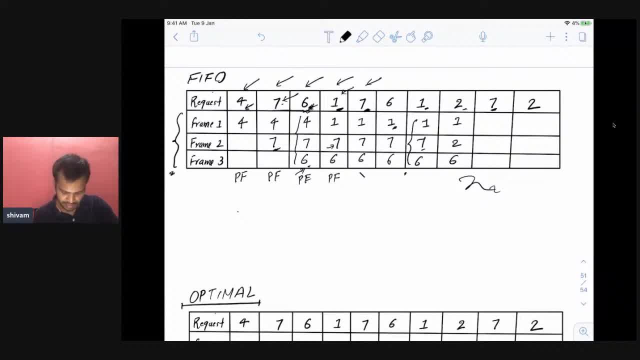 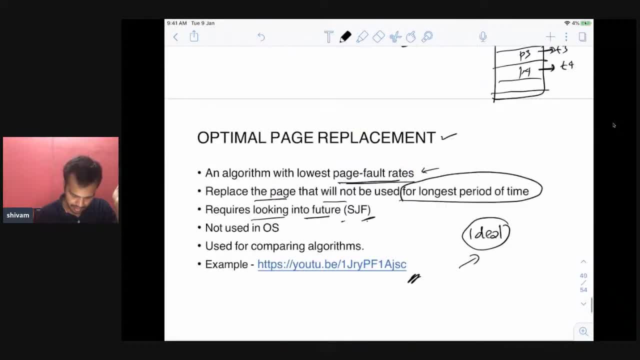 okay, what you can do is i- i think i have forgot this actually- maybe, uh, i i a bit confused about this. i'm in the fifo one, so what i will tell you is that, uh, what i will tell you is that, see, in this, the fifo replacement example is there in this video. i'll be 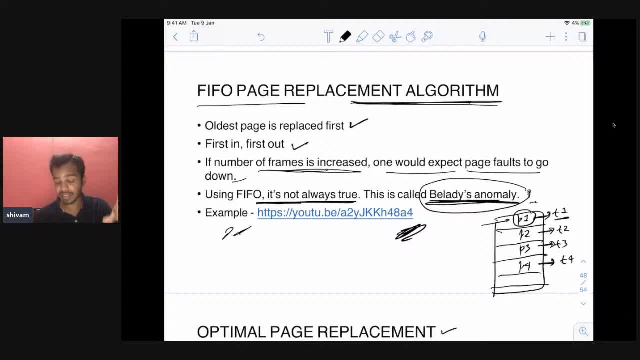 explaining clearly about all of these three algorithms. i do not remember actually. i i mean, i made this video a long time back, so i do not remember the algorithms actually now. so what you can do is you can watch this video for people. uh, why this video for optimal and this for lru? and? 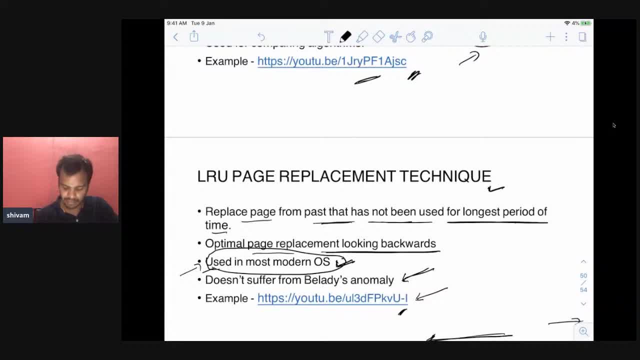 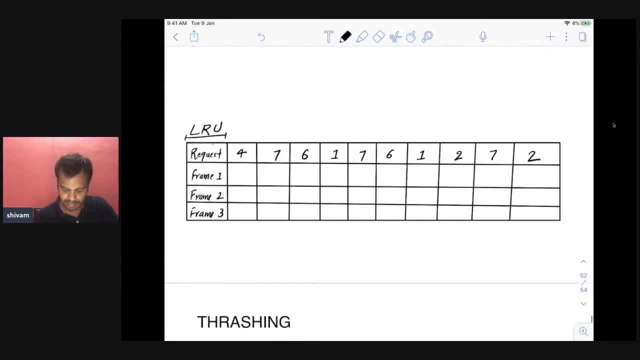 i've explained with very good way all these examples and you will get and get more clarity from there. so i'm not explaining the examples there and time is also like more than one and half hour, so let it be there and of course, i will share the ppt. people will be there in the description. 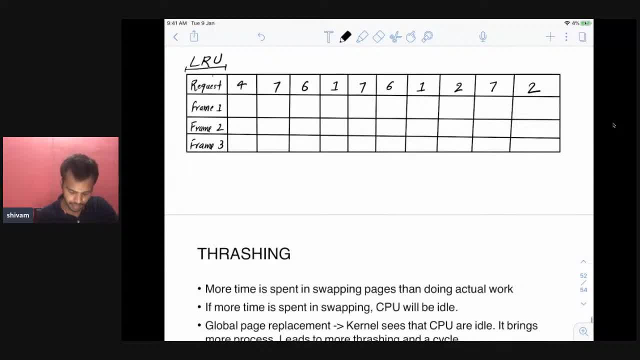 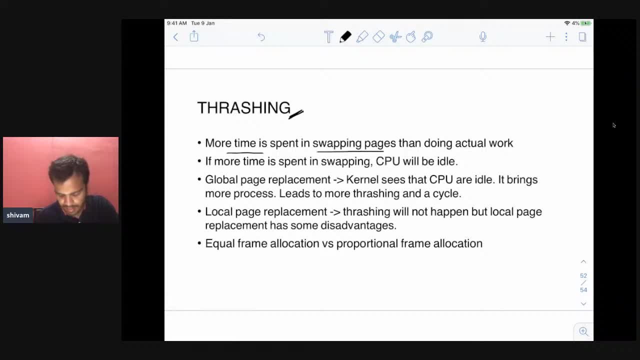 so you can take all those examples videos. so last part is thrashing. so what is thrashing? so thrashing is like if more time is spent in swapping pages than doing actual work, then this is called thrashing. so thrashing means that you are in. i mean, cpu is more busy with swapping in and out of the pages. 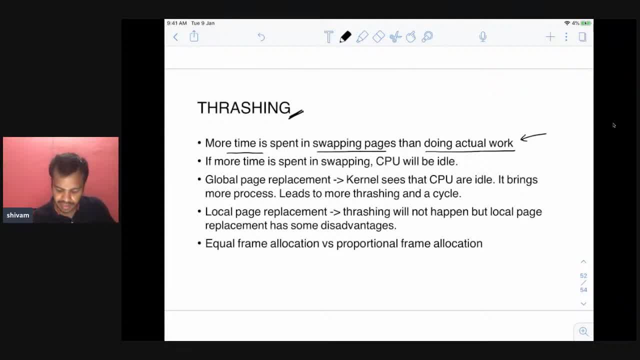 right in that, in that it is more busy than doing actually some productive work for cpu. what is the productive work? running some code, right, it is see what, when the swapping is happening, this is io what will happen? the cpu will remain idle right, because io is not controlled by cpu. so you will. 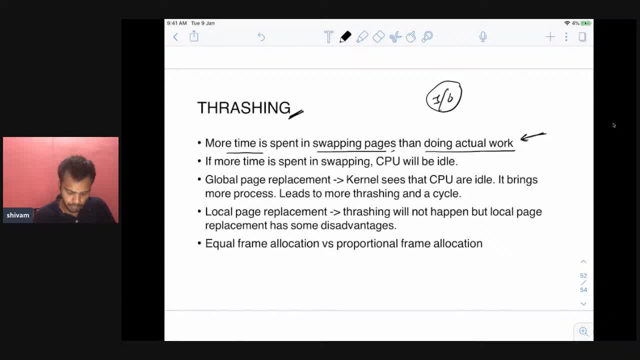 remain idle. right, that's what you have crashing. so if more time is spent in swapping, cpu will be idle. right now, see, there are two types of page replacement, that is, global page replacement and local page replacement. so in global page replacement you can replace the page with any. 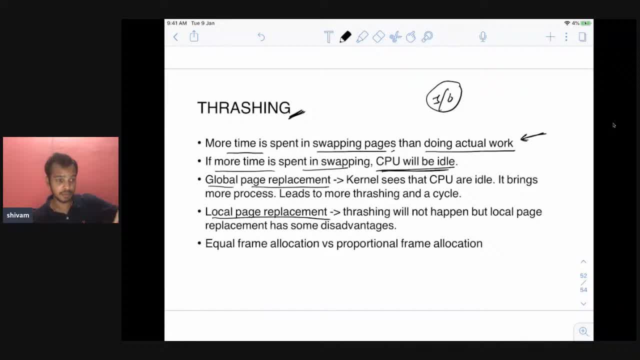 of the process. right, you do not need to replace the page from your own list of uh pages. you will replace, for you can take the pages from any other, like any other process, that is global. the kernel sees that the cpu are idle, so of course then more swapping is happening. 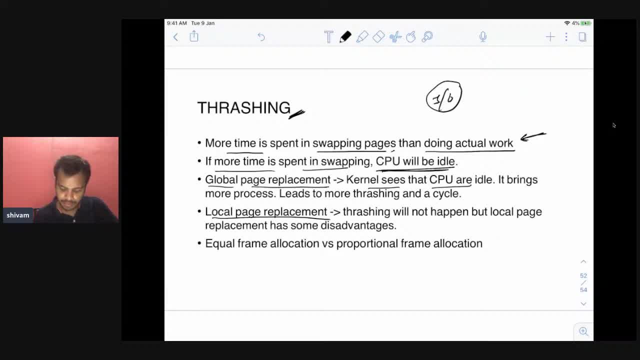 the kernel will see that the cpu is idle right now. what if? what is? it will bring more process right now. this will lead to like: see if cpu is idle currently, bring down more process. this more process will again cause more swapping. this cycle will keep on continuing like this thrashing will. 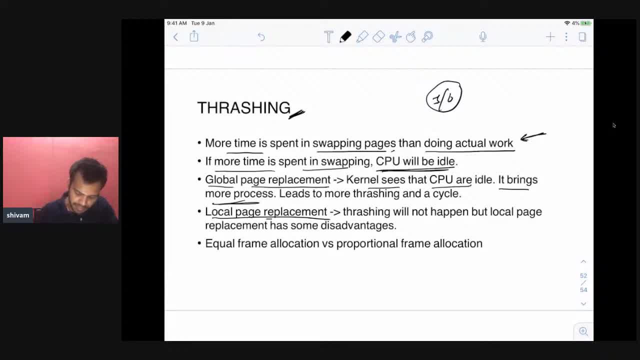 keep on continuing in local page replacement. volume will happen, thrashing will not happen, but local page replacement has some disadvantage. the disadvantage is that in local page replacement i you are allocated only three frames. let's say now, this size cannot change, right, if you do not use. 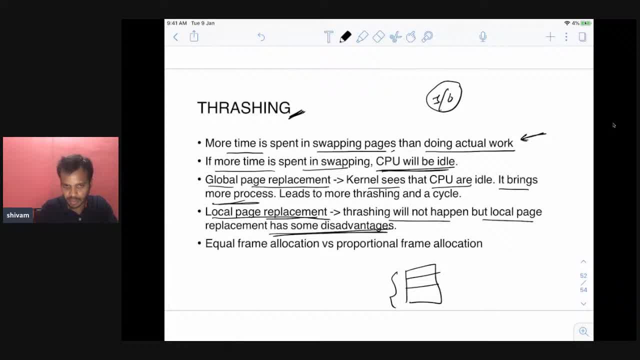 the global page, right. you cannot take the frames from another another process, right? so you are limited only with three frames. always that can be limitation. and there are two methods for allocation of frames. one is equal frame allocation and proportional frame allocation. so equal frame allocation is what let's say? if you have m frames and n pages, you give m by n frames to all of this. 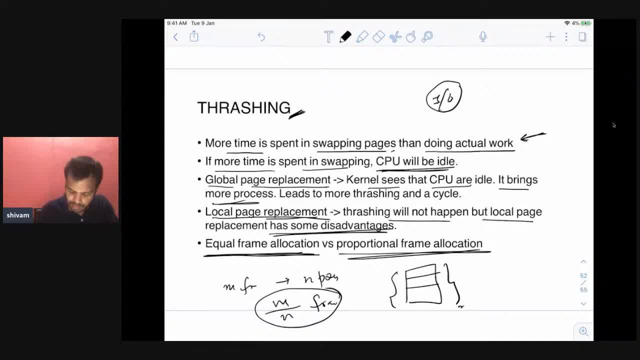 right, but this is always not good right, because one process will be of size, one kb. one is of, let's say, 10 kb. you do not want to give equal pages to both. in this case, you can use the proportional frame allocation, which is better. okay, i think i finally completed this, so the final uh session. 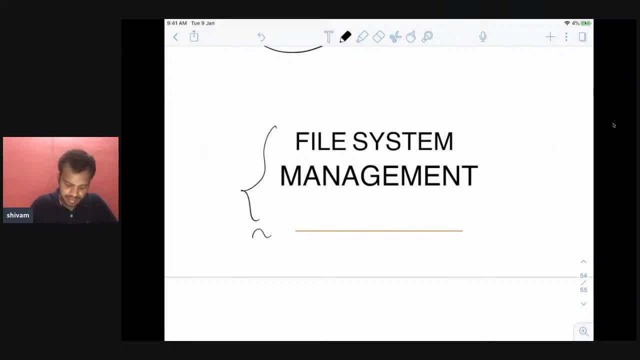 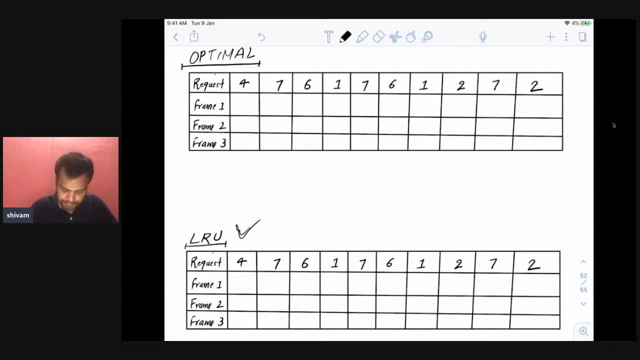 will be on five, six term management. that will be the next session next saturday. saturday or sunday, i will tell on that and also do watch this. i have not done this lre optimal here. i can forward this and it will take more time also if i do it here, so you do. 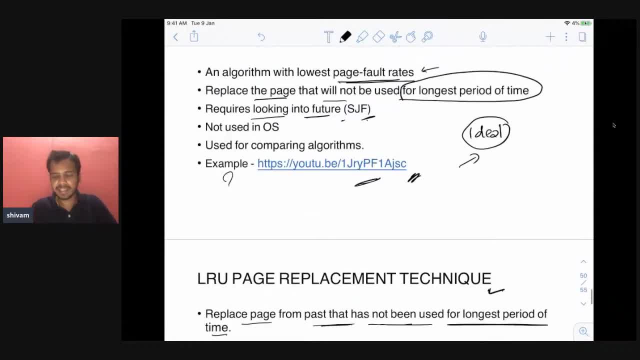 watch this video. examples here i have given here. people will be there in the description, so let me see if there are some questions. okay, what is segmentation fault? so segmentation fault, i will say, is see, segmentation fault means, uh, if your, if your process is trying to access the memory of 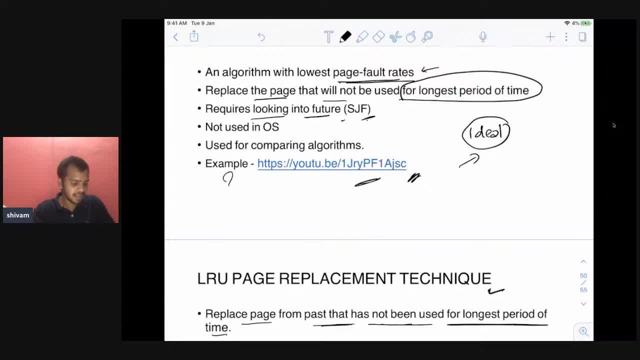 some other process it is trying to access the memory of some other process it is trying to process, then kernel will basically raise the segmentation fault. you will get a error like segmentation fault page. what is page table size? page table size is the number of pages. no, no, page table size is not number of pages, see page table size. i told you is the size, see this. 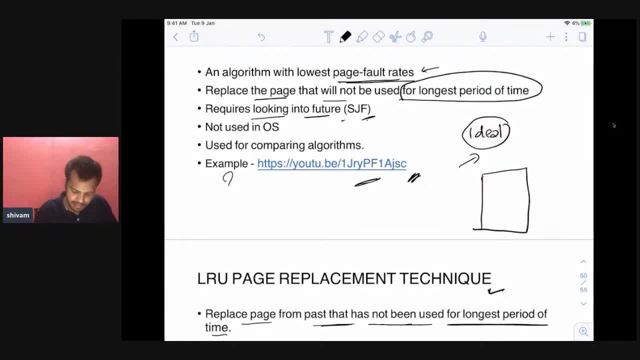 page table will take some memory right to be stored. right, that is page table size. now let's say the number of pages you have is zero, one, two, three, but the number of pages you have is four, right. but if you are storing some frame number here- right frame number one, frame number two- 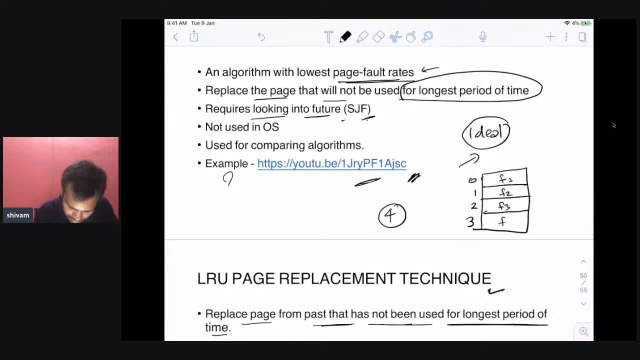 frame number three, frame number four. now this frame number itself will take some memory right, some bits it will take right to store. right now you have to multiply four into size of what what this frame is taking. let's say each frame is taking. let's say example i'm getting 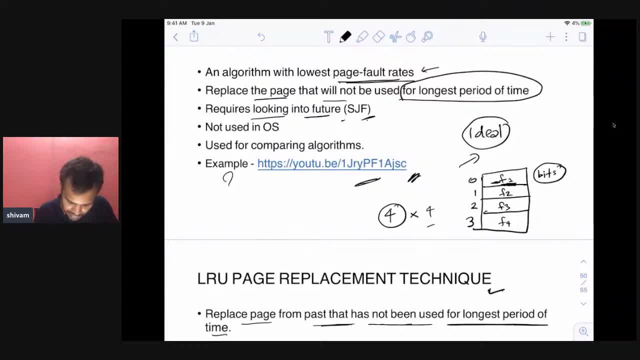 four bytes, let's say so total. total size of your page table will be 16 bytes, understand? this is very important. do not get confused. i mean between page table size and, sorry, page table size and not the number of pages. i think, harsha, if you are there, if you have understood this concept, i mean. 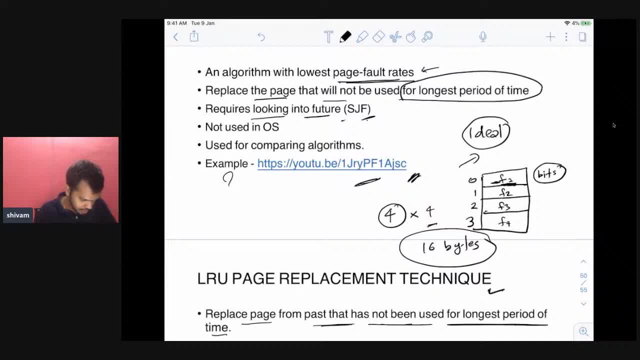 if your doubt is clear and also there should be a correction, i can logical address. so in pcb, not in program counter, right, yeah, yeah, see logical address. see, logical address means logical address is a sequence of address. right in program counter, only the instruction, only the address, that is. 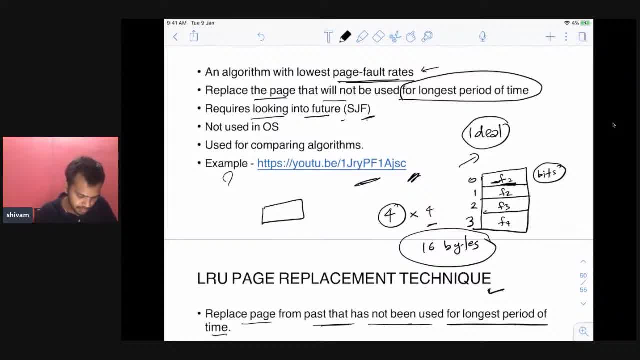 going to be executed next is going to be stored. let's say the value will be 1000, a single value. you will have also logical address, like stack. stack will go from the logical starting address of the stack can be, let's say, 200. it can go to, let's say 500. then for heap, the starting address. 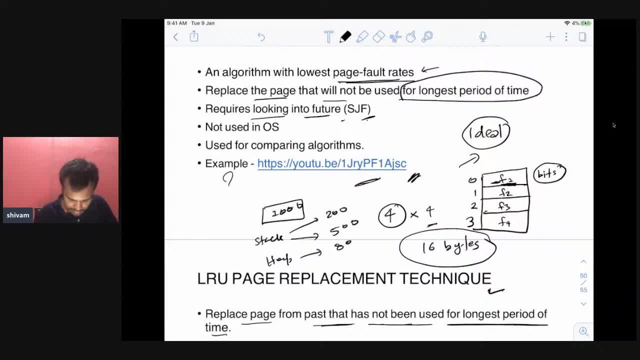 can be 800, it can go till thousand. right, let's say now this information also, you need to store in the pcb separately and that is stored in the memory management uh attribute actually separately, so that this is a program counter and this. both are different. so basically you are. 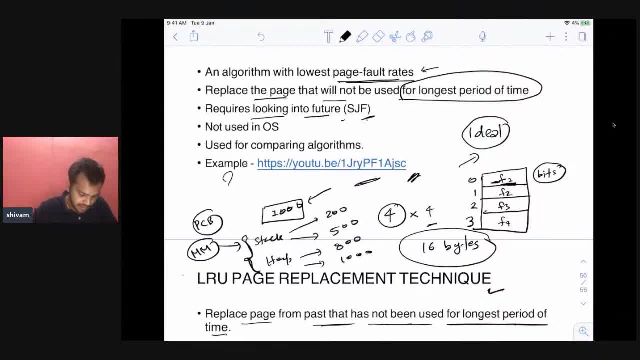 storing the whole logical address in the memory management attribute and in the program counter you are storing just the next address that needs to be executed. okay, i think these are all the questions. and yeah, how do you remember all these details? i always forget. yeah, i, i mean, i remember. 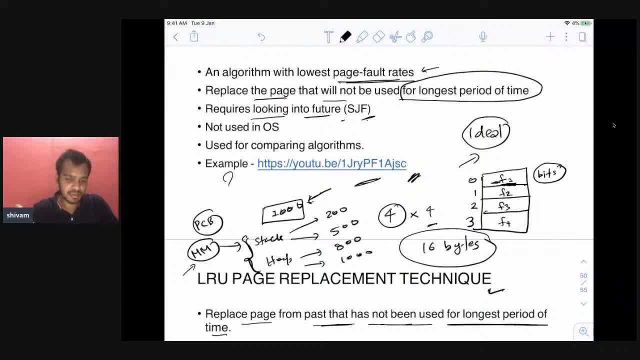 the concepts now very well, i mean something, something like i told you, like like fifa and all you need to like, go through like examples and you will understand more. so that's why i also followed that, if you see here, right, so some things i also forget. i mean, but yeah, both of the concepts i 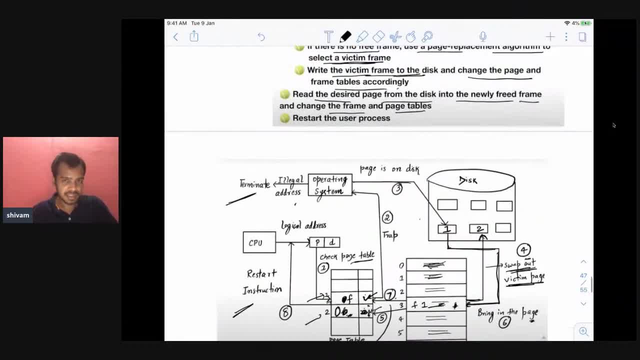 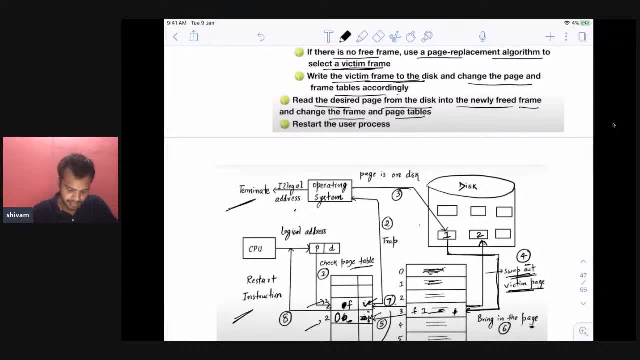 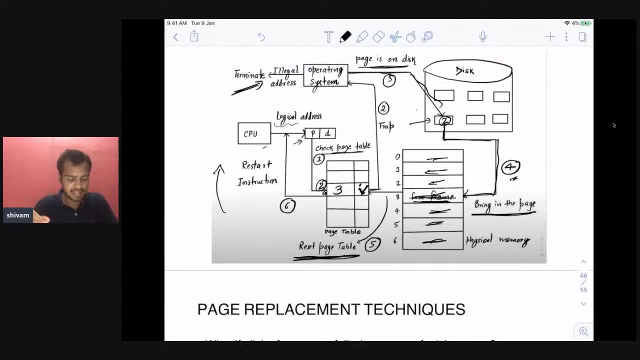 remember of paging and everything, how the paging. i mean, how this, i mean how logical address is converted into physical address. this all i still remember. i mean how that is calculated, and that's not tough right. if you understand diagram well, you'll understand that well also. so i think that's all for the session and in the last session that will be the uh. 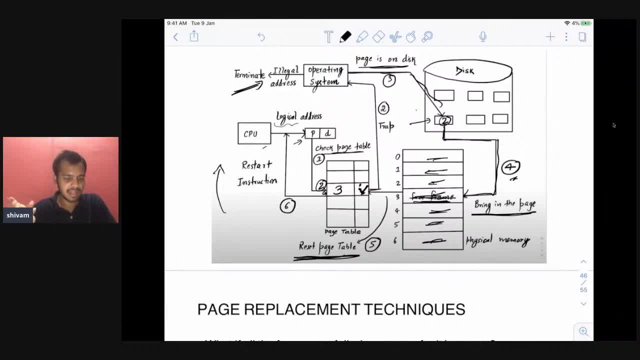 next week i will cover the file system management and i think this operating system will be over mostly, and after that maybe i can start some other series. i will see, i mean this series i can start. then i will start the number one. yeah, thank you for everyone, i mean who was here for like. 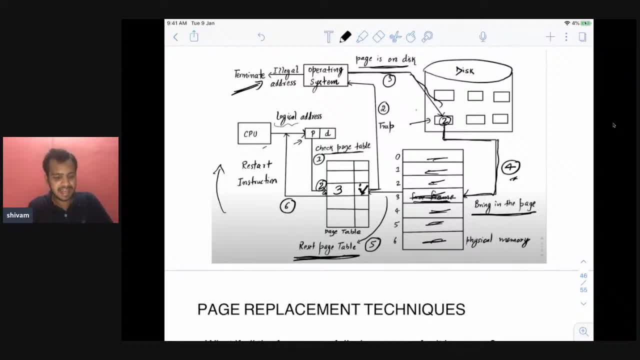 one hour 40 minutes- almost right with me here, and i am sure that you would have learned something from like whatever i covered here. you would have learned something new or maybe it would have helped you in devising the concept whatever, because memory management, i see, is very important. 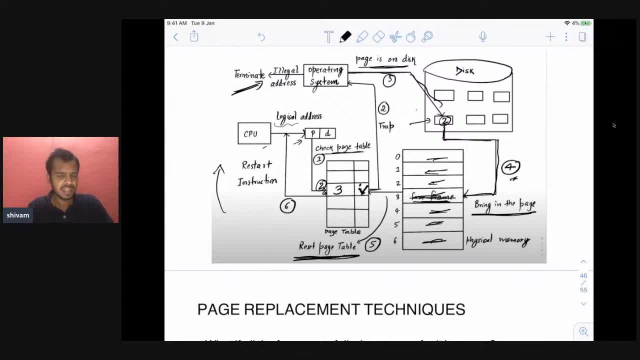 i mean in operating system process management and memory management. if you know both the two, i mean it's quite well. i mean you understand most of the operating system. i will say: if you know both, and i will also, maybe i will also start a series in which i will give you more real life.